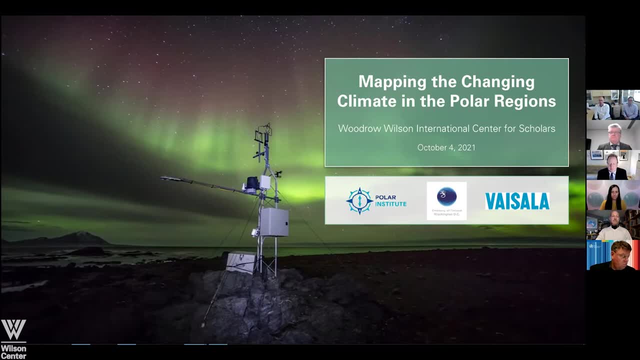 for their continued and fruitful partnership and friendship. I also thank our colleagues at the United Nations for this important program. We have an outstanding panel of experts today with us to share their expertise and their insights. Each speaker will provide opening remarks and engage in follow-up questions. 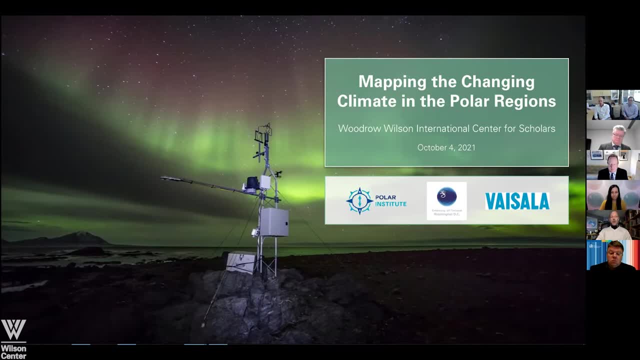 I encourage my colleagues watching to please participate in this program by emailing your questions to polar at Wilson Center, dot org. polar at Wilson Center, dot org. Let's make this a participatory program. As our website noted, as climate change accelerates and the Arctic becomes more accessible and more important, perhaps now more than ever, there is a growing 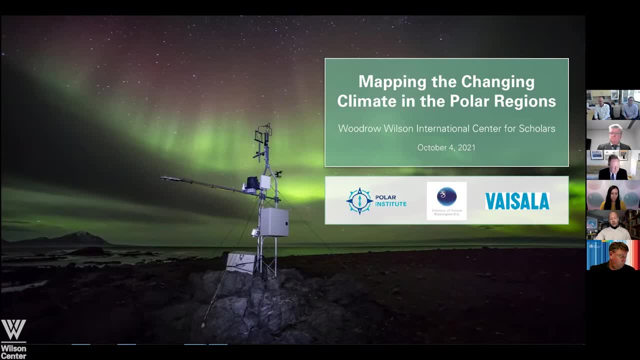 realization that the Antarctic region, too, is increasing, is increasing in global importance, so there is a need, we believe, for more discussions about these two unique but in many ways interrelated and interconnected regions. arctic countries share a commitment to protecting the environment of the arctic, as well as the antarctic region, where many 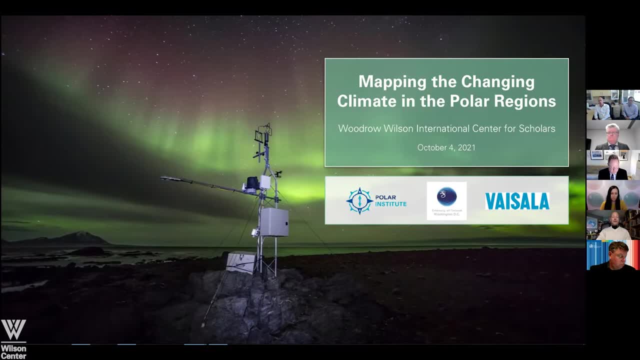 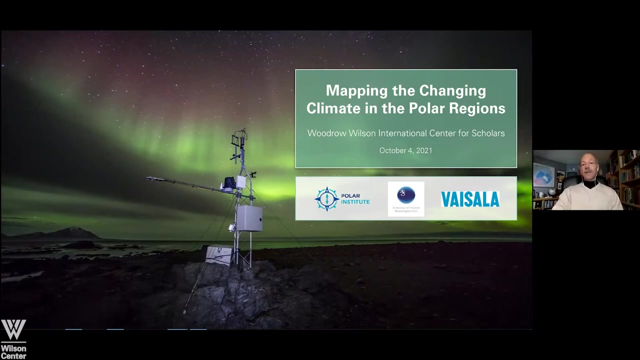 environmental, geopolitical, natural resource and scientific activities are becoming increasingly more important. finland and the united states, as well as the united nations, share a commitment to increasing arctic and polar scientific cooperation, as well as responsibility to create awareness about the pace and impacts of climate change in the regions we are so pleased. 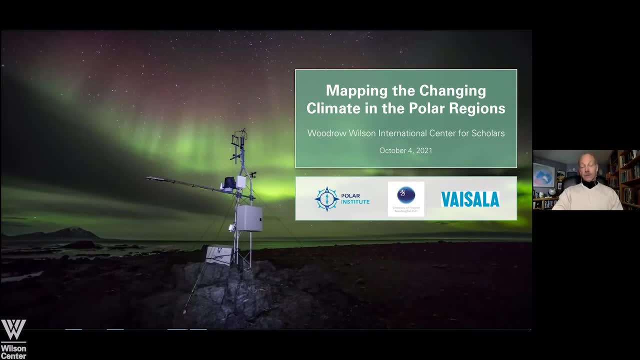 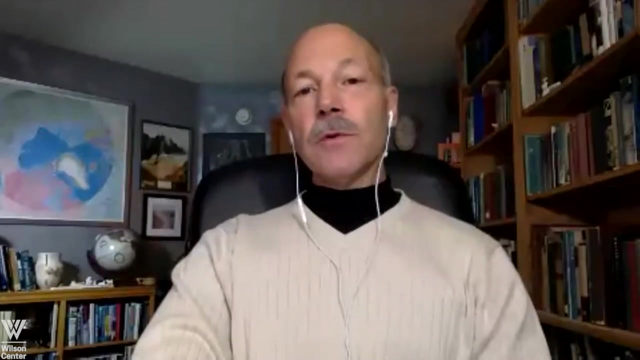 to join the embassy of finland and the world meteorological organization for discussion, exploring the new ways science and technology can assist the un, can assist finland and the united states to address the challenges presented in both of these most consequential regions is in this context that i now present miss heli hoopia, counselor section for sustainable growth and commerce. 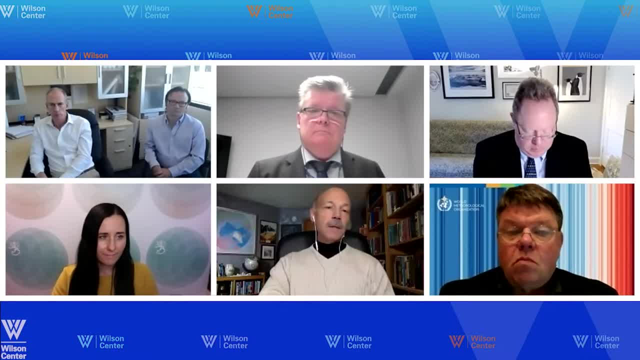 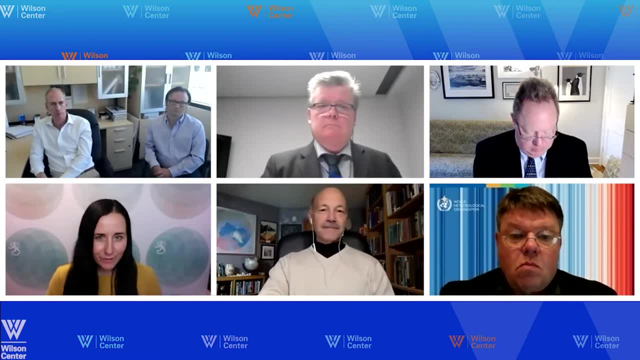 embassy of finland and washington dc for her opening comments. heli. the floor is yours. thank you very much, mike. i'm happy to cover what i believe is the most interesting portfolio at the embassy of finland to the united states in washington dc: policies related to the arctic climate and green economies. 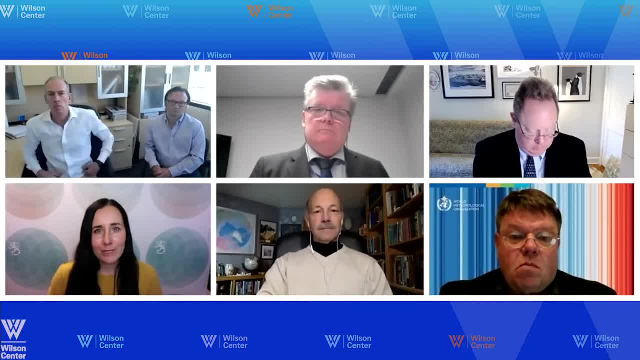 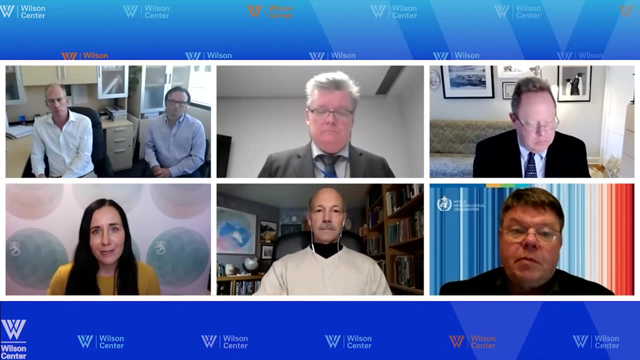 on behalf of the embassy, i would like to welcome everyone to today's event and thank dr srega and the wilson center polo institute for your cooperation, not just today, but the cooperation, close cooperation- we've shared over the years and will continue to have for many years to come. i know mike, ambassador bolton. 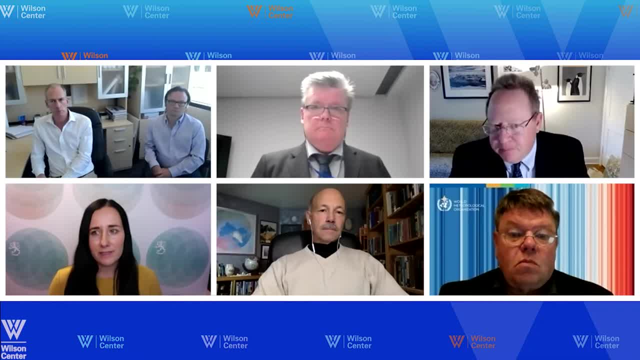 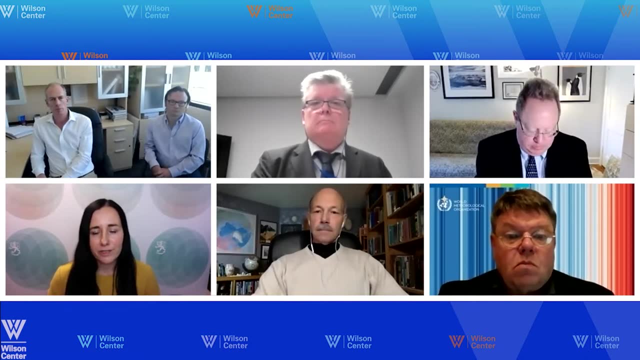 evan bloom, colleagues, your institute does such an important job in successfully bringing visibility to the significance of the arctic and polar regions in global policy, whether in climate science and policy, sustainable economic developments or or geopolitics. finland and our embassy, shares that priority. the artist arctic is never absent in our discussions with 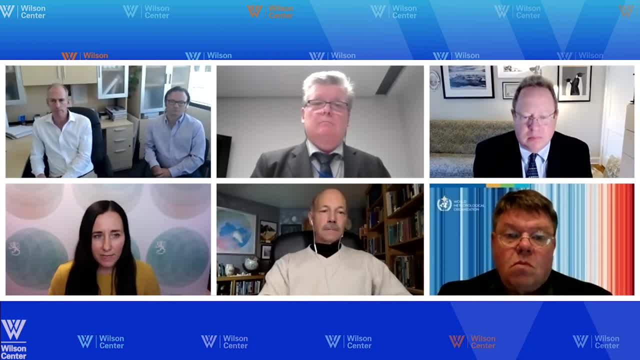 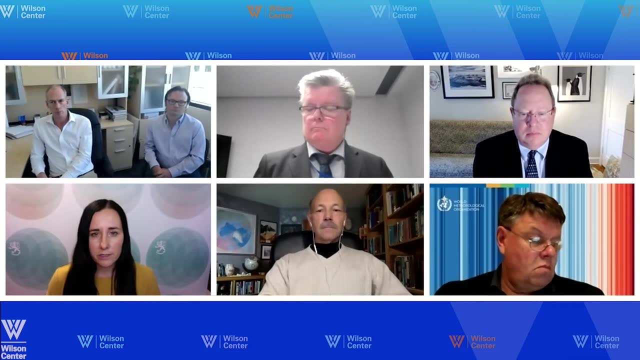 interlocutors here in the united states. finland and the us are both arctic countries and there are only eight, as you mentioned, mike. the region's importance globally is rising. finland has just set new arctic priorities, very much focused on the pillars of climate action. 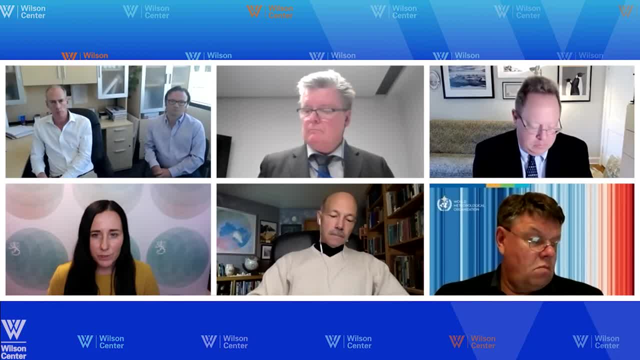 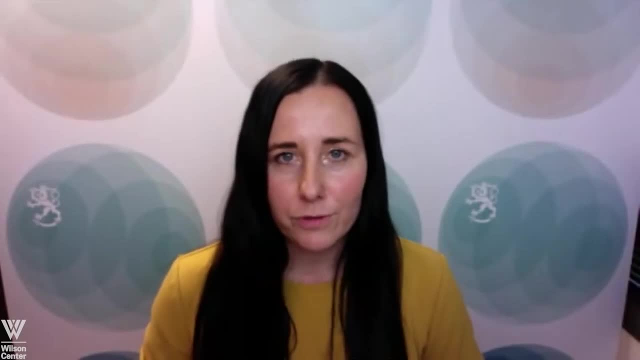 the well-being of arctic inhabitants and sustainable economic development of the region. we look forward to working together on these teams with our partners here in the us. we've just returned from an excellent visit to alaska, where a delegation from the finnish and northern european countries is present. here and in this session we will talk about the history and 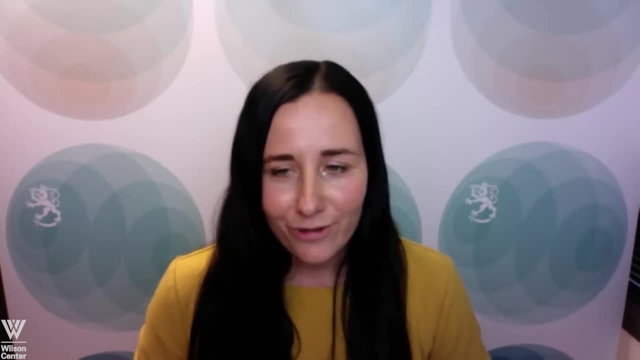 Norwegian embassies traveled together. Mike, your participation in the program and insights on the trip were priceless. also funny, as you always are, but priceless in the sense of invaluable insight connecting the dots from the US Arctic to us in the Nordics. 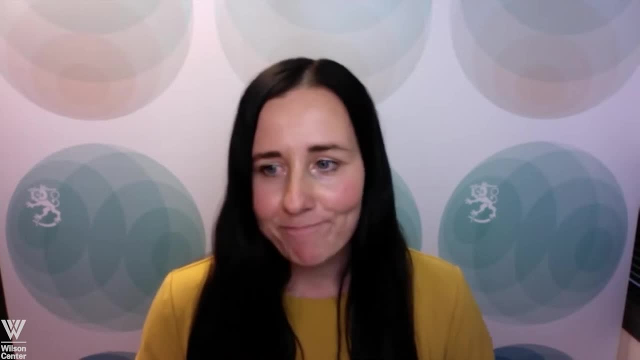 And finally, I would like to warmly thank the panelists. today We're proud and happy to have in the panel Finns and honorary Finns that are distinguished experts in their fields: Professor Petteri Taalas, Ambassador Petteri Vuorimäki and Mr TJ Matimore. 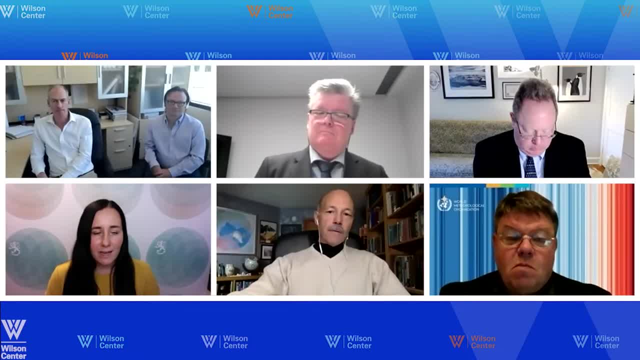 from a global Finnish forerunner company, Vaisala. I look forward to listening to your discussion and I hope we have many viewers joining today. Thank you, Mike, Thank you Heli, And it's always good to have a mix of good content. 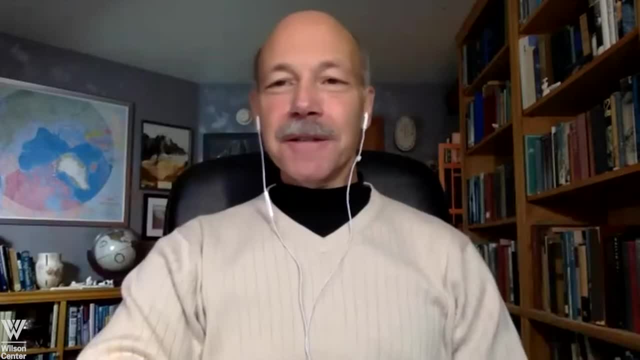 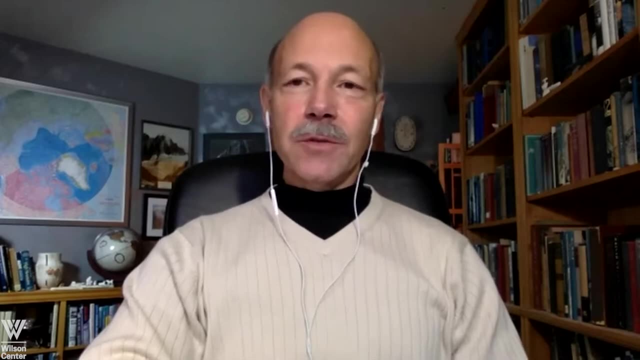 but a sense of humor as well, And I appreciate you And I appreciate you and our colleagues from Norway coming to the state of Alaska and finding so many connections between the US, Alaska, Norway and Finland, And it was priceless on both sides. 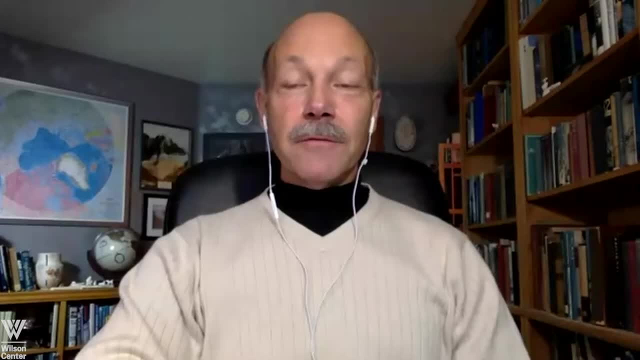 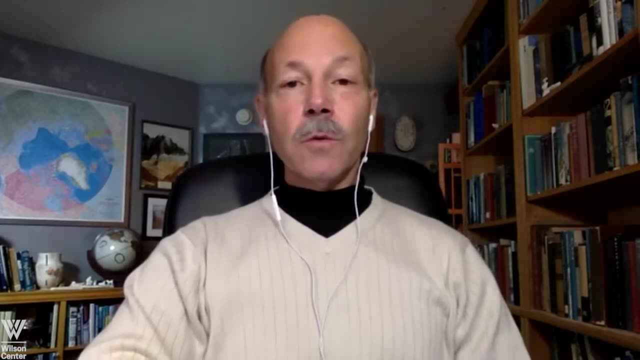 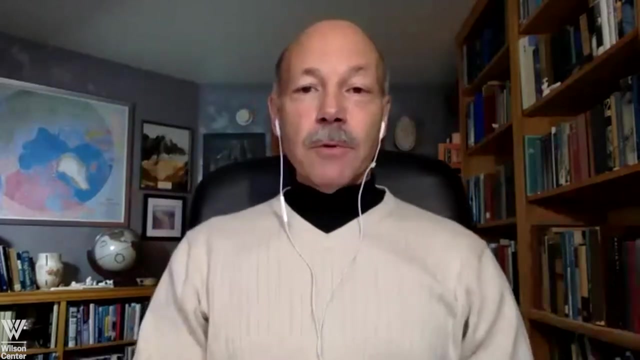 So thank you for that. As Heli noted, we have four distinguished colleagues with us today: Dr Petteri Taalas, the Secretary General World Meteorological Organization. Ambassador Petteri Vuorimäki, Finland's Ambassador for Arctic and Antarctic Affairs. 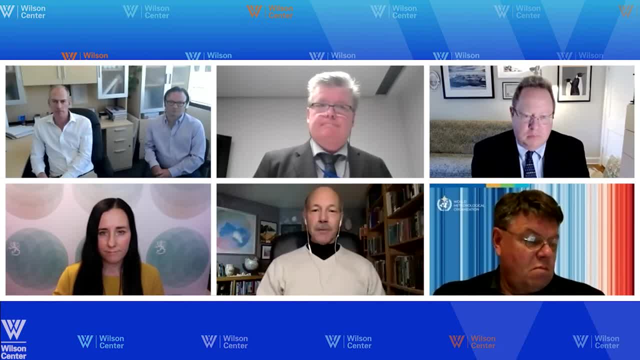 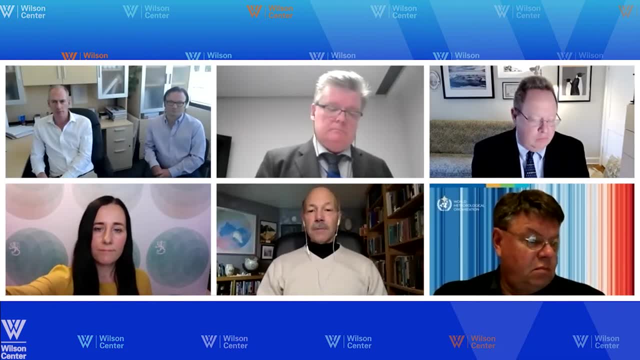 and Senior Arctic Official for the Arctic Council, Mr Timothy J Matimore, or TJ Matimore, President of VESELA, as Heli noted, And my friend and colleague, Mr Evan Bloom, Senior Fellow at the Polar Institute. 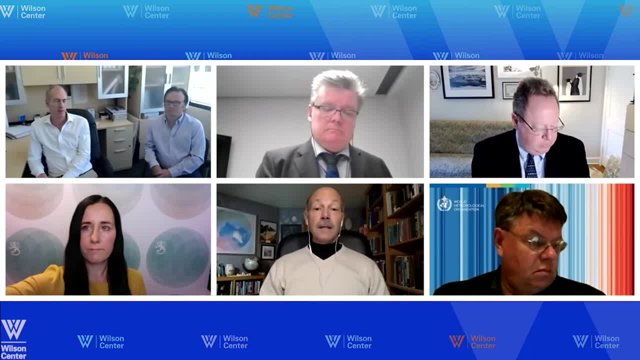 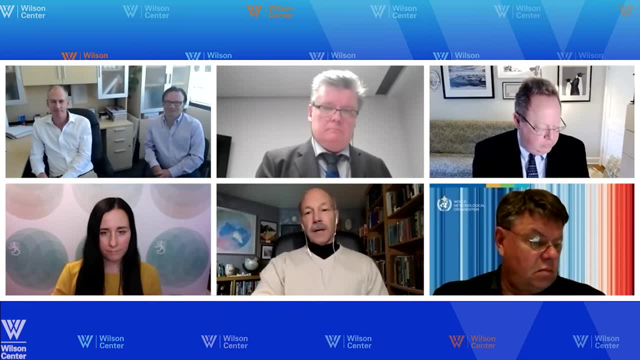 Many of you know that Evan served as the former acting Deputy Assistant Secretary for Oceans and Fisheries. He also served director for Ocean and Polar Affairs at the United States Department of Fish and Wildlife state, an outstanding panel, and we thank them very much for their time and their effort, mr secretary. 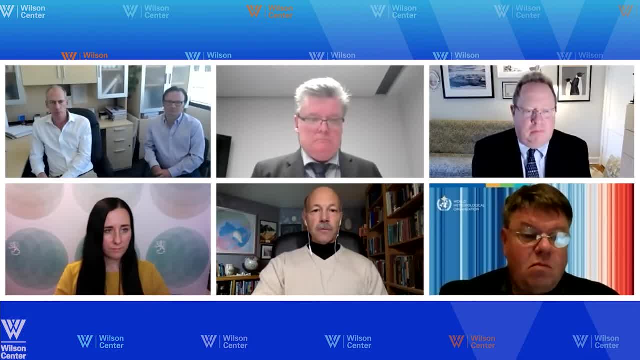 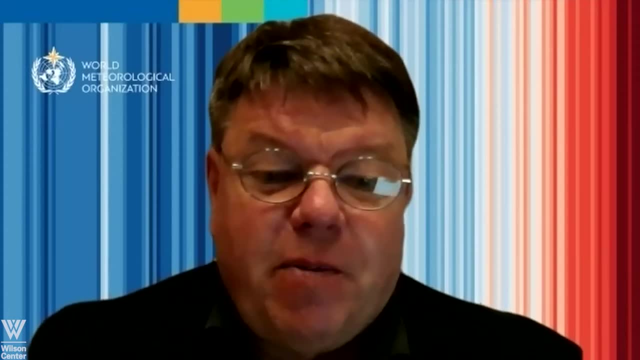 general. with that very brief introduction, allow me to turn this virtual floor over to you, thank you. thank you, mike, and greetings from rainy, rainy geneva. it's it's a late, already late evening here, but i'm happy to happy to join you from here and i would like to share you some, some slides. 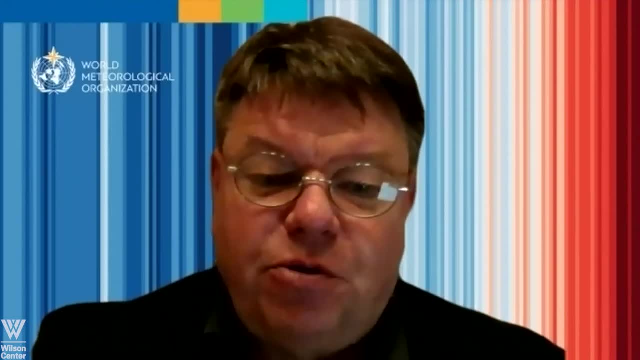 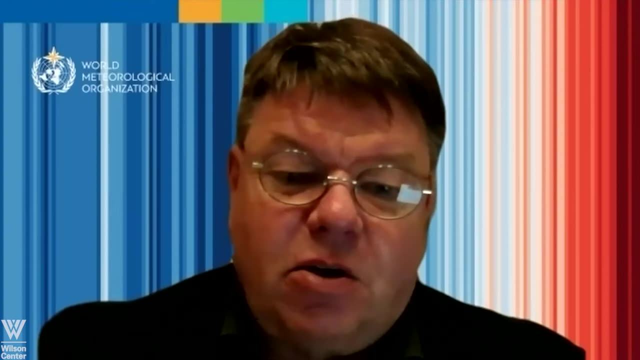 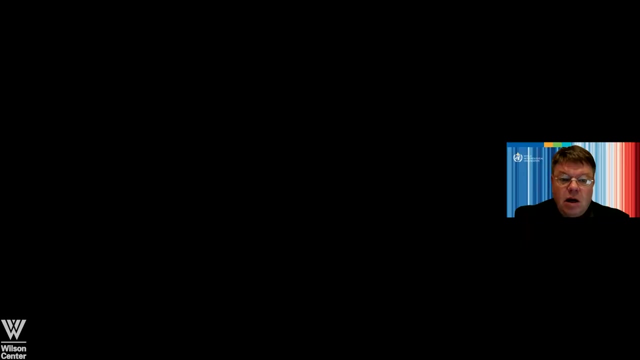 concerning the status of arctic and how the user of arctic looks like from the perspective of of a climate science organization like wmo that i have been leading for the past six years. i will share my my screen with you and i hope that you can. 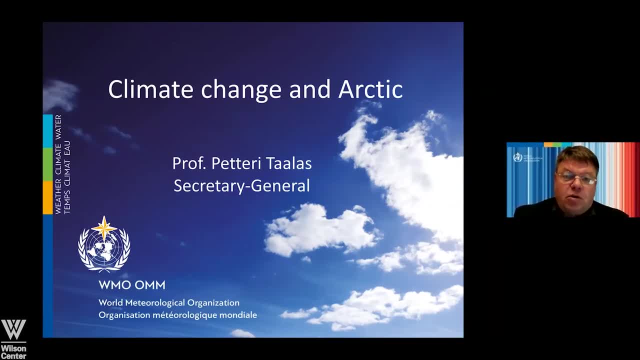 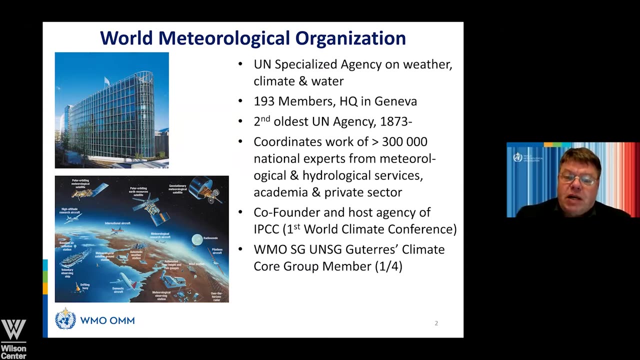 you can see it now. so, uh. so wmo is, uh is the united nations specialized agency on on on weather and and climate, and and we have practically all of the un members are also our our members and and most of our work is done by our our members. we are, we are coordinating the 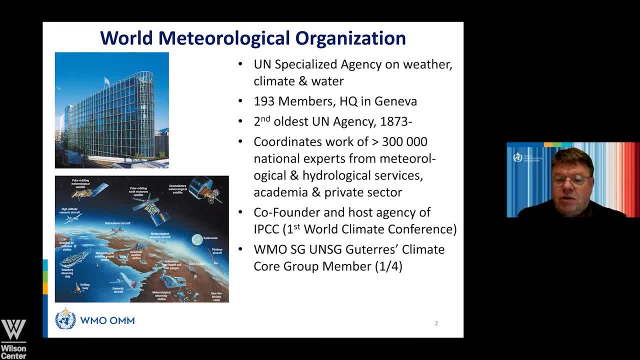 work of of meteorological, hydrological services, academia and also growingly private sector. and we are hosting ipcc, which is providing scientific reports on on climate and uh, and we are just in the process to publish the sixth assessment report and i'm personally also a member of uh secretary general guterres climate, the core group, and we are preparing this cop 26. 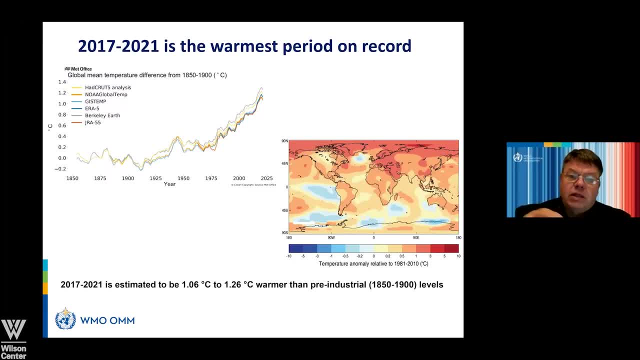 meeting at the moment. this is what we know about. about the temperatures, you can see that we have seen already uh from one one point one to one one point three degrees warming, depending on on which center is uh calculating this time series since 1850s, and you can see on the map here that during 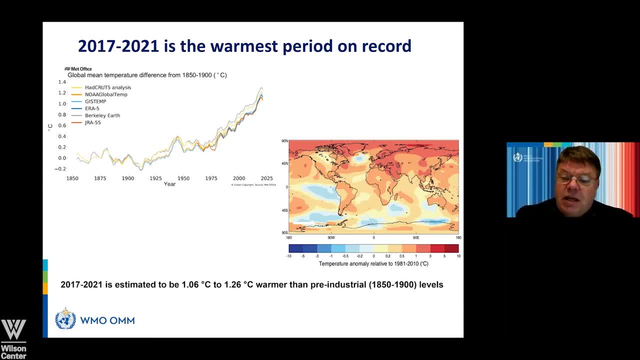 the past, past five years, we have seen uh anomalies, especially in the arctic, and there's one special feature in the arctic which is the cooling that seems to be happening south of greenland and iceland and that's most likely related to the slowing down of so-called the gulf stream. 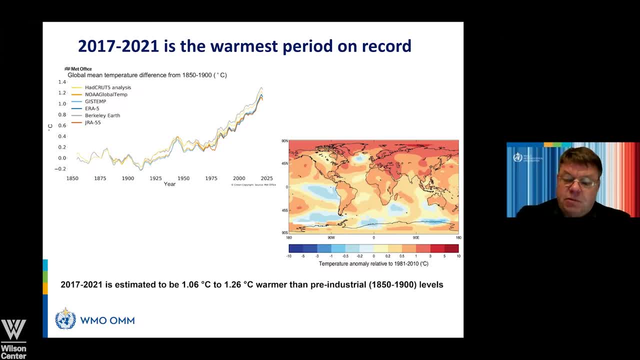 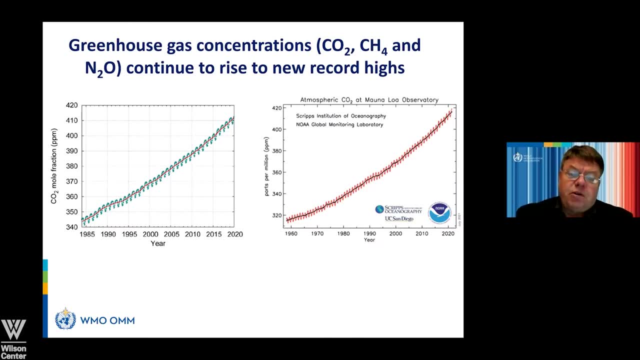 but arctic, of course. globally it's the. it's a special, special area on our planet and we have seen an increase of of the main greenhouse gases- carbon dioxide, methane and nitrous oxide- and and the same trend that has been observed at mauna loa has been also observed. 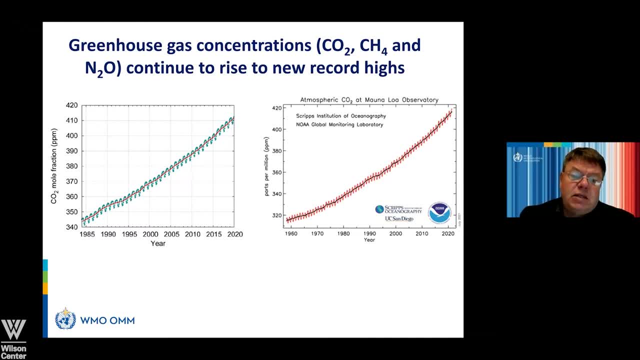 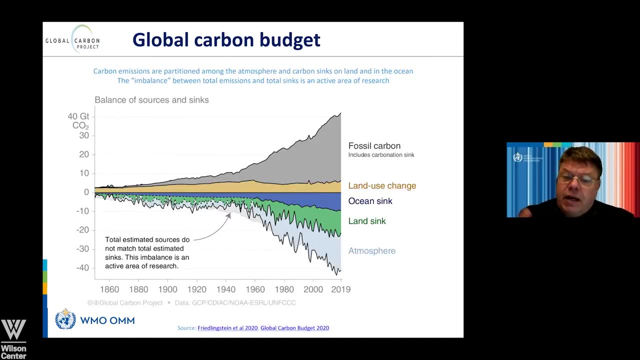 in the arctic, for example at the finnish palace station, the amplitude is a little bit higher, but overall average concentrations are the same and and the trend has been the same as as in in case of mauna loa. and we are dealing with the carbon budget and you can see that the fossil carbon is clearly 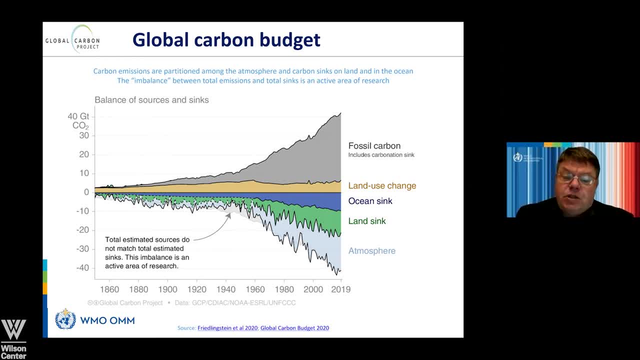 dominating this picture, and and land use is contributing about 14 percent of the of the challenge, and that's mainly uh. deforestation. the tropical, tropical areas, notions serve as a sink of carbon, and and so do forests, and the remaining part stays in the atmosphere, which is this light blue. 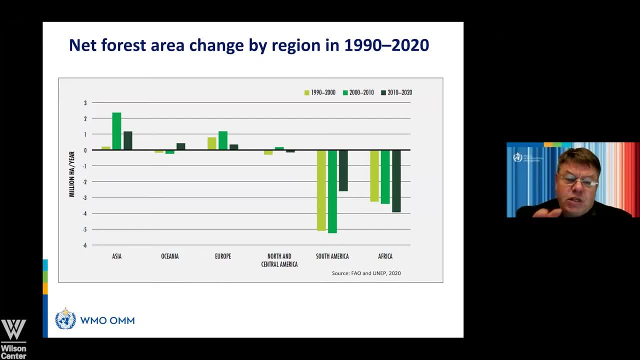 area here, and we have seen deforestation, especially in south america and africa, whereas in in most northern hemisphere areas we have seen either zero or or slight increase of the forest power, and and this climate change has been contributing to the more intense growth of forests and and that's why we have started seeing growing amount of biomass there. 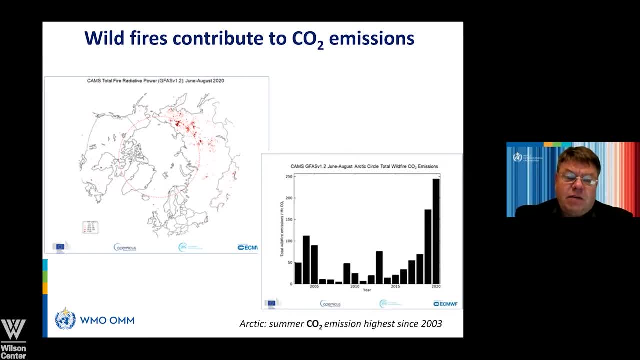 one forest. the forest related challenge in the arctic is that we have started seeing also heat waves and drought and- and that's why we have we have started seeing growing amount of carbon dioxide emissions coming from wildfires and and so far the record has been broken in 2020. a year ago. 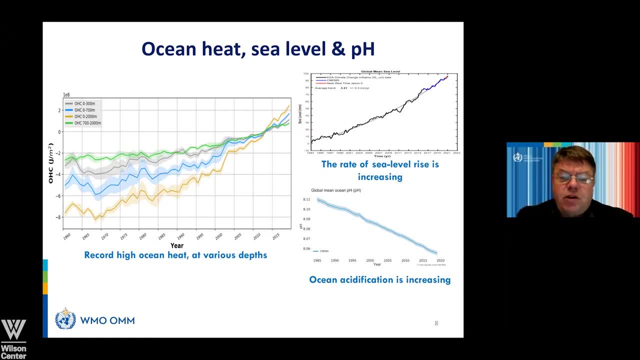 we have stored more than 90 percent of the extra excess heat to the oceans and- and this is partly contributing to the sea level rise- besides melting of the glaciers and once, oceans serve as a sink of carbon, we have also changed the chemical composition of the seawater, and there's an estimation that the 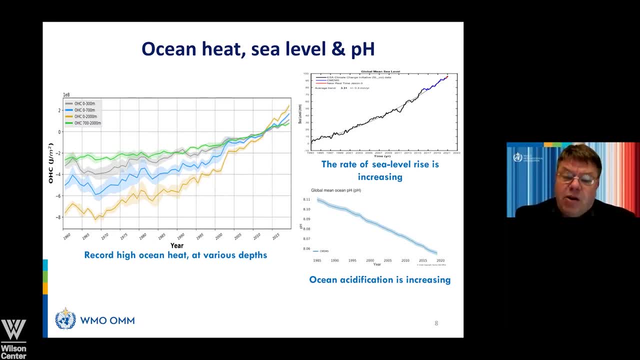 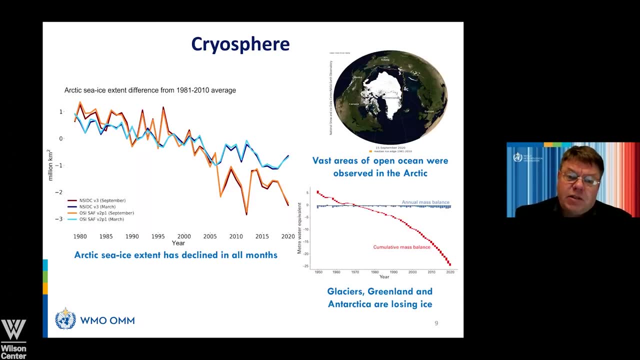 bsc is now lowest in 25 million years, and i'm sure that you have seen these, uh, these ice cover graphs demonstrating that both the spring and the autumn ice covers are shrinking and this year to year variability, And then we have seen also intensified loss. 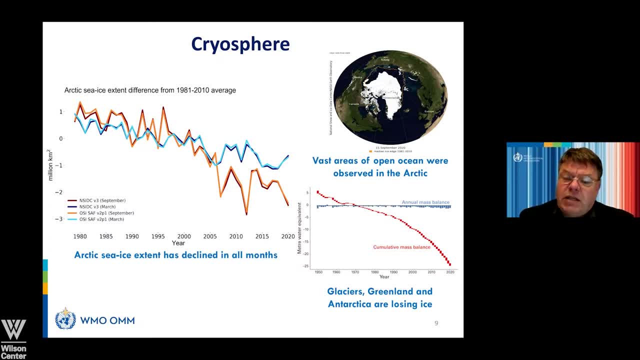 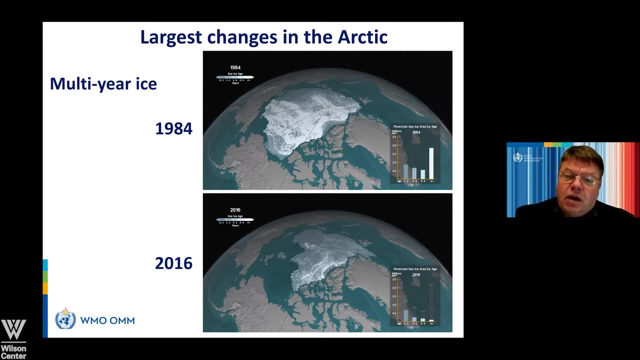 of ice mass in the glaciers, and especially Greenland has been losing record amount of its ice mass And I'm sure that you're also aware of this ice mass changes in the Arctic. We have practically lost multi-year ice from the Arctic and we have mostly one to two years old ice left nowadays. 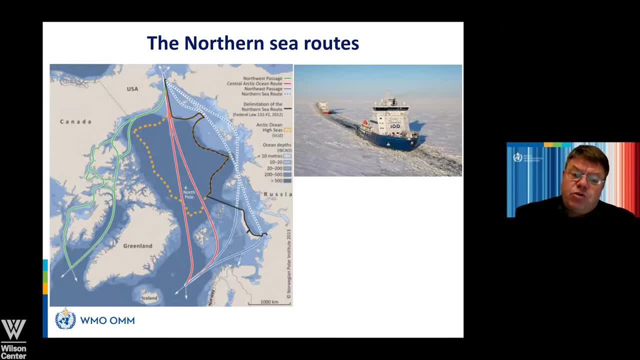 And by the 2040s we expect that the shipping routes will be open in summertime and autumn time, but the winter will still persist and you should keep in mind that especially these Russian Arctic sea routes are fairly shallow, which means that the biggest 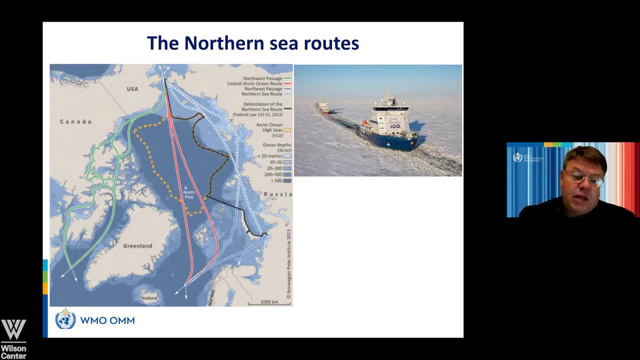 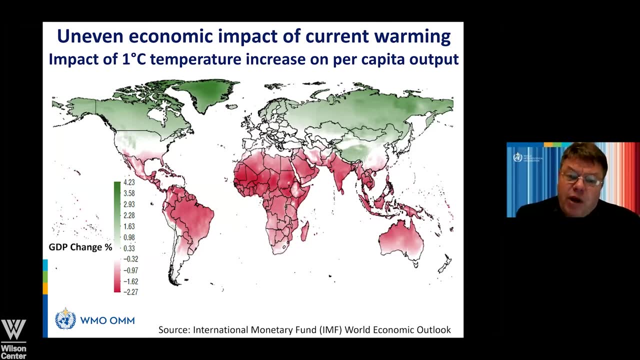 container ships couldn't be used in that area, And IMF has estimated that this already seen. one degree warming has had a positive impact on the economies of high Northern latitudes. It's a long growing season, the forests are growing better and we need less energy for heating of the premises. 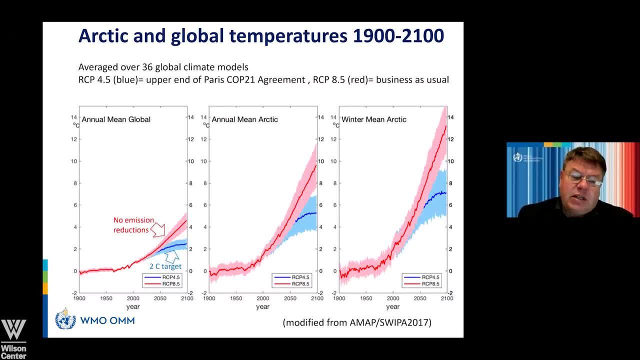 And the future in the Arctic looks such that we expect to see at least double the global warming. So if you would reach two degrees globally, which is this blue curve? which are these blue curves here? we would reach between four to five degrees in the Arctic. 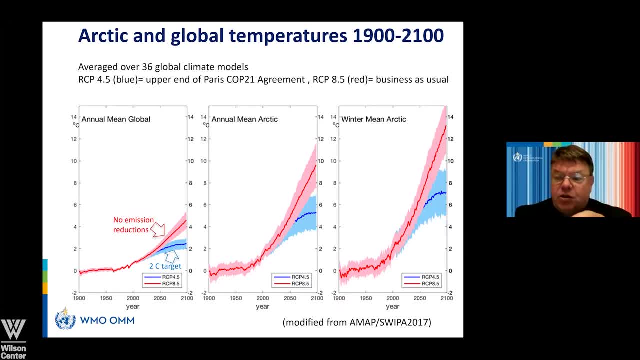 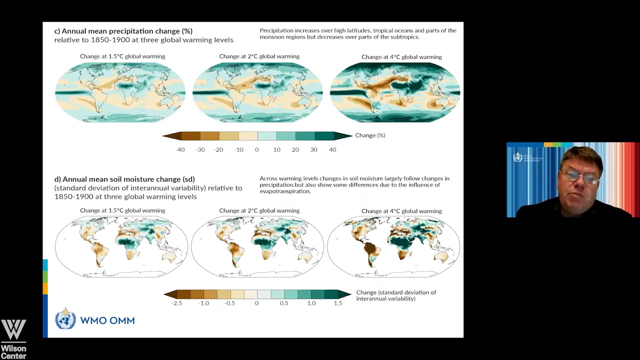 and at a much higher temperature and in winter time, around seven degrees warming. And if you fail with the mitigation then the numbers would be fairly dramatic: up to 10 degrees on annual average and around 13 degrees during winter time. This is from the most recent IPCC report. 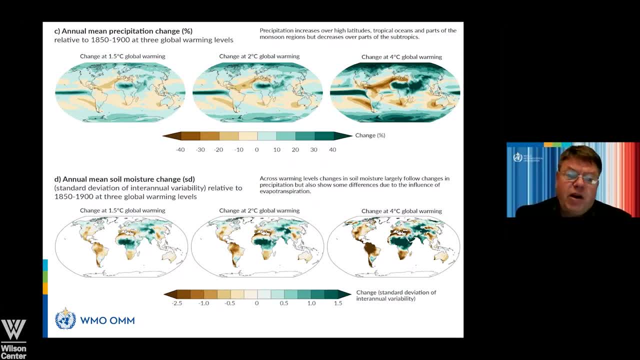 what's going to happen to the rainfall amounts, which is on the upper panel here, and what's going to happen to the- you know, the climate changes. So these are some of the things that we expect to have in the Arctic. 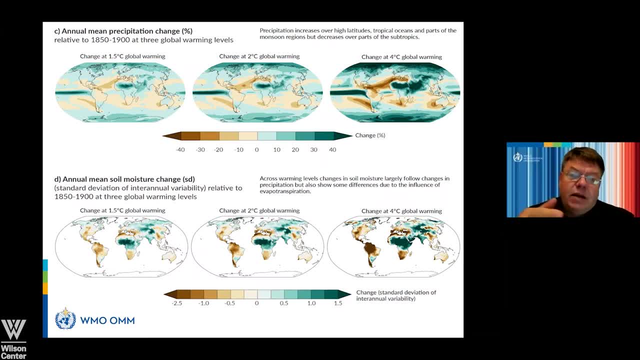 soil moisture, which is in the lower panel here and dependent on the warming rate- 1.5 to 4 degrees. we would see anyhow more rainfall in the Arctic and in most cases we would still see a growth of the soil moisture in almost all of the cases. 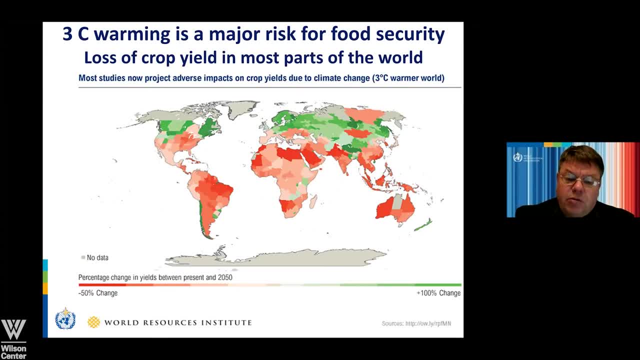 And the World Resource Institute has estimated what might happen if you reach 3 degree warming. what would happen to the crop yield worldwide? and you can see lots of reddish color which indicates loss of crop yield, whereas at the high northern latitudes you see lots of green color which 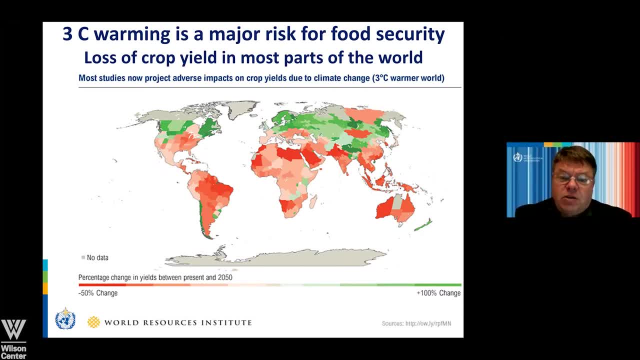 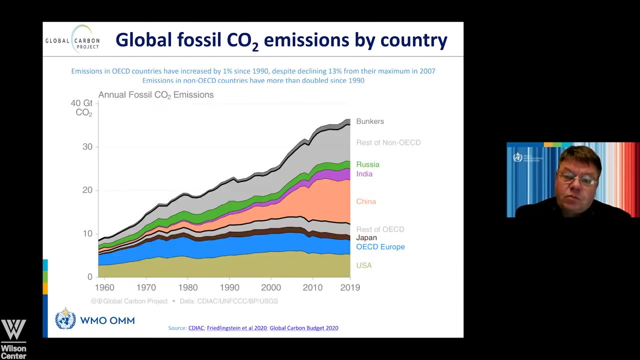 indicates again that basically the agricultural conditions are improving there, but the soil is not the most suitable and of course this solar radiation is limited, so it wouldn't solve this loss worldwide. And finally, a couple of words about the perspectives of mitigation. You know, of course, that the biggest emitter today is China and number two here. you can see the rest. 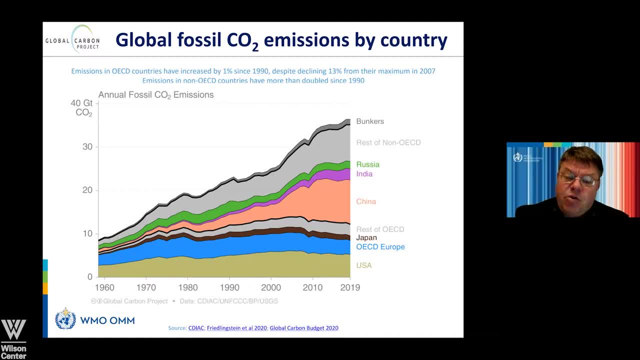 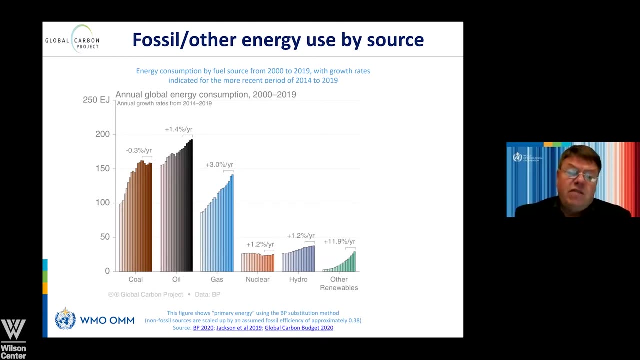 of non-OECD countries, where emissions have been growing also fairly rapidly, And number three is USA, and thereafter it's always EU. And the challenge that we have ahead of us is that we produce 85% of the global energy for energy production industry and transport sector based on nuclear, based on fossil fuels and only 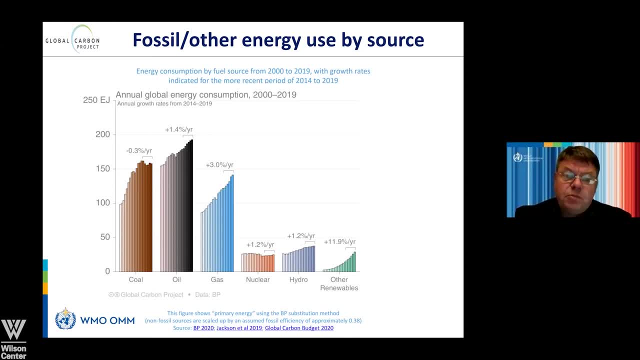 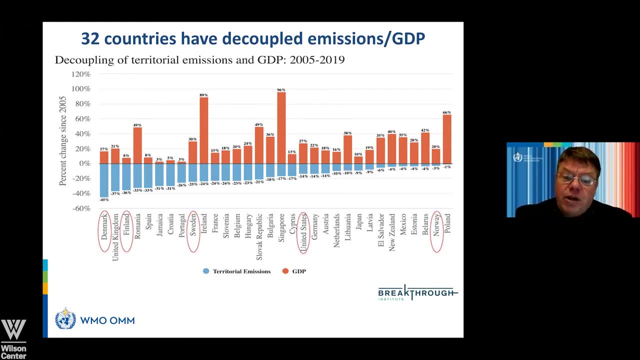 15% based on nuclear hydro renewables. Good news is that many of the arctic countries have been able to reduce their emissions during the past 15 years. you can see denmark, finland, sweden, usa and norway, which have been dropping their emissions and, at the same time, 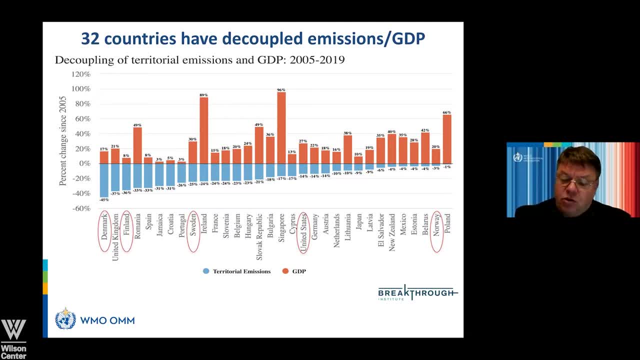 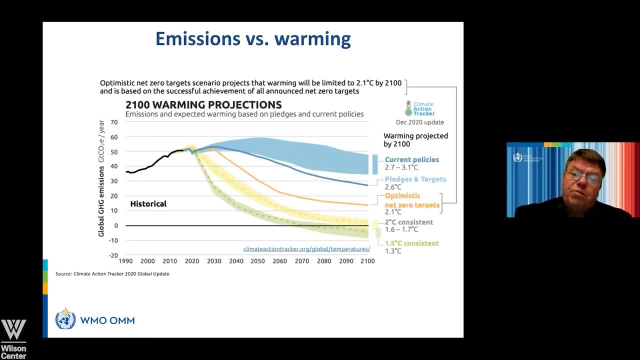 in all cases, we have seen economic growth. so this is uh, this is uh. this is positive news, and we are just preparing for this cop 26 meeting, which will start in one month's time, and at the moment we have pledges which would indicate 2.7 degrees warming, and from the un. 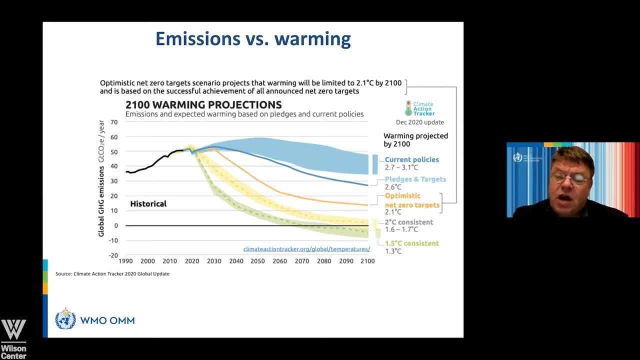 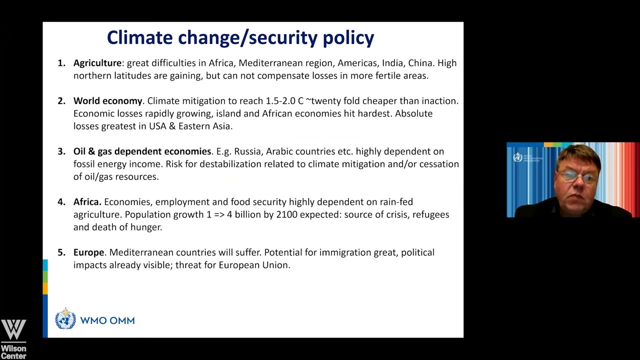 side. we would like to see at least the upper limit of paris agreement, two degrees target. the much more on the table. there have been lots of. there have been lots of political promises, but the concrete, the pledges, have been still missing. and finally, what this climate change needs from. 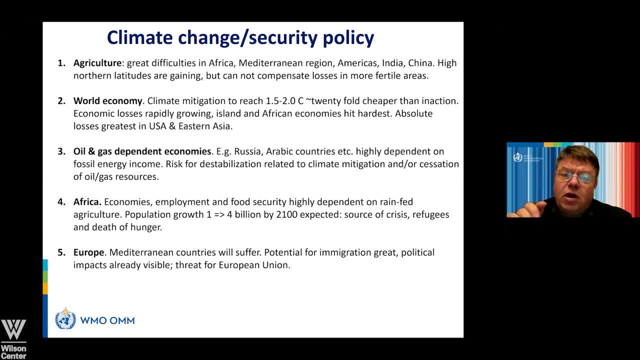 means from global perspective, where we would lose lots of agricultural productivity worldwide and these arctic areas wouldn't compensate, wouldn't fully compensate the loss of propel in those areas and it's it has been shown that the mitigation is much cheaper than than living with the consequences of climate change change, and the usa is the country where these 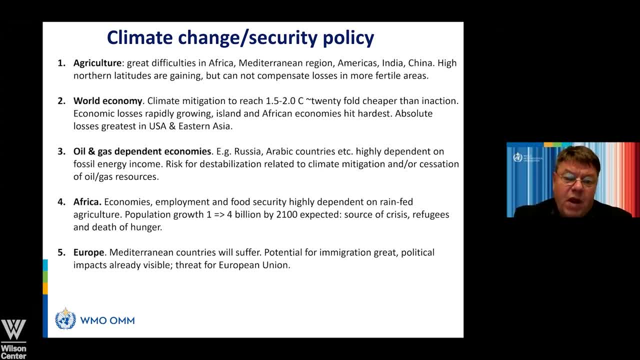 expenses have been uh is so far. and then it's a challenge for the oil and gas dependent the economies like russia: how, how to cope if you really start leaving the, leaving the resources in, in, in that, in in the ground and and that would be a challenge for for such such countries and 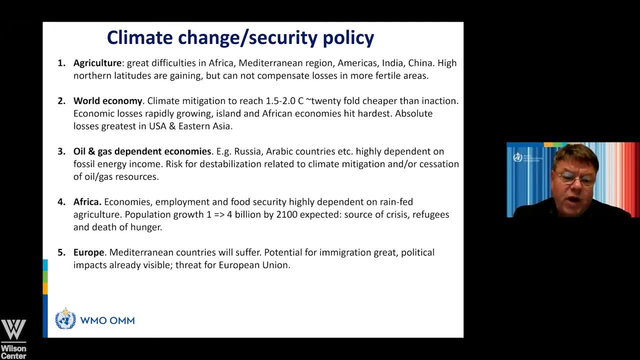 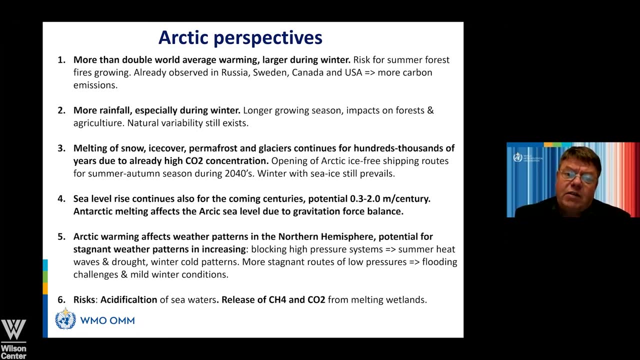 africa is the is the most challenging area worldwide: the population growth and and poorer climate in the future, And also in Southern Europe. we would see challenges in the future And, finally, what is supposed to happen in the Arctic. I already demonstrated that we would see. 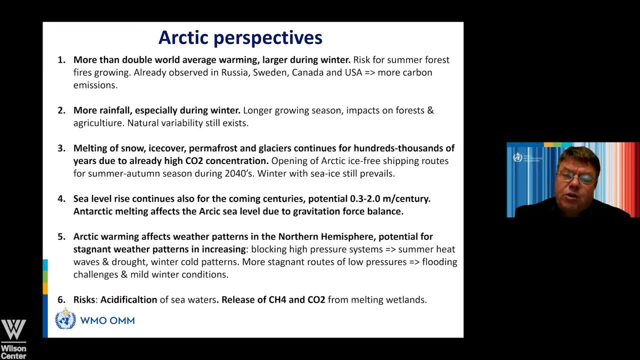 more than double world average warming, and especially during the winter season and in the summertime, the risk for forest fires is growing, and that's what we have already been seeing in practically all parts of the Arctic: Rainfall. we expect to see more rainfall. 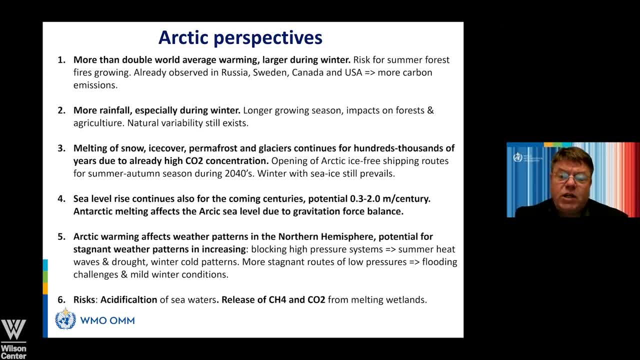 especially during the winter season and the growing season is already getting longer, and which has positive impacts on forests and agriculture. but we will also see natural variability in the future And this melting of snow, ice and permafrost and glaciers will continue for at least hundreds of years. 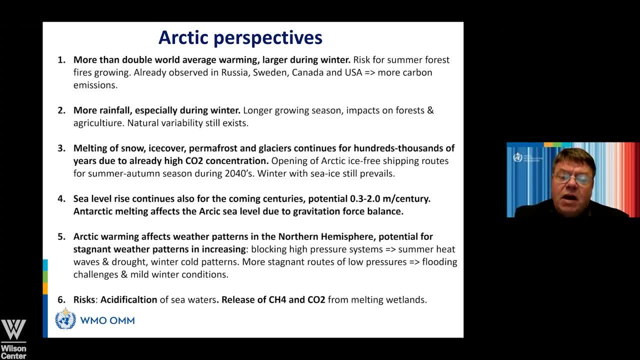 or even thousands of years, because we have already been reaching high carbon dioxide concentrations And I also demonstrated that we are going to see opening of the shipping routes. but one should keep in mind that the winter, with sea ice, still prevails and there's a risk. 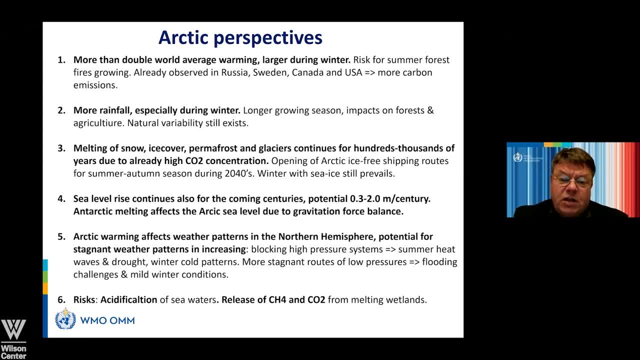 for major packed ice conditions, which would be an obstacle for the shipping. Sea level rise will continue for the coming centuries anyhow, and the range is from 0.3 meters per century and in the worst case we could see up to two meters sea level rise per century. 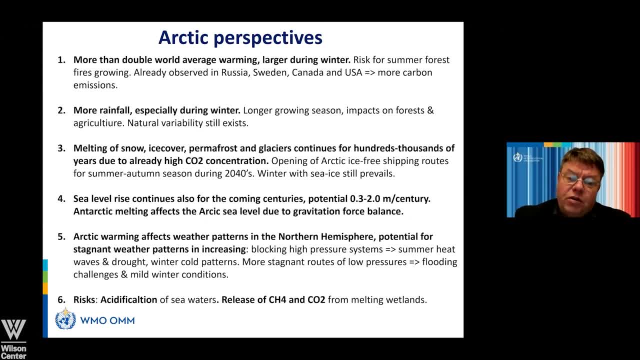 if, especially the Antarctic melting would take place in a speedier manner, And what happens in the Arctic Antarctic glacier is having a big impact on the Arctic. The Arctic is a sea level huge, And then there's a risk that we would see much more. 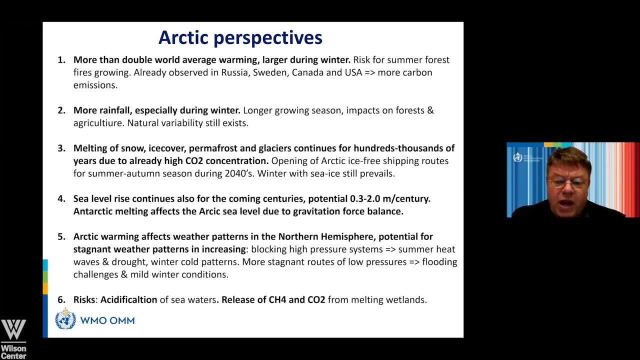 this kind of stagnant weather conditions blocking highs, which would mean in summertime heat waves and drought and in wintertime cold patterns. And again this would mean that the low pressure areas would have same tracks and this would enhance risk. 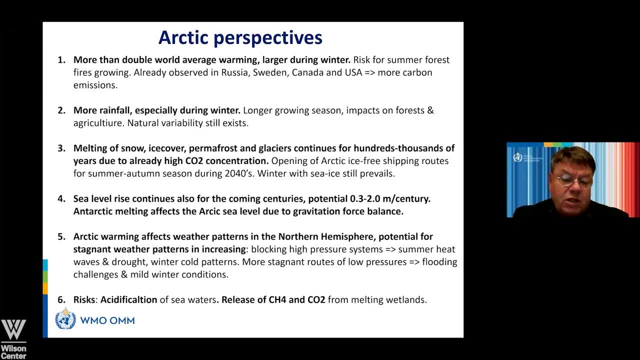 for flooding And, of course, mild winter conditions as well. And then there are certain risks that we have to follow: Acidification of the seawaters, that's clearly one of the risks. And then what's going to happen to the methane and carbon dioxide that has been stored? 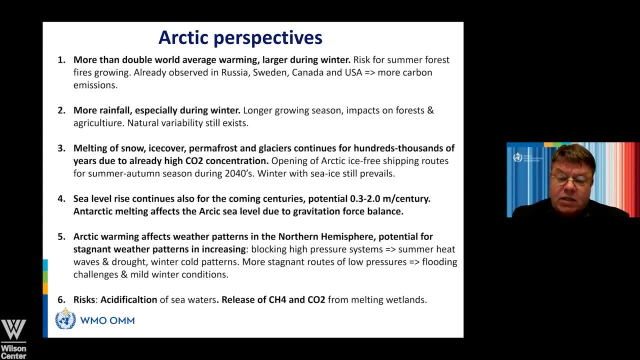 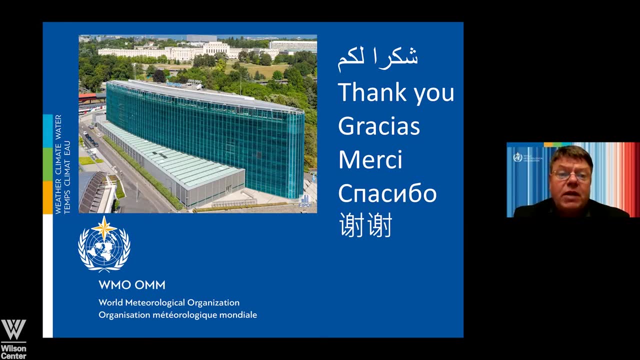 in the frozen wetlands? that's a question. So far we haven't seen a major outbreak, but that's something that we have to follow With these words. thanks for the opportunity to address you and I'm happy to answer any of your questions later on. 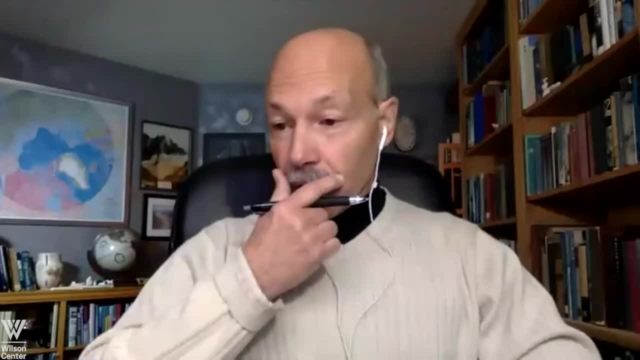 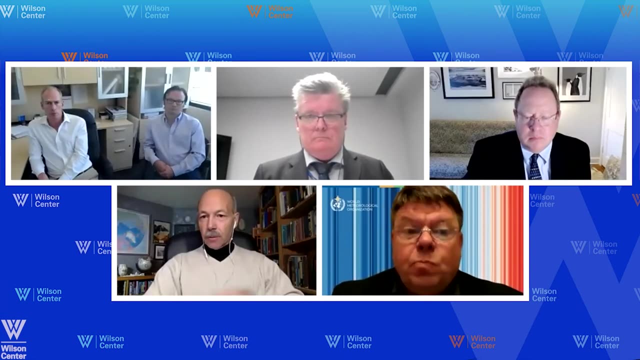 Thank you, Secretary General. thank you so very much for covering a lot in a very short period of time. I do have some questions, as the audience will come back around to those, But I think one particular theme I'd like to think about when we come back around to some questions is this: 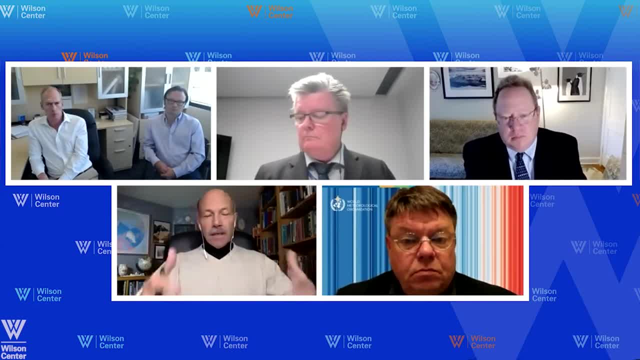 that these are my words, but in some ways, everything that you have just noted is baked into the climate, the global climate system. So your note, this sense of urgency here on all of our part, the fact that permafrost will continue to thaw. 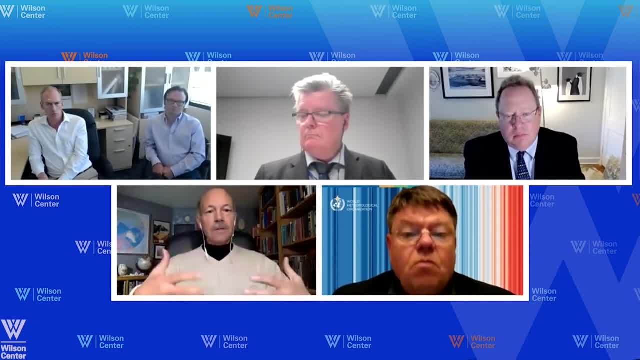 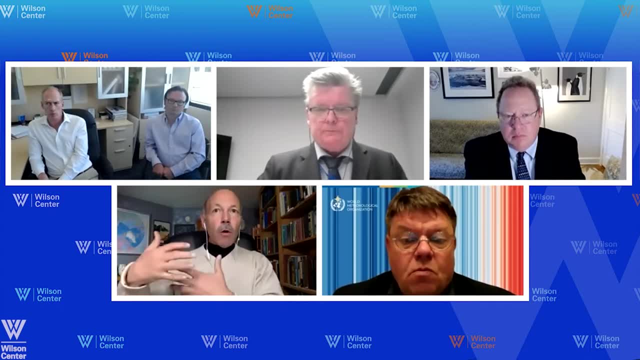 glaciers will continue to melt, sea ice will continue to recline. These are all baked into the current global climate system, no matter what we do today or in the next decade. And so what? all of those things you just addressed? they will be with us, our grandchildren. 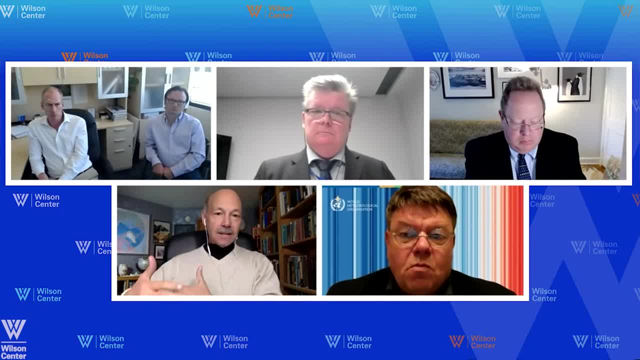 and our grandchildren's children for quite some time. hence the urgency and getting as much as we can done in a short period of time to mitigate what is really out- 50 years, 100 years- But we're dealing with what we were dealing with now. 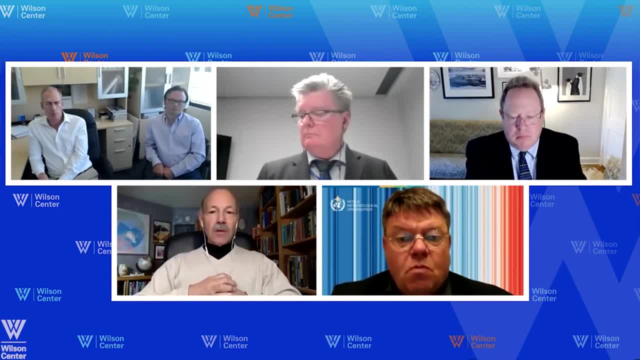 and there's no way to stop it now. So thank you very much for that. I do want to come back and touch that a little bit, including the ways in which you are trying to communicate this, the different ways you're trying to communicate. 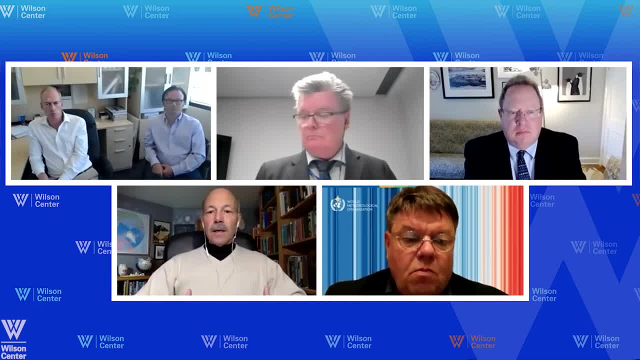 the very situation that we are in and how we can at least adapt and mitigate in the short to long term all of the issues that you just discussed, because we're all trying to do the very same things that you are doing, So thank you very much for covering so much. 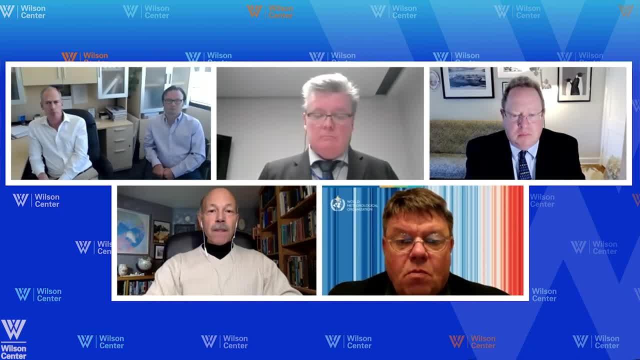 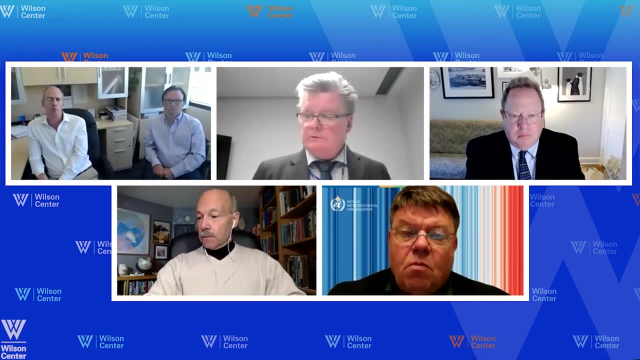 and so little time and we will come back to some questions With that. now I'd like to Ambassador, would it make it please take over the floor and your presentation, and I look forward to your comments as well. Thanks very much, Michael. 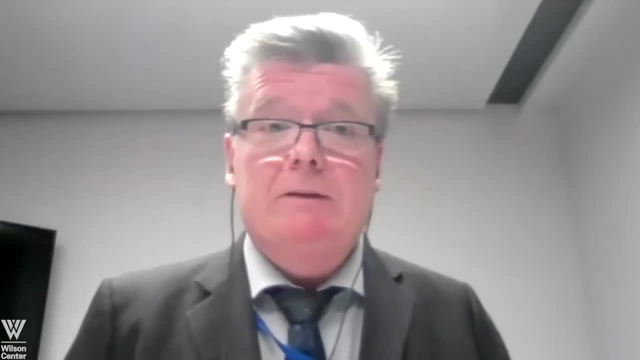 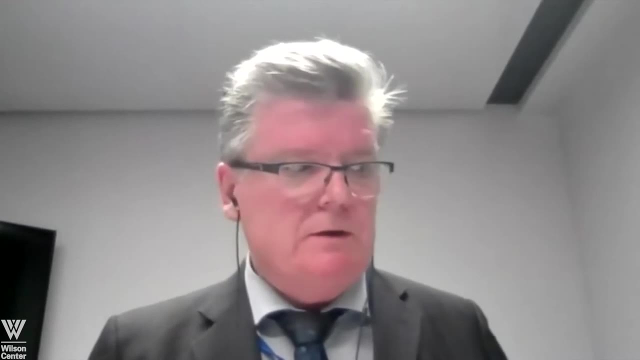 And greetings from the deserted foreign ministry. It's even later here than it's in Geneva and I have no idea if it's raining. It's a bit dark outside. Thanks for the invitation. Over the past year and a half I've very much enjoyed the Polar Institute's webinars. 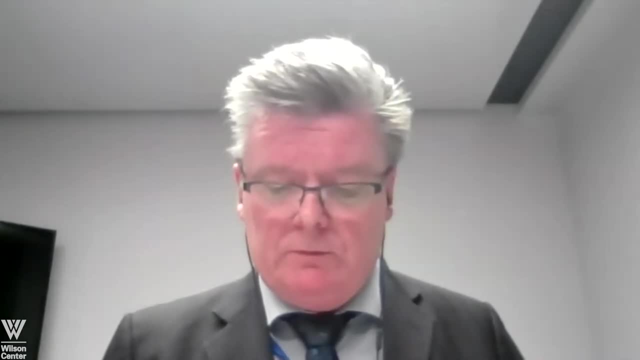 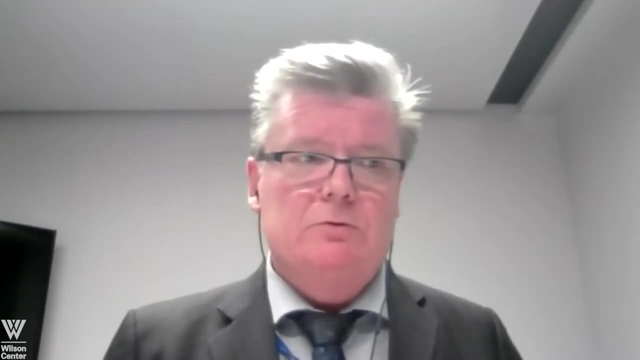 They've really been, top of the line, very interesting and thought-provoking. As I listened to the Secretary General, I realized that there's no way I can match his scientific knowledge, not even close, So I think the best that I can do is to offer a few. 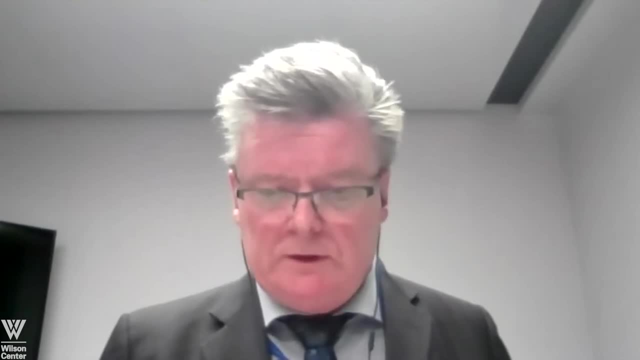 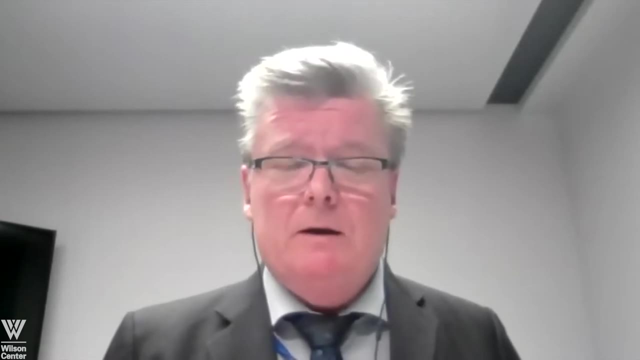 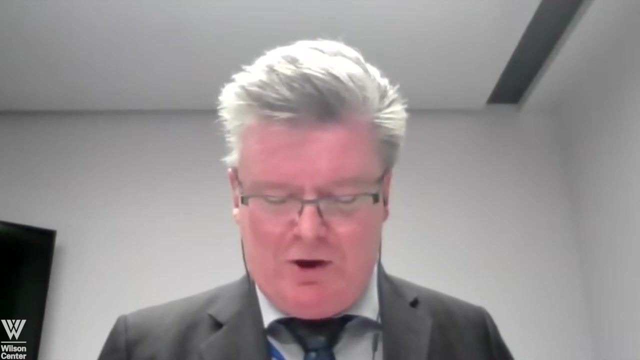 reflections on the theme of our discussion today. It also occurred to me that quite possibly this is the first international webinar in recorded modern history that has two persons by the name of Petteri in the panel. It's not that common of a name up here either. 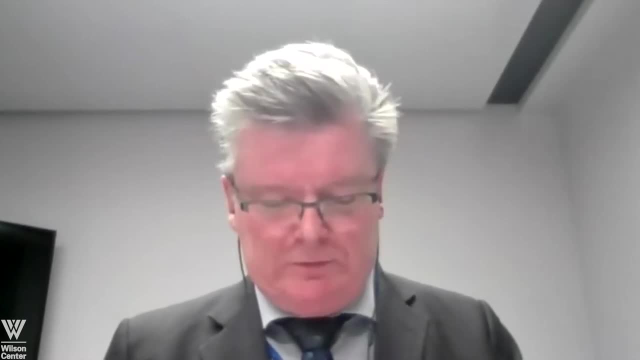 I'm just saying that And knowing where Mike's from and staying with the issue of climate and the Arctic and as Michael referred to and Heli did, Finland and Norway just conducted a joint trip to Alaska. Mike was there as well And I have understood from Heli and the other colleagues. 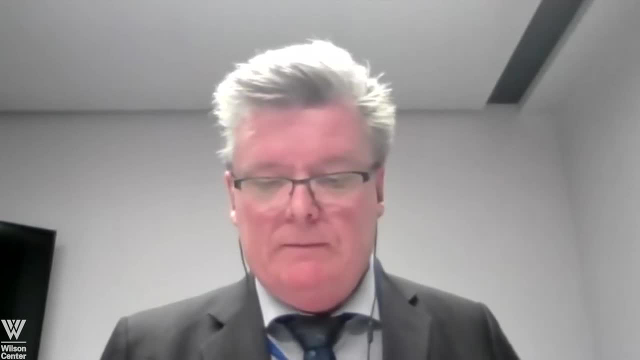 in the embassy that it was an excellent trip. In fact, Heli has repeated that fact to me several times and I take her word for it, And I do hope that the trip will lead to new concrete ways in connecting the US Arctic. 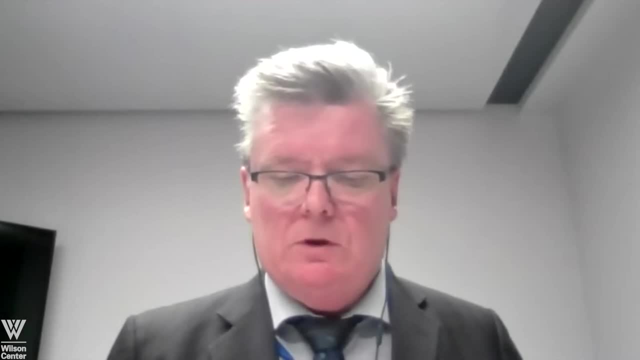 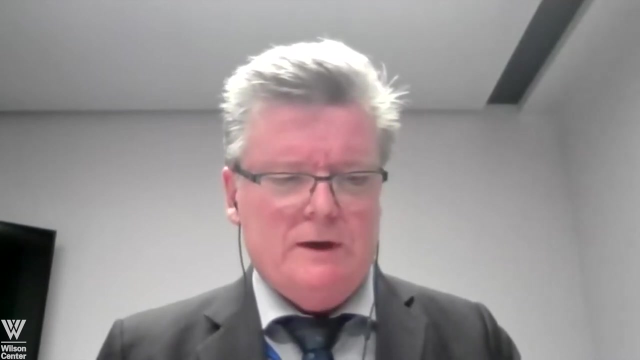 with us here in the Nordic countries even more strongly. We share many similar challenges and stand to gain from increased exchanges, And hopefully we'll be able to host a delegation of Alaska in Finland soon. On a personal note, if I may also say that a trip to Fairbanks, Alaska. 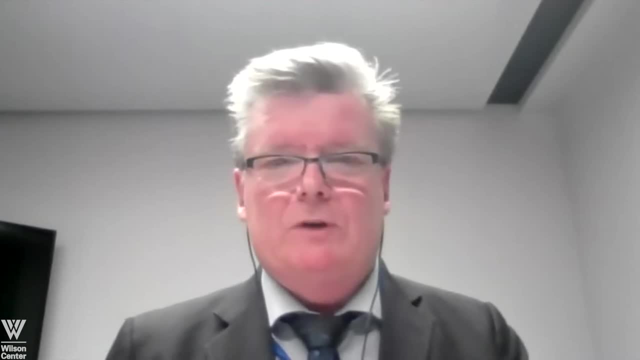 was the first pandemic-related trip that I had to cancel in March of 2020.. I was already in transit in Stockholm and late in the evening my US colleagues sent text me a message saying: Petteri, I hope you're not yet on your way. 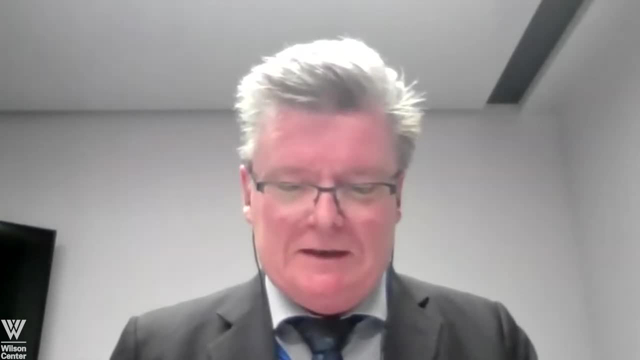 It's been canceled And ever since, one of the biggest objectives that I have in this post- that I would actually one day get to Fairbanks Alaska. So, Mike and all the other people listening in Fairbanks Alaska, can you please take notes of that? 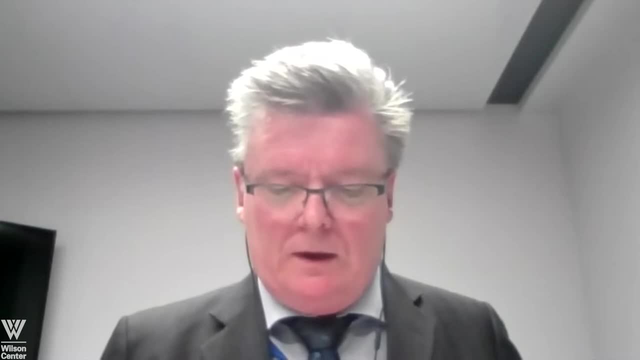 I'd love to come there. With regard to my country's relations with the United States, I'd like to also note that our president Sáulí Niinistön, special envoy John Kerry, have exchanged views on the Arctic and the importance of increasing ambition. 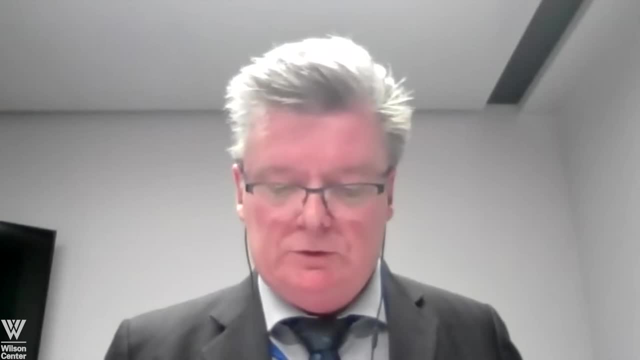 for example, in reducing black carbon and methane emissions. That work continues within the Arctic Council, particularly in its expert group on black carbon and methane, The EGBCM, as we affectionately refer to it. EGBCM refer to it, and we should really make sure that this super year for climate diplomacy 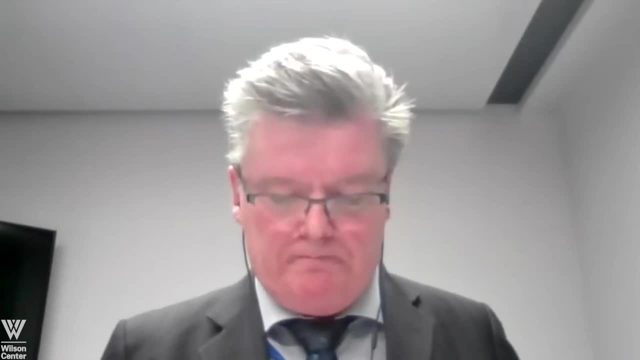 helps to highlight this work globally. With regard to climate and, obviously, being Finland's senior Arctic official to the Arctic Council, when someone starts talking about climate to me, I start talking about Arctic Council to them and I never stop talking about the Arctic Council. When people get very tired of me talking about the Arctic Council, I then start talking about the. 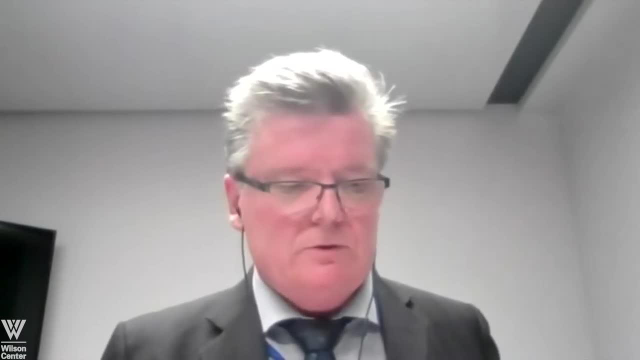 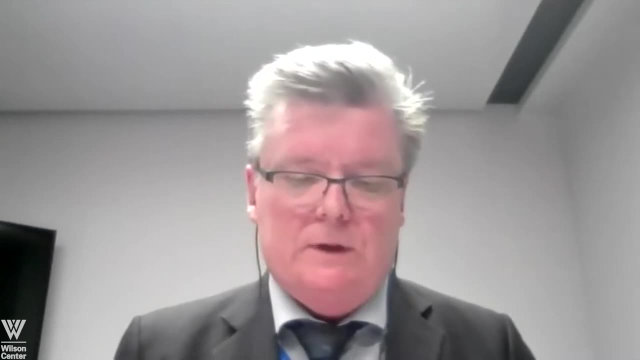 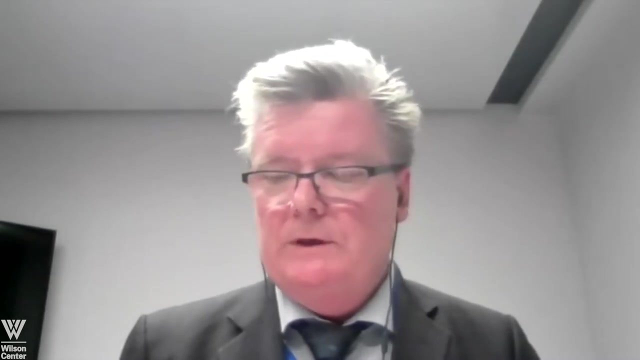 Antarctic Treaty, which I think is also of tremendous importance. In the Arctic Council this year we celebrate our 25th anniversary and I was very pleased to be in Reykjavik in May when the eight foreign ministers and the permanent participants reached an agreement on the Reykjavik. 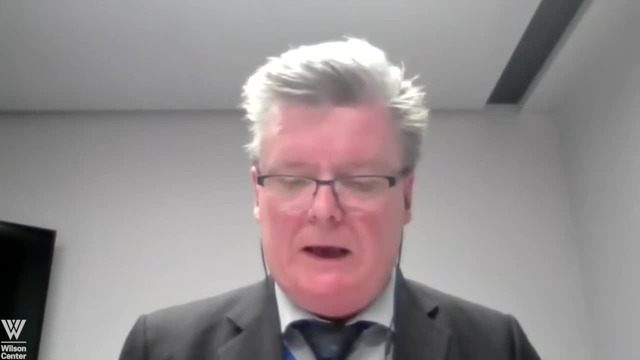 ministerial declaration And our first ever strategic plan taking us to 2030.. I think both are good documents, in my humble opinion. I've spent tens and tens of hours in the spring drafting them with my colleagues and I can just assure everybody that drafting documents virtually is not fun. 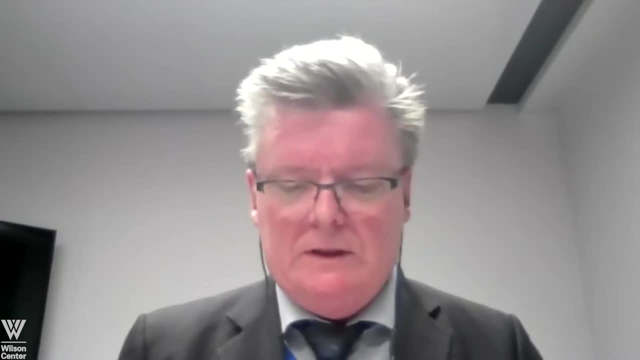 to put it mildly, but I'm very glad that we got there in the end. The right-hand side of the equation is that the Arctic Council is a very important part of the project. The Russian Federation is currently at the helm of the Council and quite possibly they. 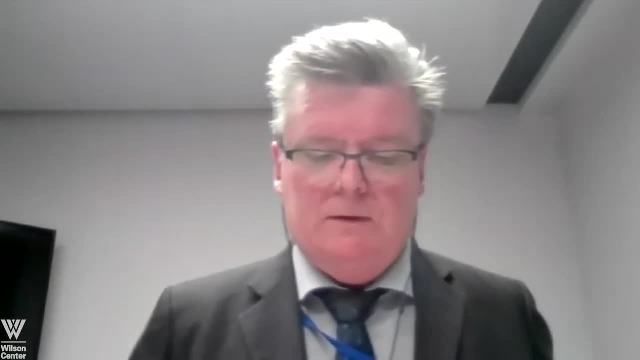 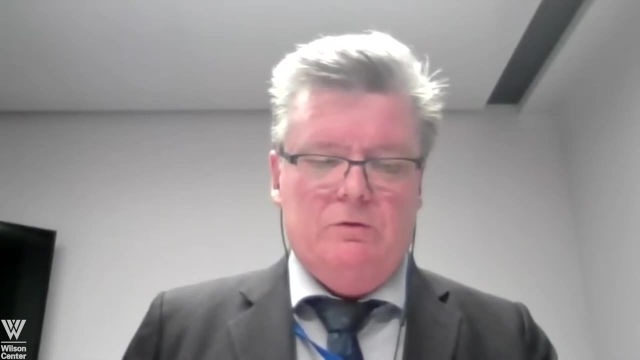 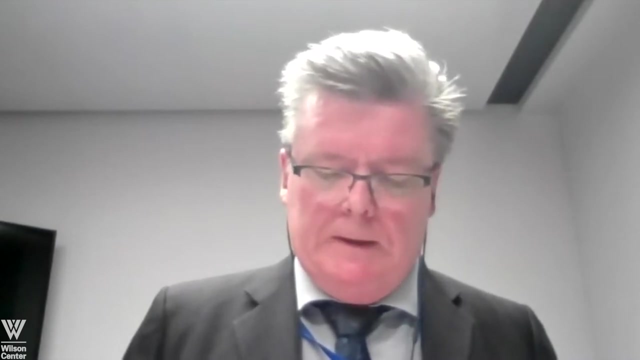 have the most charged and ambitious program ever. If I was to take part in all their planned events, I think I would basically need to move to Moscow or somewhere in Russia. There's an enormous amount of events which have been planned, and I have kept saying that the Arctic Cooperation does offer a way. 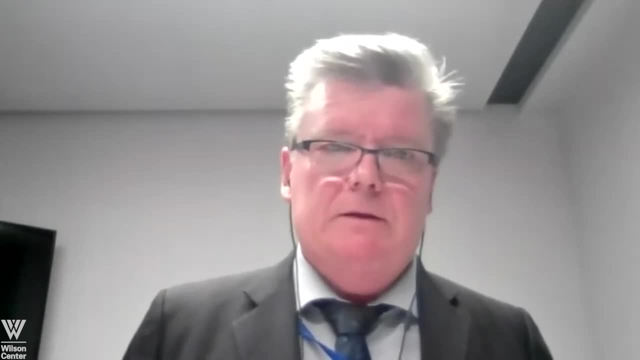 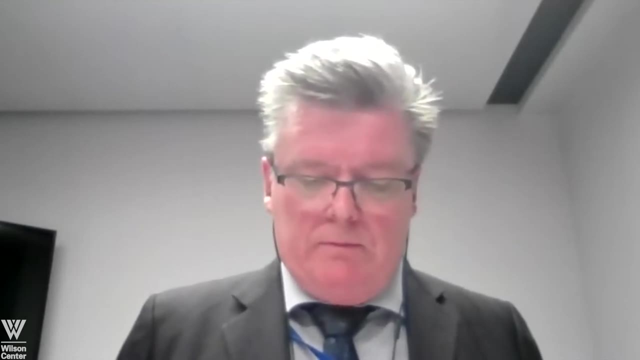 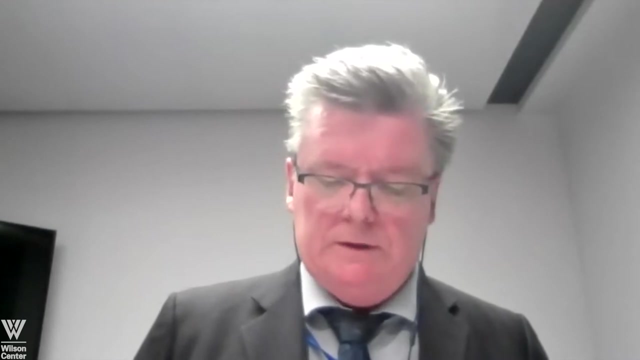 for constructive engagement with the largest Arctic states, the Russian Federation. despite the challenges elsewhere, The important thing, however, is to ensure that climate change continues to remain at the very top of the Arctic Council's agenda and priorities, together with the rights of the indigenous people and sustainable development throughout the region. The importance of the 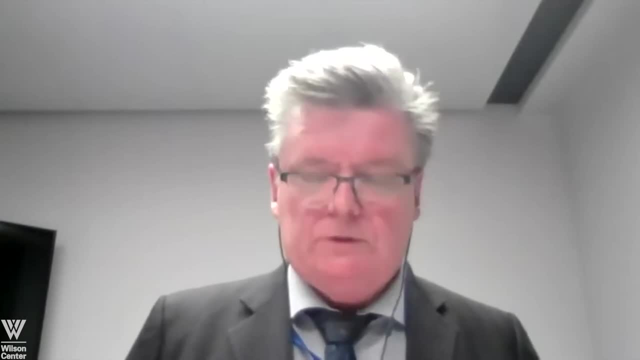 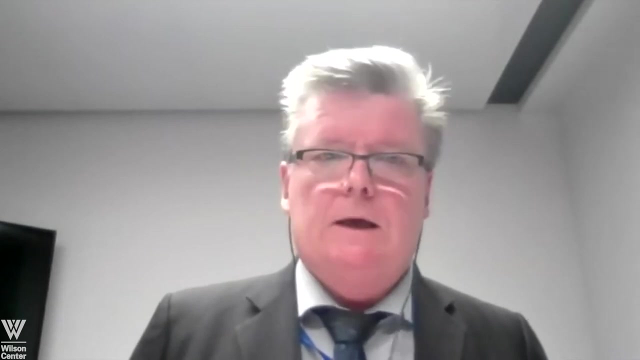 climate change was also very clearly acknowledged in our own National Arctic Policy Strategy, which we released early in the summer and presented with the diplomatic representations in Helsinki just a few weeks ago. I'm sure that the European Union's new Arctic Strategy, the Joint Communication which will come out next week, will also highlight the importance of climate and 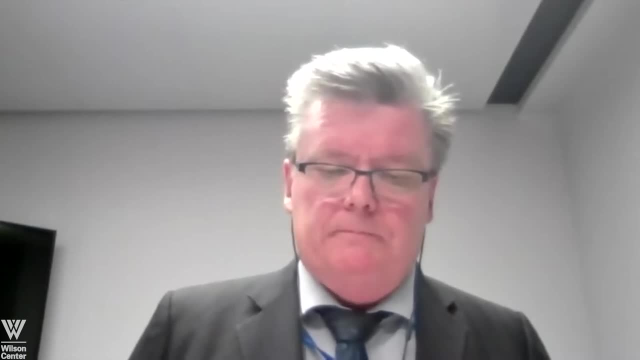 climate change, Mike. since science is the other important theme in this webinar, there again I'd like to underline the key role of the Arctic Council in that regard, and I think the Council is very successful in pulling together the scientific experts and producing high quality. 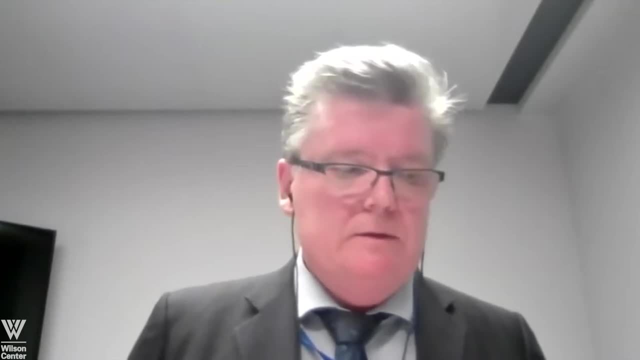 reports on a variety of themes. I think the importance of these reports has been acknowledged throughout the world. The work that our experts in our working groups do is really the engine of the Arctic Council, and I'd like to use this occasion if there should be any delegates in any of our 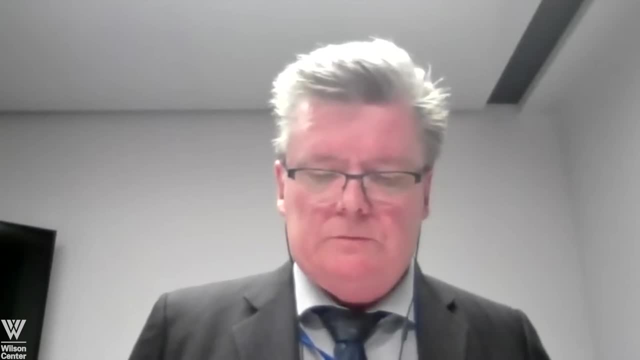 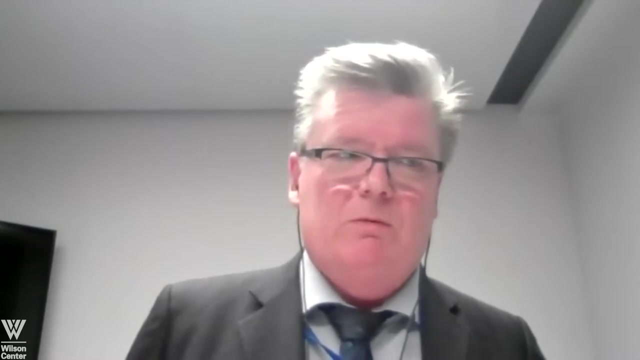 working groups listening to this discussion to just wholeheartedly offer my sincere appreciation and gratitude for your devotion and commitment. I think you all do a very, very important work. I think all the Finnish delegates are probably fast asleep by now, but I'm sure there are others around. 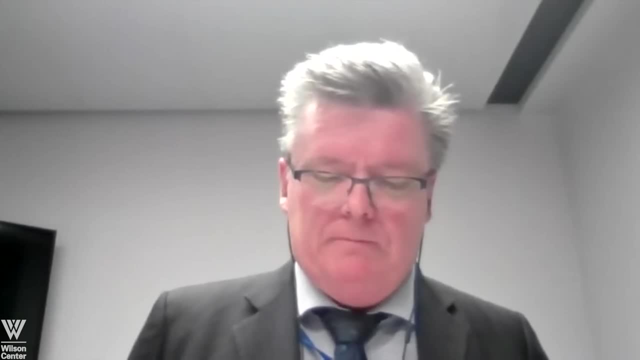 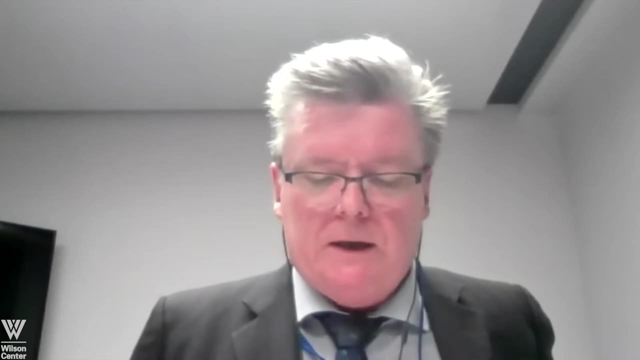 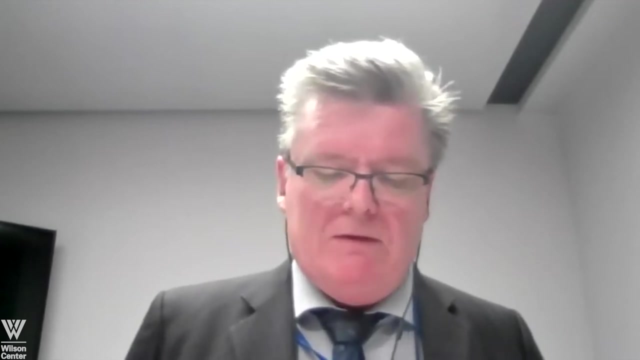 the world that might be listening to this. Thank you. The key issue for us and for the whole of humanity would be to study further the impact of climate change, but also the impact of the impacts of climate change. The climate change, as we all know, will have an impact on the environment and meteorological circumstances. 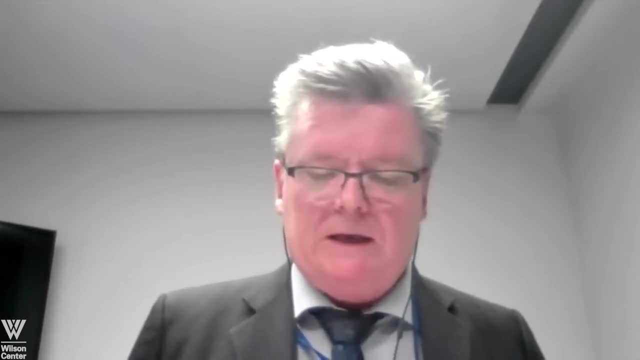 in the Arctic region and beyond, but then these impacts will further cause loss of human life and money because of the thawing, permafrost, flooding, landslide and countless other impacts. In this regard, the work underway in the Council's AEMAP and CAF working groups on the 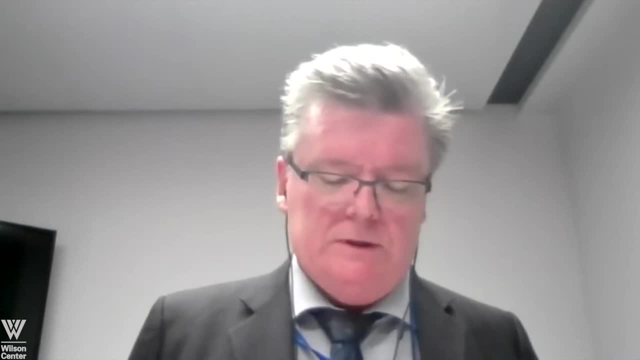 assessment of climate change and its impacts on Arctic ecosystems and ecosystem feedbacks will be of particular importance. the world around The climate change is an existential planetary level threat which is already underway and which has moved forward and will move forward. It presents us with a clear and present danger, however one looks at it. Ignorance, complacency and apathy are the worst we could now do Because of the arctic amplification. the Arctic region is at the very center of this process. The AEMAP working group refers to three-fold increase of temperatures in the Arctic. 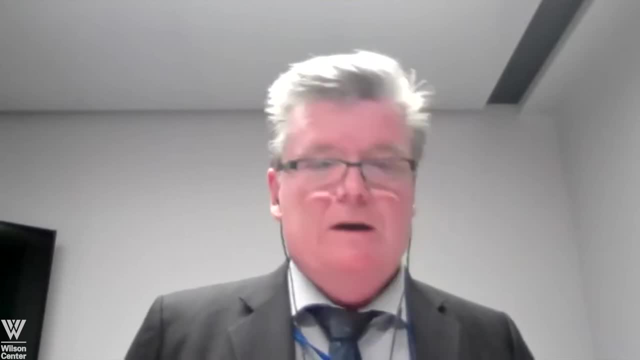 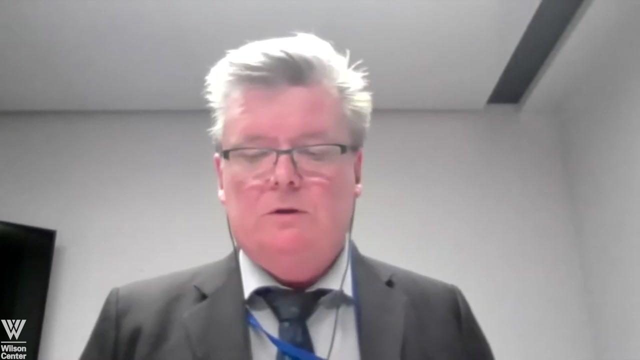 whereas the IPPC refers to more than twice, and I think the secretary-general just said at least uh, twice. um, if there still are people in doubt of the impact of our actions, i would imagine that the most recent ipcc report should put those doubts in rest by concluding, and i quote, that it is: 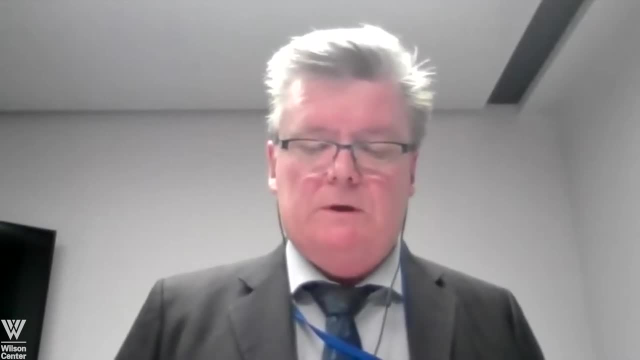 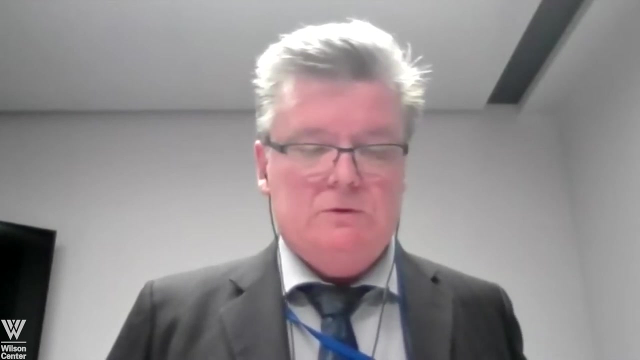 unevocal that human influence has warmed the atmosphere, ocean and land. widespread and rapid changes in the atmosphere, ocean, cryosphere and biosphere have occurred. to someone not trained in climate science like myself, that sounds convincing way beyond any threshold of reasonable doubt. in my current function, i will tirelessly try to do my little part in increasing awareness. 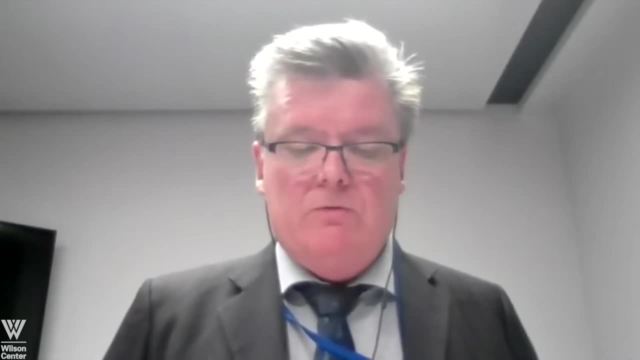 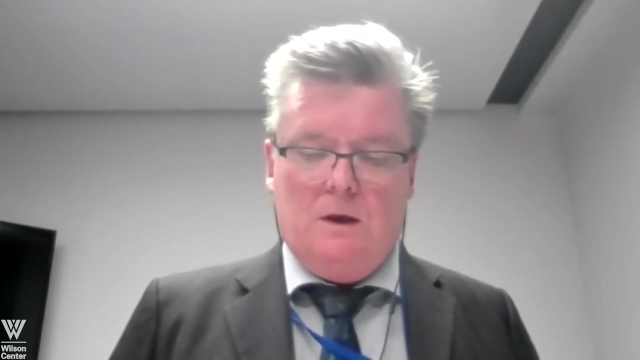 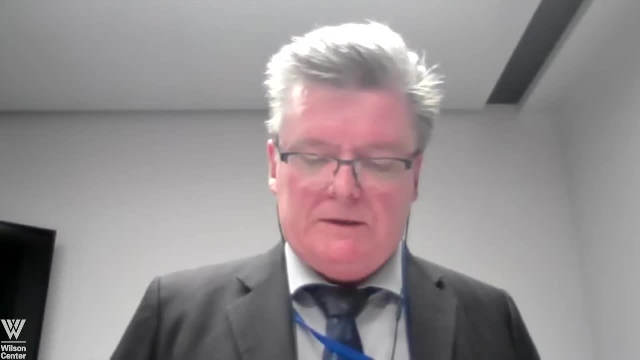 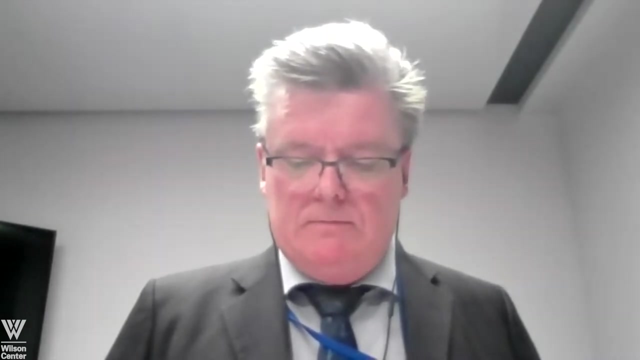 level. the reports both by the ipscc and aim up make it clear that the arctic which we currently have is not the same arctic we had in the 80s, and the arctic of today will not be the same arctic we will have in the 2050s. my son turned 20 few weeks ago, um, and i wonder what will his world? 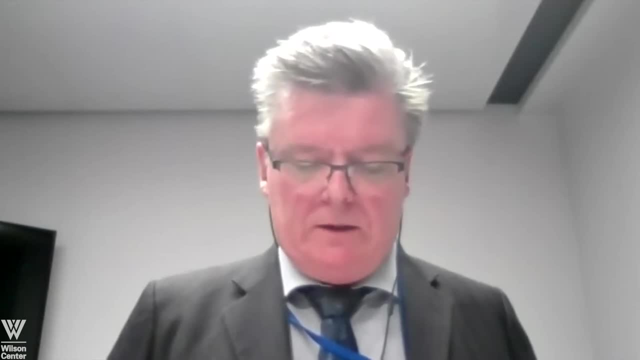 be like when he gets to be my age, and that thought worries me. to stop, slow down, control and adapt to all of this requires that our scientists spare no effort in revealing all the facts and all the predictions, however unpleasant it will be to hear them. we diplomats 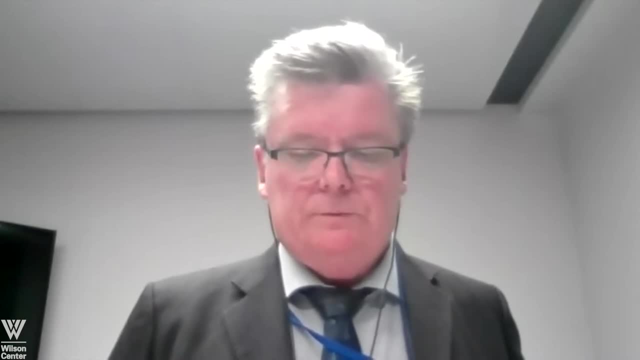 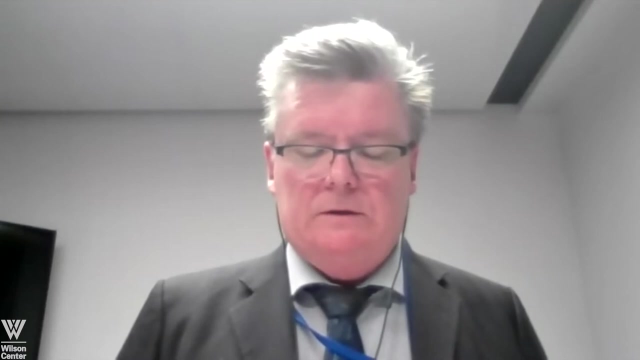 in turn must give that process all our support. in the arctic council we have also the legally binding agreement on scientific cooperation, which is a useful instrument, and the arctic science ministerials are very important gatherings of our scientists around the participating countries, and i look forward to the arctic science ministerial. 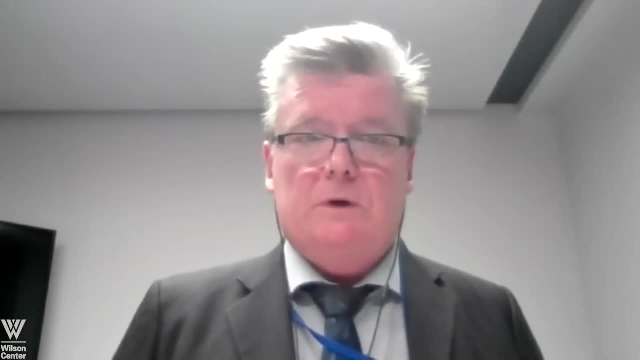 the fourth arctic science ministerial to be hosted by the russian federation and france in the next couple of years. in concluding um on science and education, um, i feel obliged and i want to also highlight the role and great work of the university of the arctic network, the new arctic, which is hosted by the university of lapland here in finland. 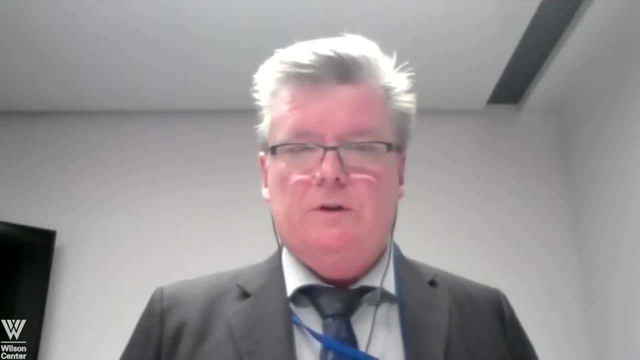 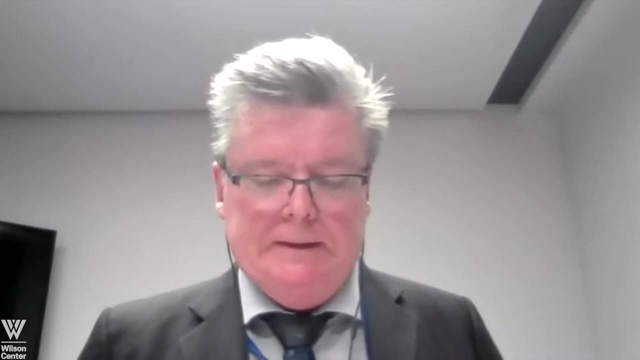 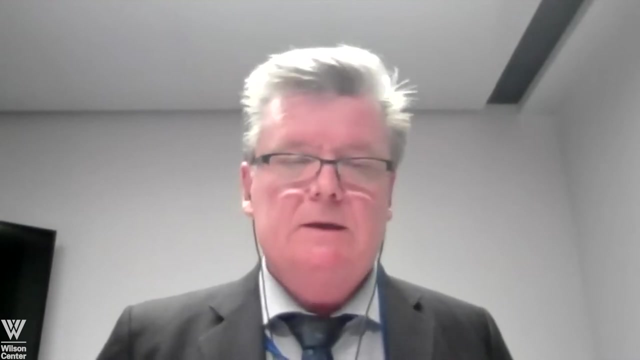 i attended, few weeks back, their celebrations for their 20th anniversary and delivered an address together with my us, russian and french colleagues. the new arctic currently has 200 members in nearly 20 countries countries and has activities in about 60 different thematic networks. That is an impressive achievement. 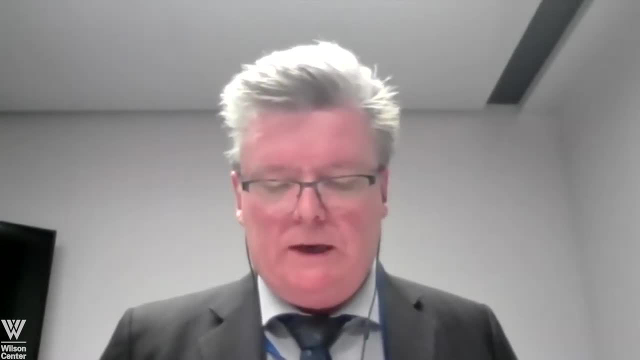 in my humble opinion. The final word that I just want to cite is to cite the letter that the President and Vice President of the EU-Arctic sent just before the celebratory event a few weeks back, and they said something that stayed with me. They wrote, quote: 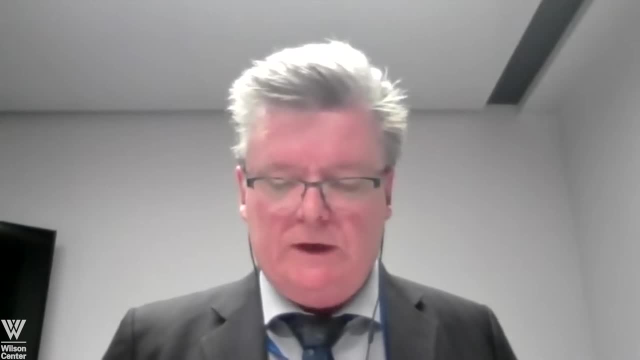 as an investment in human capacity. education is key component in any effort to create a sustainable future for the north and the globe. Universities are drivers of new ideas and communities of knowledge, and EU-Arctic is an expression of such community on a regional scale. 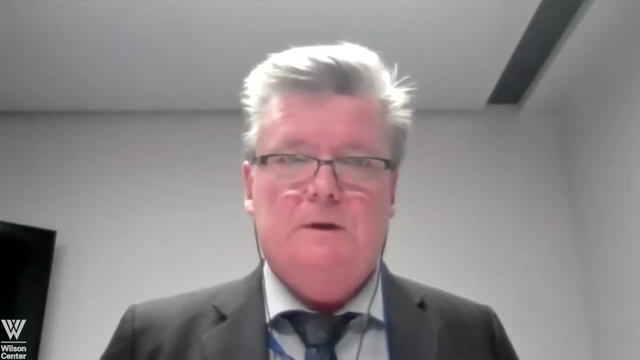 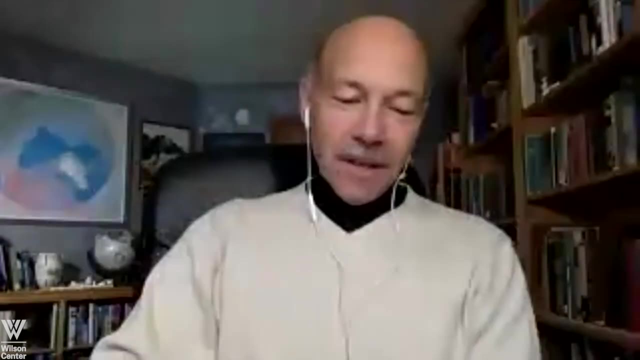 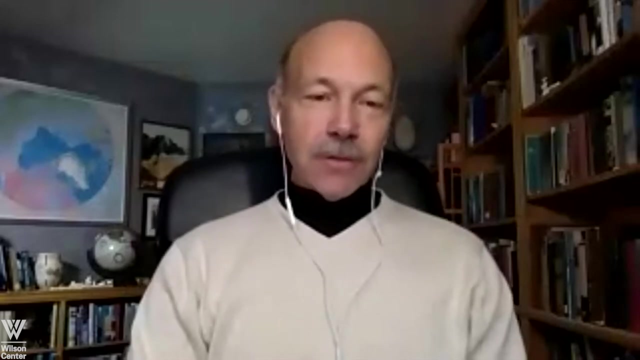 I can't really put it better myself, and with that that's my case, and thank you very much, Mike. Mr Ambassador, thank you very much Again. several notes here that perhaps we'll have time to circle back to. One is: I am so very pleased that you mentioned Lars Kullerud and 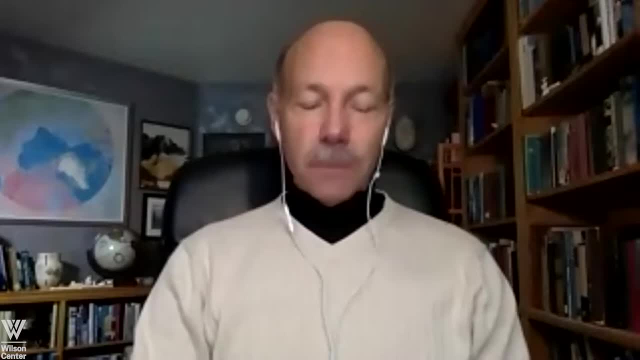 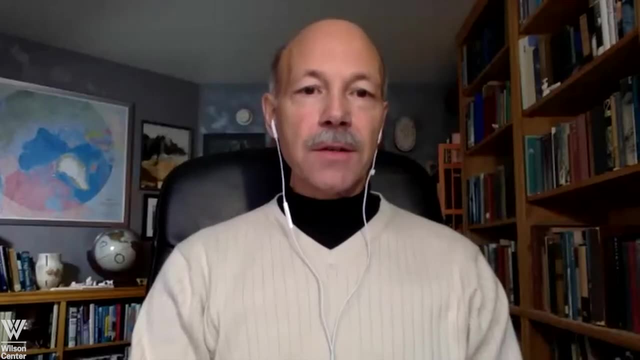 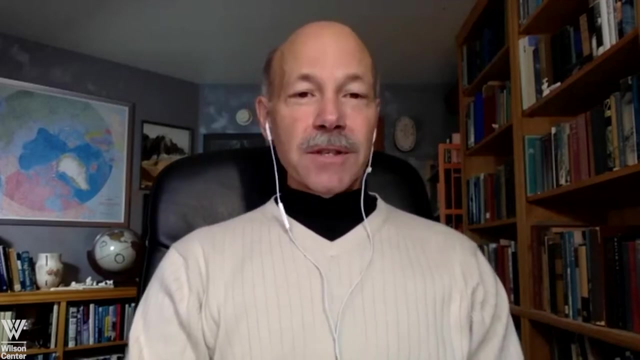 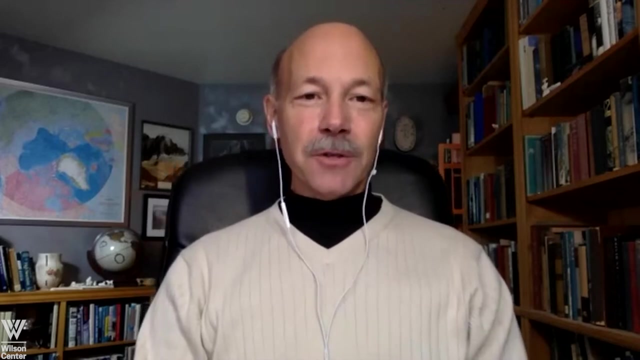 our friends at EU-Arctic. We've long been associated with them. We feel the same that there is a power in bringing together the intellectual capacity of the institutions around the north in service to the north, and I'm very pleased that you highlighted that work that has grown so much over the last two plus decades from sharing courses to now sharing. 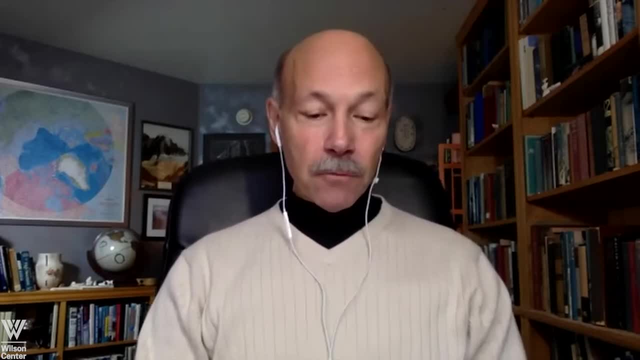 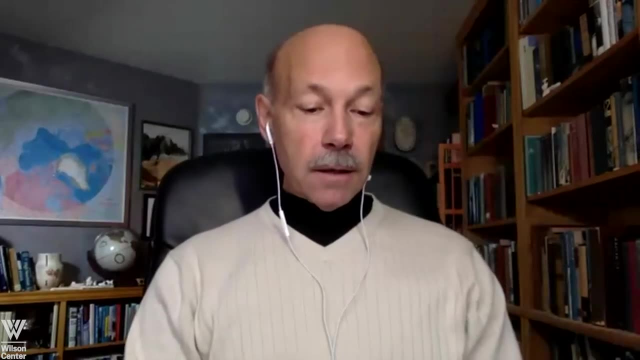 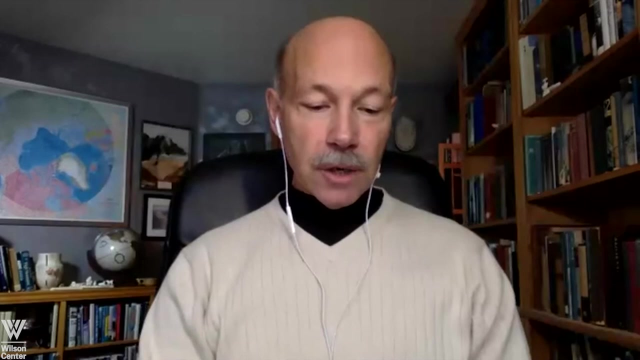 common solutions to common challenges. That's really very much appreciated. I also took note of the rest of your task list, starting with the groundbreaking note that we have two Petris on this, this program. We'll see if we can strive to find the third for some future program, I should note. 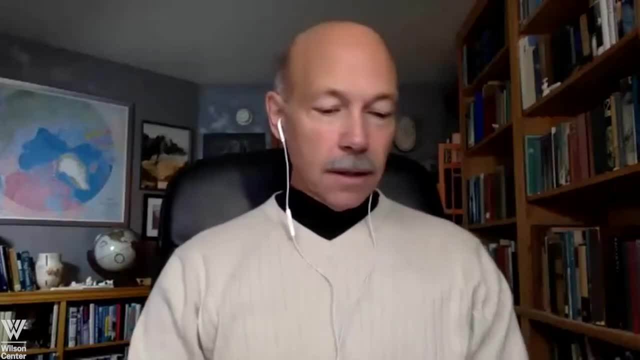 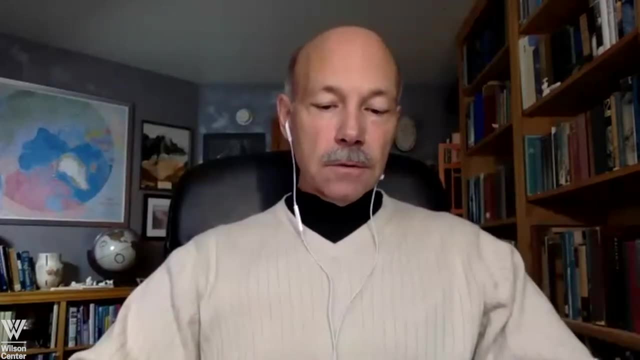 to my colleagues abroad that we had some problems with the audio at the very beginning, but those it'll be. this whole program will be posted on our website, so no doubt you will be able to listen to the comments you may have missed. Third on the punch list is an invitation to Fairbanks, Alaska. 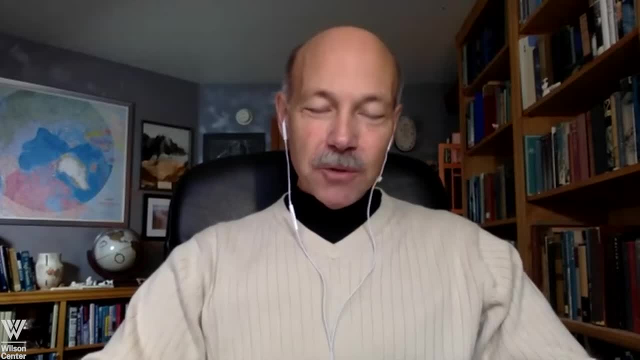 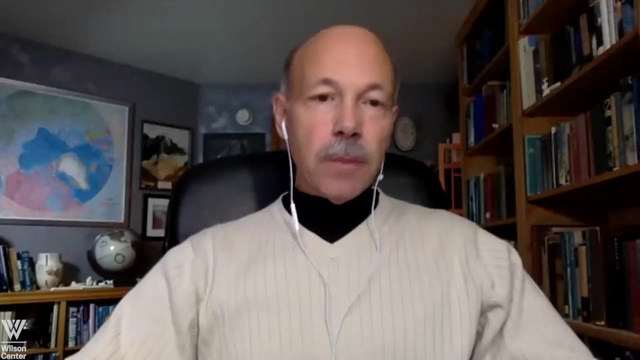 and I think Alaska would welcome you with open arms, Mr Ambassador. so you just need to tell us when and when the when the world allows, we'll make that happen. You noted this: the Venn diagram of your president, who has been very, very vocal, very well received, on both black carbon and the issue of 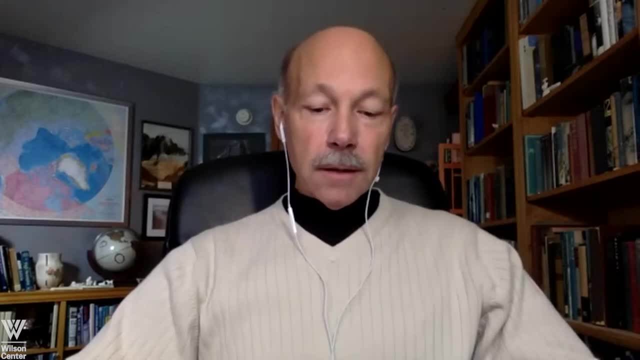 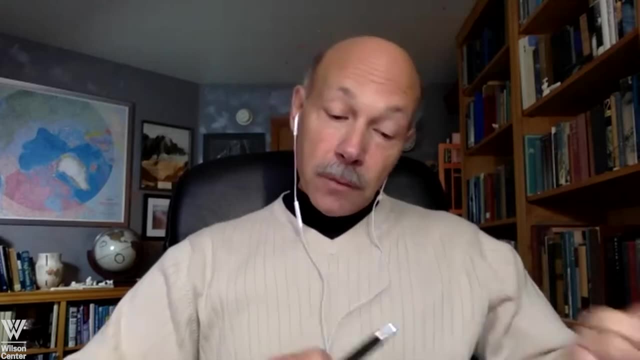 methane, not just in the Arctic but globally, and I've had the pleasure of speaking with him about that and the discussion with Secretary Kerry. that's noted- and then with my other new hat, as the incoming chair of the United States Arctic Research Commission. I'm most interested in all of 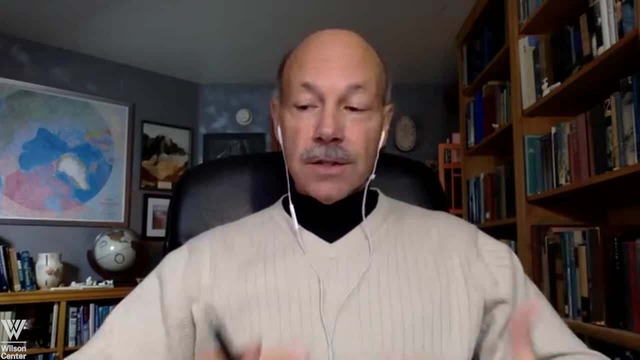 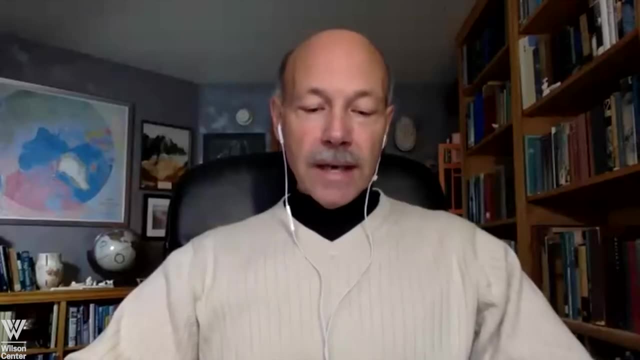 your comments related to how countries around the north can harness their scientific and research expertise and leverage all of that for the good of the Arctic. No one country can do this alone, so thank you for all of that, including underscoring the importance of probably the most consequential. 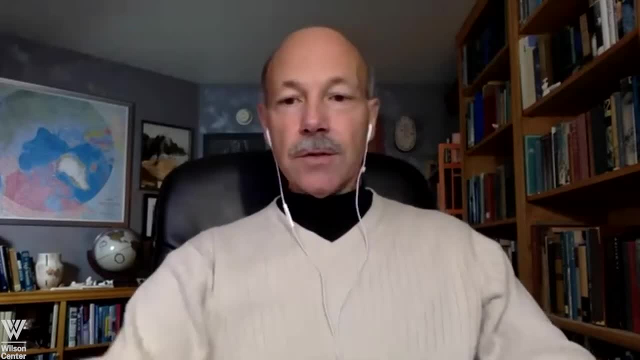 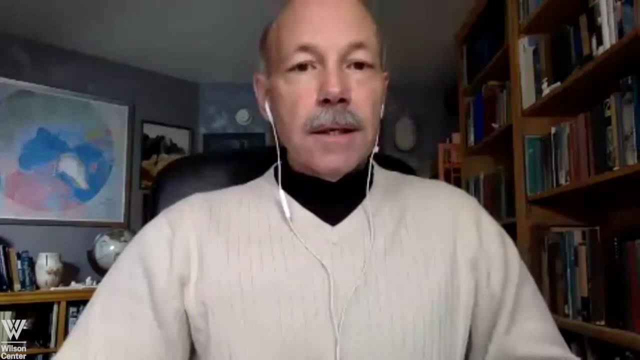 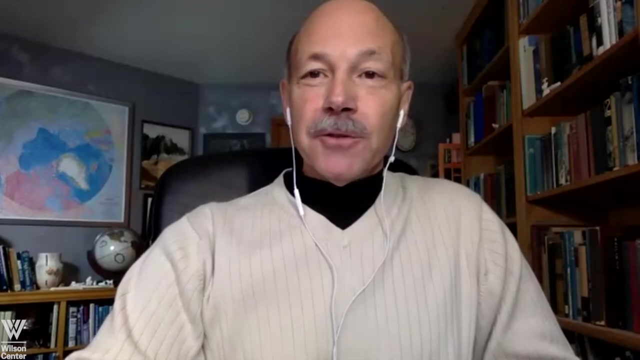 organization we have in place at the moment, which is the Arctic Council. so thank you very much for again covering so much in so little time. Now on to our third colleague, TJ Matamor, who serves as the Vice-Chancellor of Viisala. and TJ, thank you for allowing me to use the more common note for your 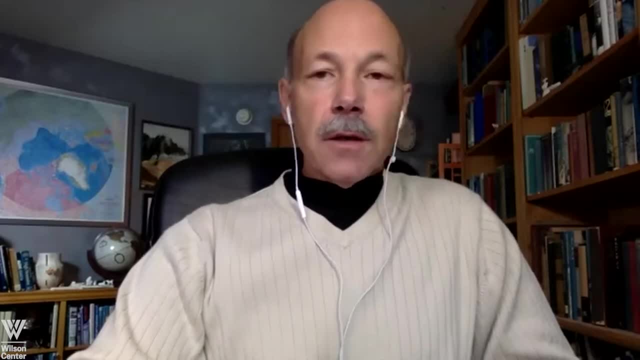 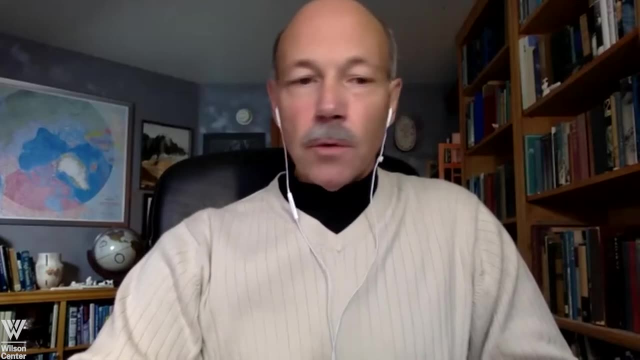 name, not Timothy, as preferred, but I want to thank you for being with us today and, if you would not mind, would you please introduce your colleague that's joining you today as well, and I will turn the virtual program over to you, Certainly and unfortunately that my colleague here is not a. 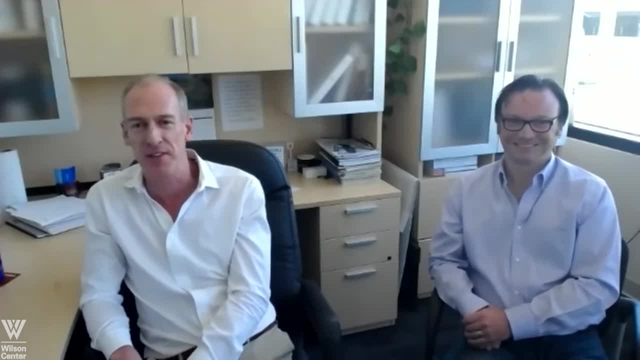 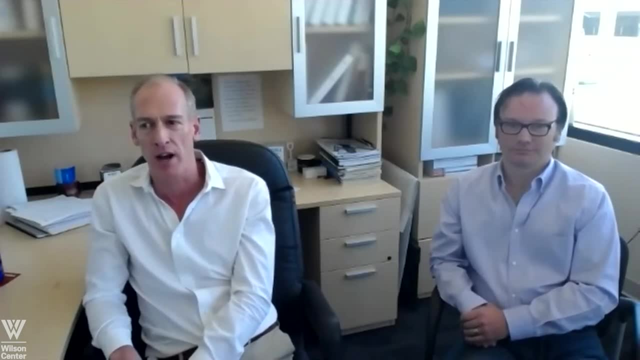 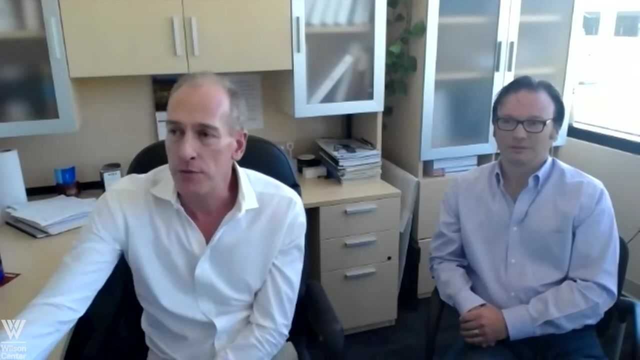 Petri, but we have plenty of Petri's at Viisala over in Finland. but this is our in-house meteorologist, Chris Vagaski, and he is much more knowledgeable than I on a lot of what we're going to talk about today, so I am very happy that he'll be joining us. So I'll just introduce. 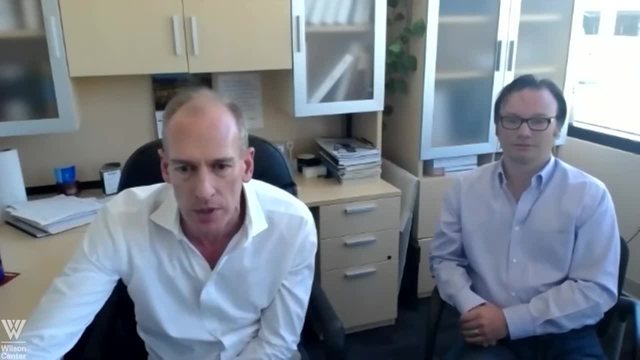 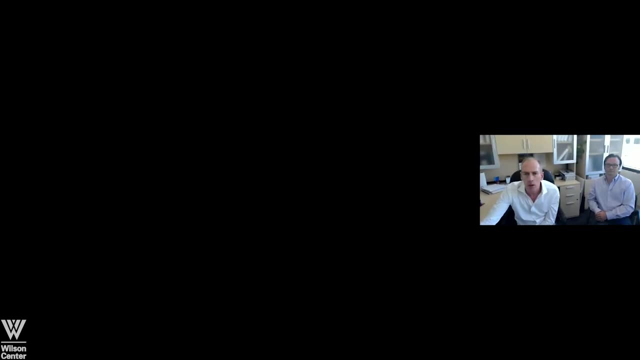 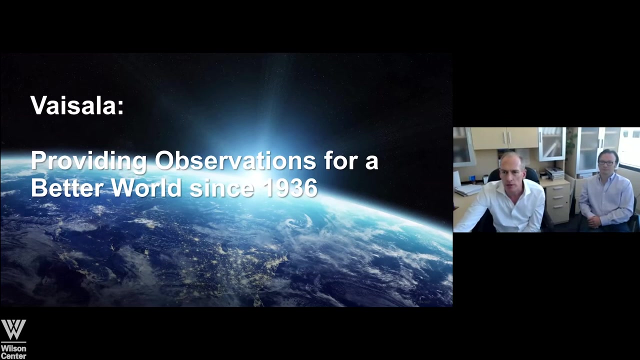 a few things quickly and then turn it over to Chris, but let me share my screen here, Okay, so hopefully you can see the slides at this point. So Viisala is a company based in Vantaa, Finland, just north of Helsinki. We've had a wonderful working relationship with Heli and the 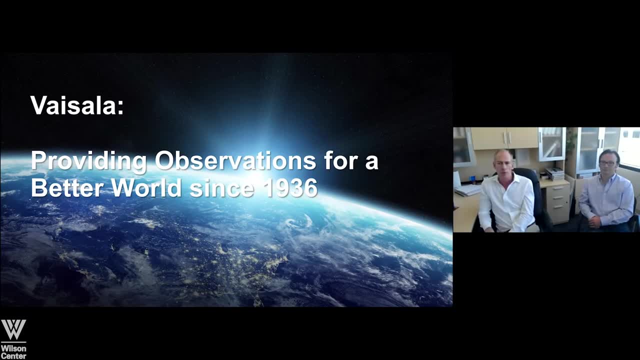 ambassador's office here in DC for many, many years, and we are based right now in Lewisville, Colorado, just outside of Boulder. It is 75 and sunny here, so I feel a little bit guilty talking about polar issues, but that's okay. So we're going to talk a little bit more about Viisala. 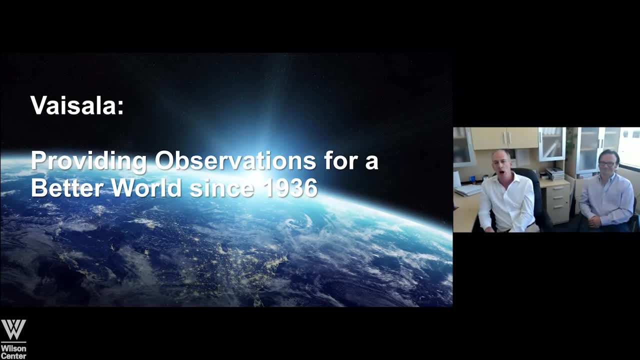 So we're going to talk a little bit more about Viisala. We're going to talk a little bit more about Viisala as well. Well, let me tell you what we do, and what we do now that we have the opportunity to talk. 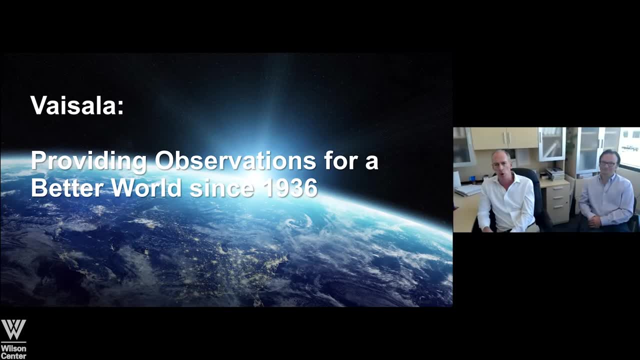 about a lot of the solar issues but we'll take the good weather while we can get it. But Viisala has been providing observations for a better world throughout our 85 year history. We do that through the manufacture of leading environmental measurement products and we're getting more into the data world and what I think Chris can provide and we at Viisala. can provide is a little bit more of how these observations are being taken in the Arctic and Antarctic, and we can really work with them as well. So I'm sure you can see this as well. So, if you would like to read- and I'll give you a few moments- 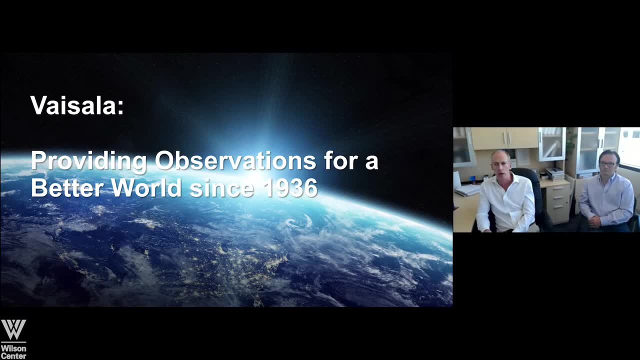 Arctic regions and some of the challenges they're in. So, with that, I'm going to turn it over to Chris. I'm going to give him the captain's chair here and let him steer from here. Okay, well, thank you, TJ, And thank you everybody for joining us today on what is. 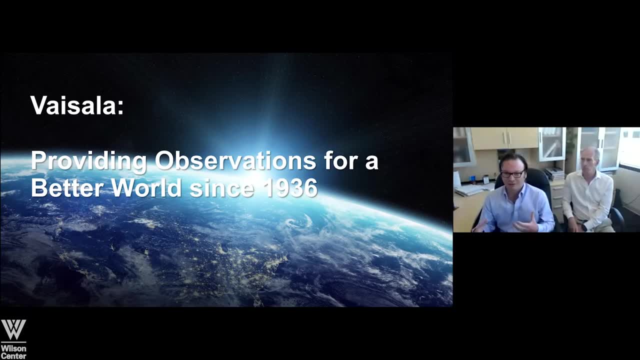 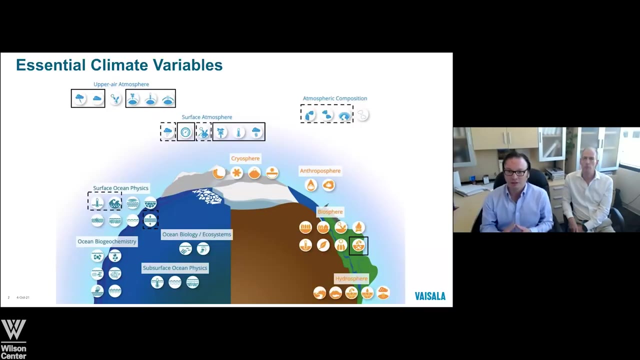 really an important topic, which is how are we measuring and how are we reacting to the changing climate in both the Arctic and the Antarctic regions? And, as TJ had mentioned, we do a lot of environmental measurements And from the WMO here is the essential climate variables that 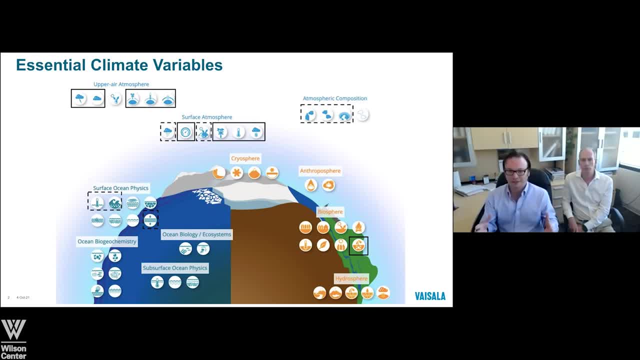 we try to measure- And there's 54 of these that go across the spectrum from the ocean to the atmosphere, the cryosphere and things that the humans are doing to the planet that we live in. And we can measure a wide assortment of these essential climate variables, ranging from 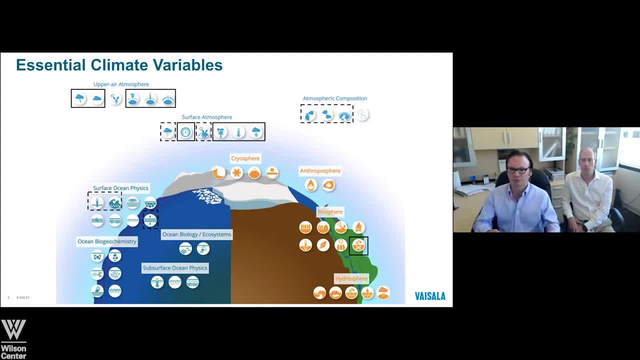 lightning to clouds, just the surface pressure, the temperature, even some of the sea state conditions, like the sea surface temperature and wave conditions, And so to be able to touch so much of these different variables that have an impact on the changing climate and how they're. 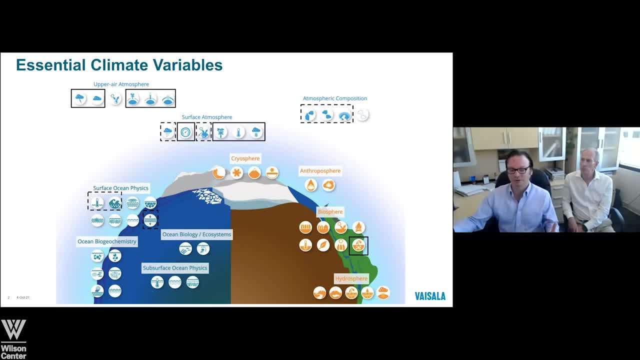 going to impact people, the plants and animals as we go into the future. it really is very meaningful to work for a company that can do this and provide that information to those researchers, those scientists, those policymakers that are determining how we're going to react to a changing 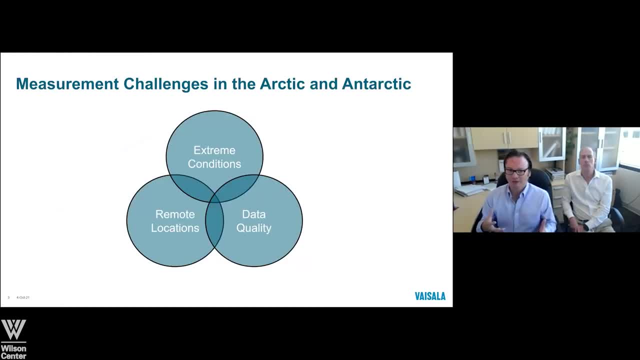 climate. Now, when it comes to measuring things in the Arctic, the Antarctic and the polar regions, there are some challenges, And one is the extreme conditions that are. you know that exist. Yesterday, when the researchers at the South Pole launched their weather balloon, it was negative 65 degrees Celsius. 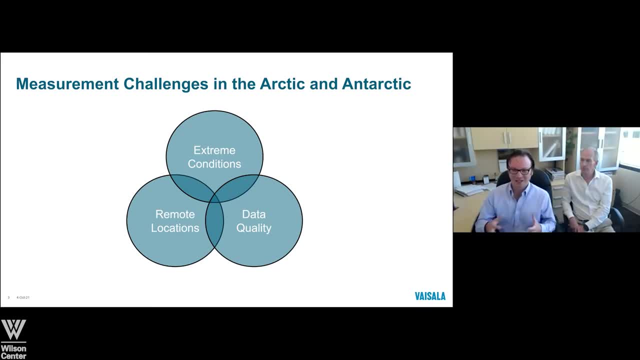 at the surface. So it was much, much colder than it is here in Colorado, there in Fairbanks, in Helsinki, in Geneva. It's also extremely challenging to get to these places, very remote locations, And then you want to have very good data quality, So it's kind of right in the middle there. 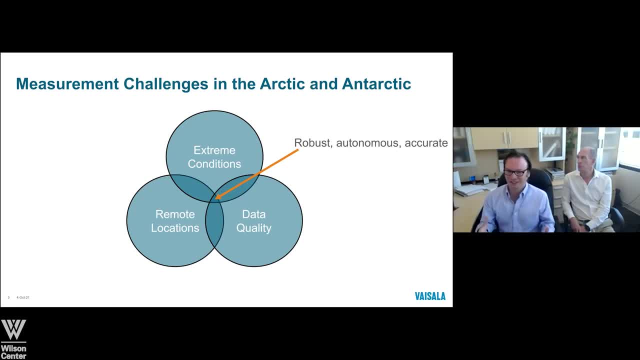 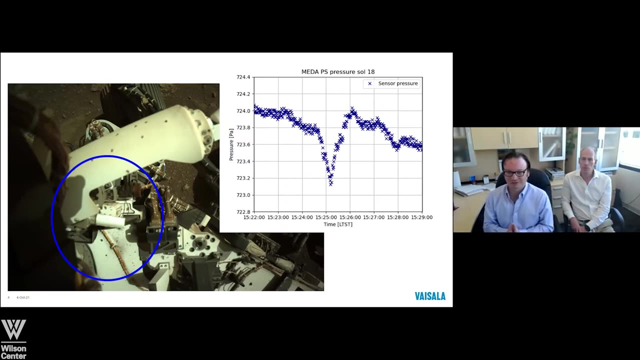 You need something that is robust, potentially autonomous and very, very accurate. We're going to go a few million miles away to talk about this. This is the Mars rover. So this is the Perseverance rover, And we are measuring some of those same essential climate variables that we're measuring here on Earth. 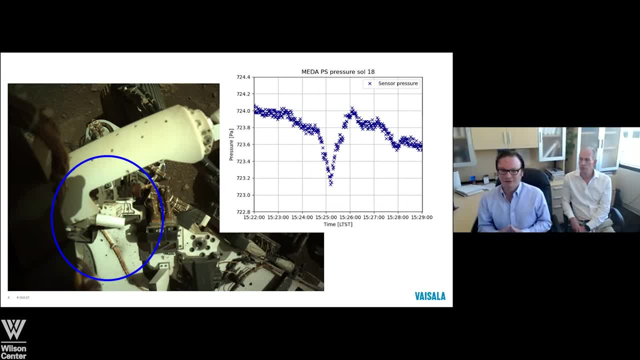 On Mars with some of our technologies. So this is some of the first data that was given back from the Perseverance rover And this is the air pressure on Mars over about a 10 minute period and you can see how the air pressure has changed. 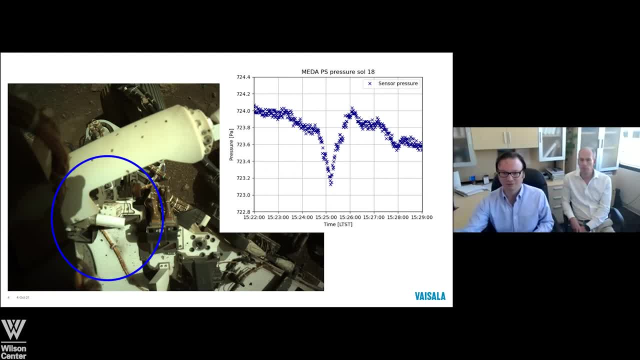 with a little dip in air pressure and then a rise in air pressure over just a very short period of time, potentially as one of the very common dust devils on Mars passed by the rover. So if we can measure very accurately, precisely, and get that information back from another planet, 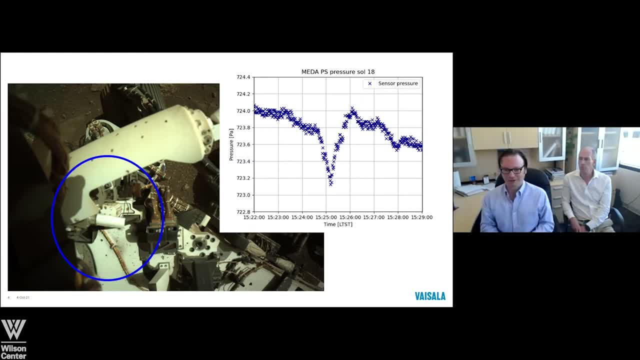 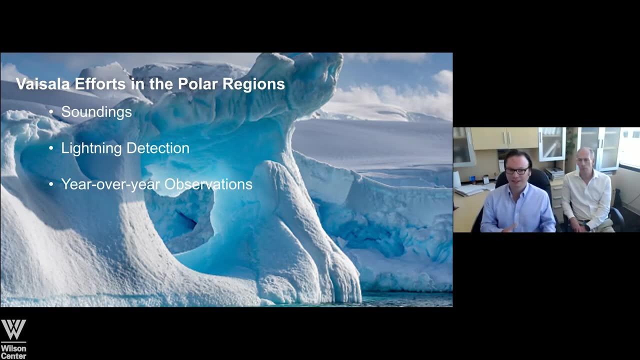 being able to do similar things in the polar regions, where it's very remote, very extreme conditions, should be something that we're able to do as well, And we do do that, do some of that. We're going to talk today about atmospheric soundings, so weather balloons and lightning detection. 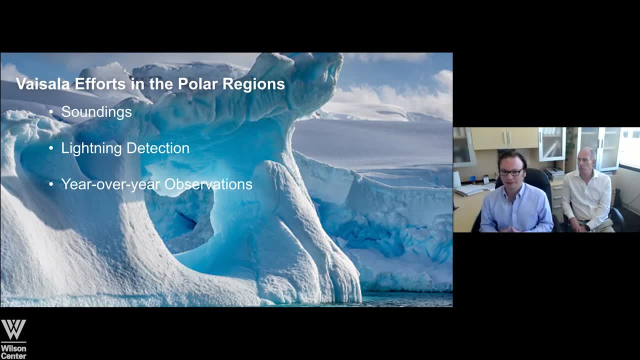 But with that we're going to talk about atmospheric soundings, so weather balloons and lightning detection. But with the technologies that Vicella has we can really measure a wide assortment of these essential climate variables that we've seen on the first slide that we looked at. 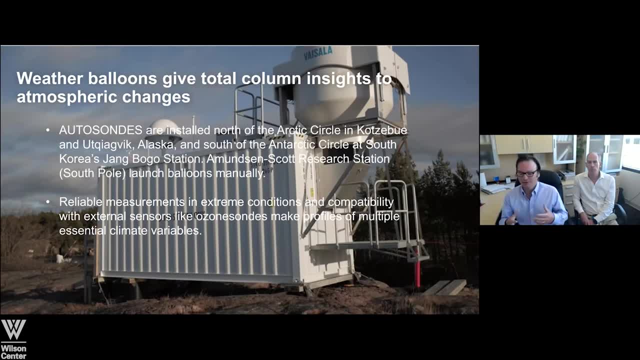 I will talk first about weather balloons. Weather balloons have been launched for over 100 years, Coming up on 110, 120 years. now. Vicella has a At least a dozen of our systems in the Arctic and Antarctic regions. At least a dozen of our systems in the Arctic and Antarctic regions. 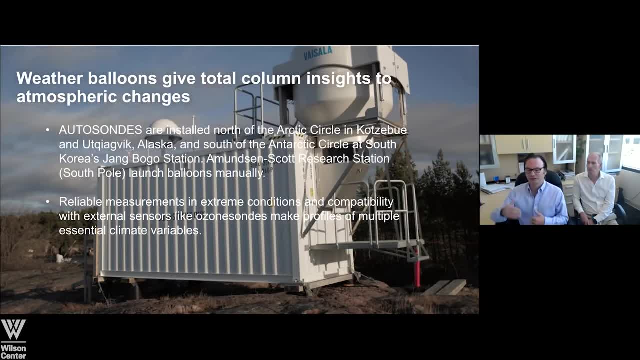 regions that are measuring, from the surface to the stratosphere- temperature, humidity, wind speed, direction, the air pressure, And you can connect these sensors as well to other external sensors, like ozone signs, so that you can get a picture of multiple essential climate variables. 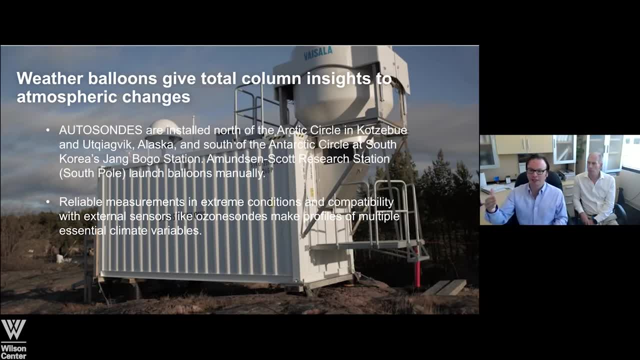 so ozone temperature pressure throughout the entire column of the atmosphere, And some of these are being measured in very extreme locations. As I said, right there at the South Pole we have the weather balloons that are going up daily and temperatures that are negative 65 Celsius or 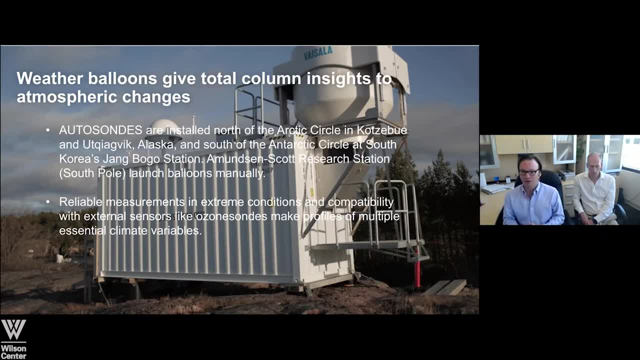 colder in the wintertime. But we've also installed a network of autosigns which are automatic balloon launchers so that you don't have to send people out into the elements across Alaska, including in Fairbanks, Kotzebue, at Utkaivik, And then there's other researchers across the 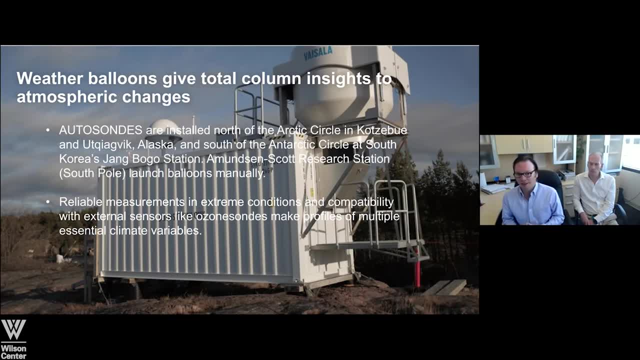 northern South Pole, And we've also installed a network of autosigns which are automatic balloon launchers, so that you don't have to send people out into the elements across Alaska, including in stretches of the world and the southern stretches that are using these sensors to get a better 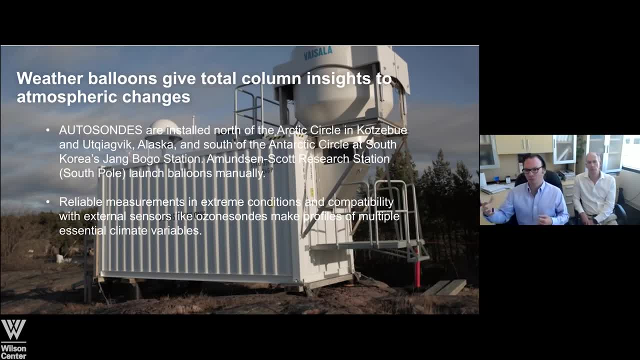 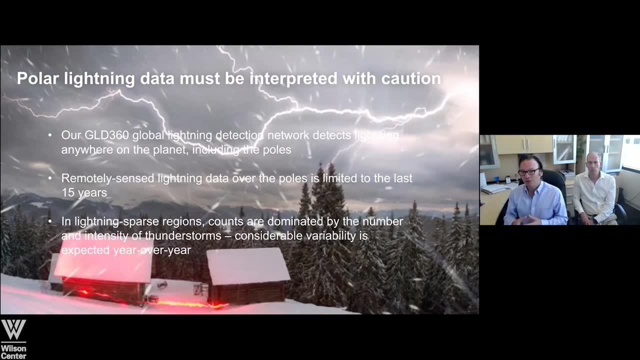 picture of how temperatures and how winds are changing at all levels of the atmosphere over time. Now polar lightning data. it needs to be interpreted with caution And there's been a lot of talk about increasing lightning over the Arctic, But when you think about it, we've only 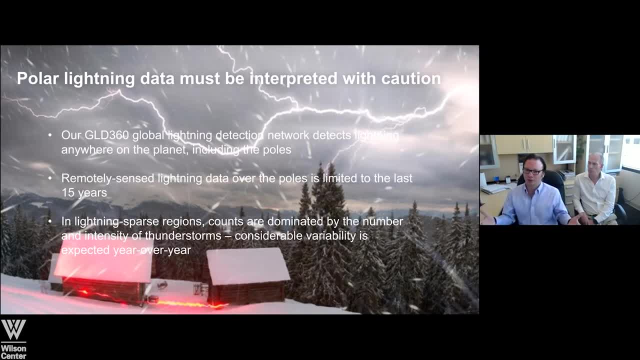 talked about increasing lightning over the Arctic for about 15 years, And that doesn't give us a long period of time, a long period of record, to do data interpretation In lightning sparse regions like the Arctic and the Antarctic. the number of lightning events detected is going to be dominated. 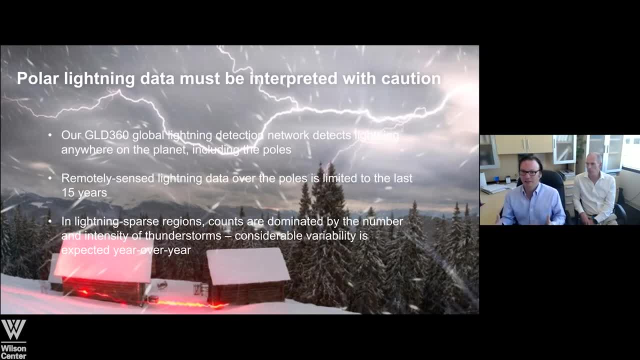 by the number of thunderstorms and how intense they are. And if you have a very lightning sparse region, if you have one or two storms in one year and not the next, your numbers are going to fluctuate wildly. And so if you have a very lightning sparse region, if you have one or two, 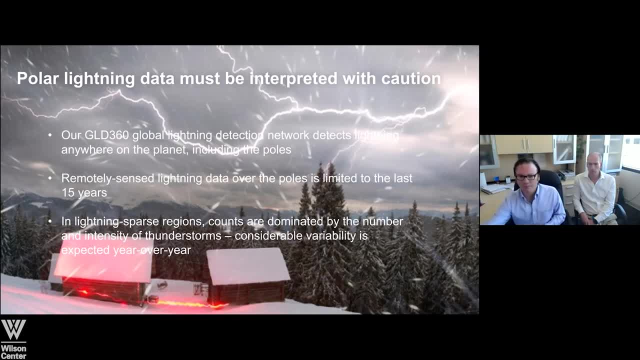 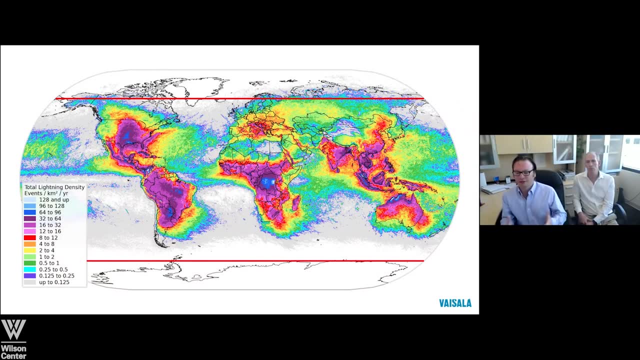 storms in one year and not the next. your numbers are going to fluctuate wildly And we'll see that in the coming slides. So our lightning detection network. we have a global lightning detection network that detects lightning 360 degrees around the world, from pole to pole. I've noted the Arctic. 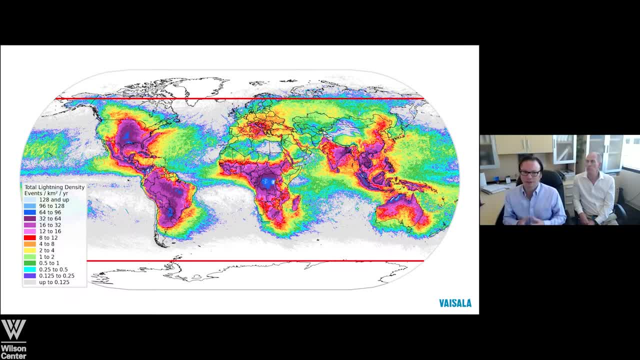 and Antarctic circles here in red. So you can see that these really are very sparse regions for thunderstorm activity when you compare it to the Great Plains of the United States or Central Africa, Southeast Asia, Northern Australia, Which are some of the more commonly known lightning hotspots. But, as the Secretary-General, 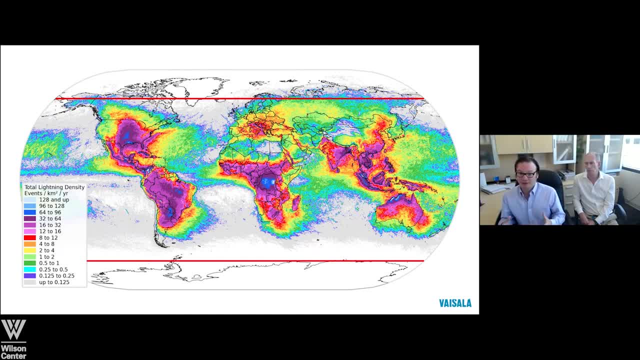 has shown, wildfires in the Arctic is going to be a big contributor to greenhouse gas emissions And with lightning in those regions they can actually trigger more wildfires, which can trigger more greenhouse gas emission releases. So monitoring and having an effective network of lightning detection sensors to monitor changes in thunderstorm activity and lightning activity. 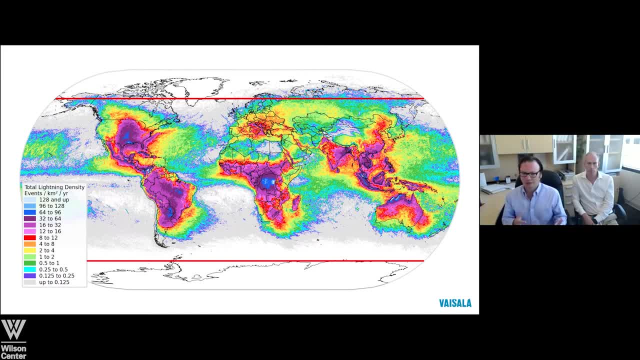 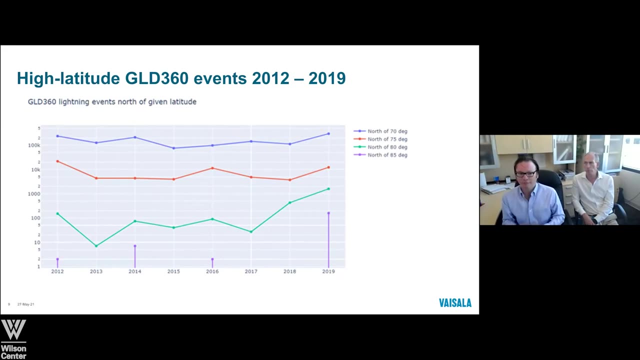 in these polar regions is an especially critical data source for helping to monitor climate change in these regions, And we'll look at the last seven years. I haven't put in the 2020 data here yet, But this is lightning that we've detected north of given latitude bands. 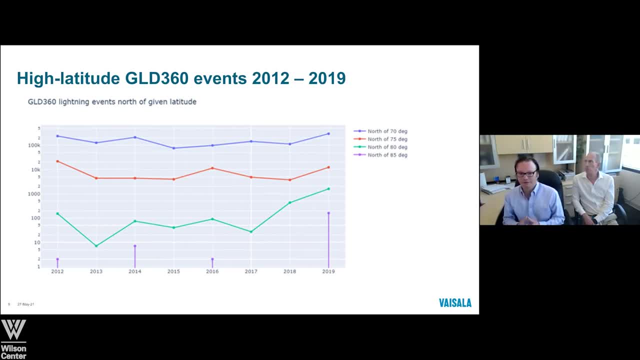 So at the At the top, there in the blue is north of 70 degrees and then down to north of 85 degrees And you can see, at the north of 70,, north of 75, there's been not much of a real increase or decrease. 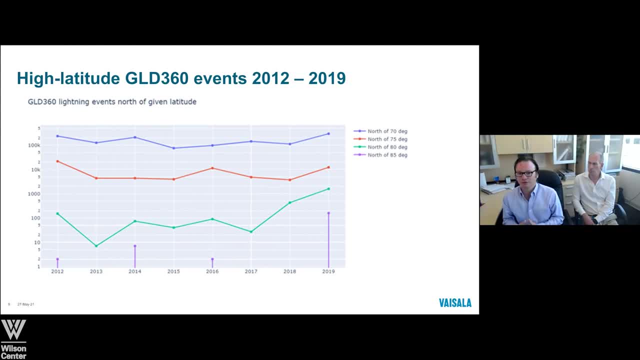 in lightning north of those regions between 2012 and 2019.. Whereas you can see more substantial increase north of 80 degrees And north of 85 degrees, where lightning is extremely rare. you can see that fluctuation from the east to the west. So you can see that fluctuation from the east to the west. 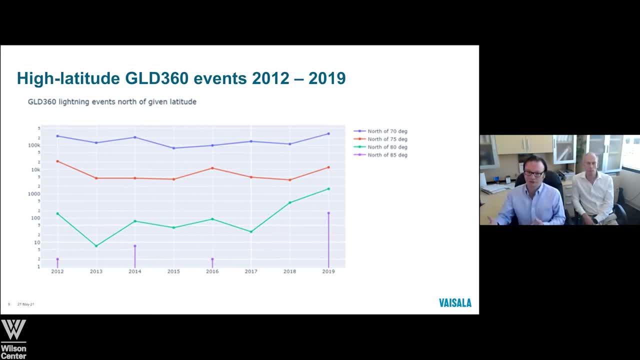 So you can see that fluctuation from year to year, whether there is a thunderstorm or two thunderstorms. In 2019, we detected more lightning that year north of 85 degrees than in any of the previous years, And then in 2020, we actually detected even more lightning north of 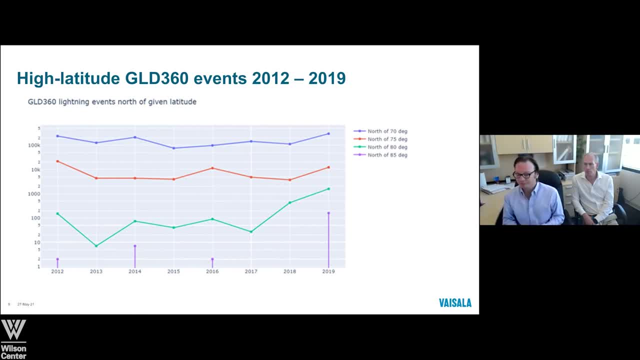 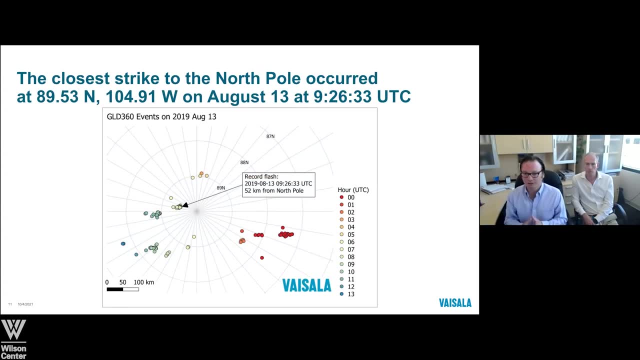 85 degrees north than in even 2019.. What really kind of got our attention in 2019 was that frequency of lightning north of 80 and then north of 85. And the National Weather Service in Fairbanks, Alaska, had actually noted a substantial thunderstorm north of the Arctic Circle. 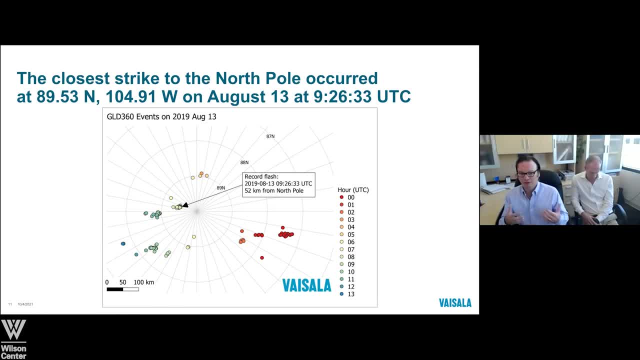 north of Alaska And we started looking more and more into lightning in these high-latitude regions And we actually detected August 13th of 2019, the furthest north lightning detection on record. It was just 52.8 degrees. 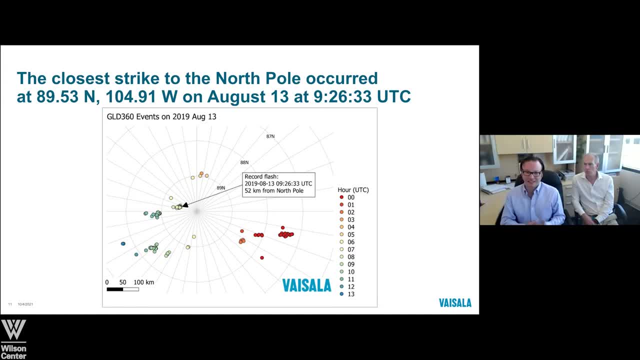 was 52 kilometers from the North Pole. It was actually about 5,500 miles due north of where I'm sitting right now, or 5,500 kilometers due north of where I'm sitting right now. So we had multiple thunderstorms on August 13th that developed south of the North Pole and then 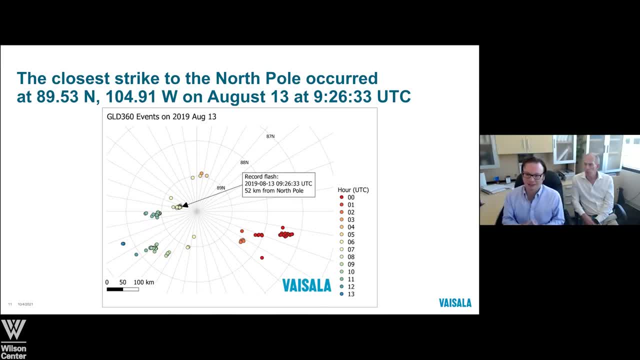 moved north over the pole and then back south, So very uncommon phenomenon here to have this cloud-to-ice lightning that we were detecting this far north And, as I said, last year we actually detected even more lightning than in 2019.. Some of the preliminary numbers that I've 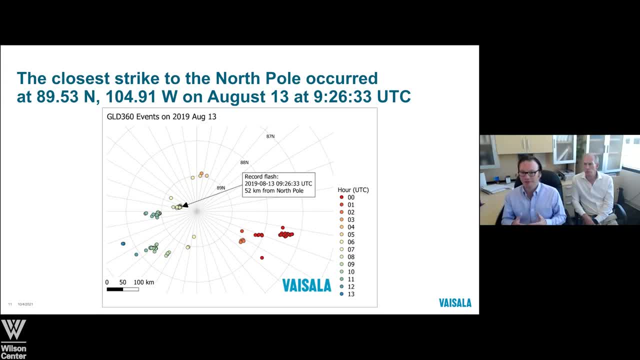 looked at for north of 70 degrees, is that we may have detected even more this year than in the previous two years. So, all of this data that we're collecting, whether it's through lightning detection, through weather balloons or even through automatic weather stations, many of the 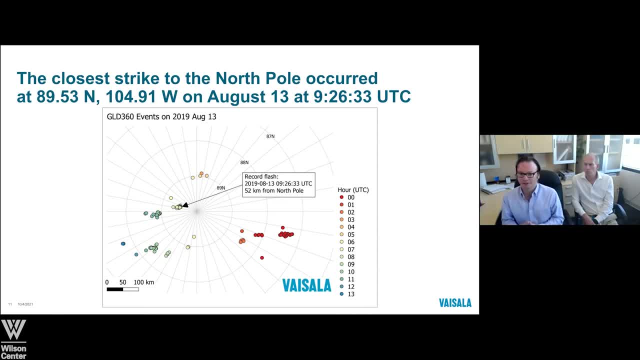 other technologies that we're collecting, we're able to detect even more lightning than in 2019.. Technologies that we've developed here at Vaisala will be especially important for the atmospheric and other climate researchers. We're trying to understand exactly how climate change. 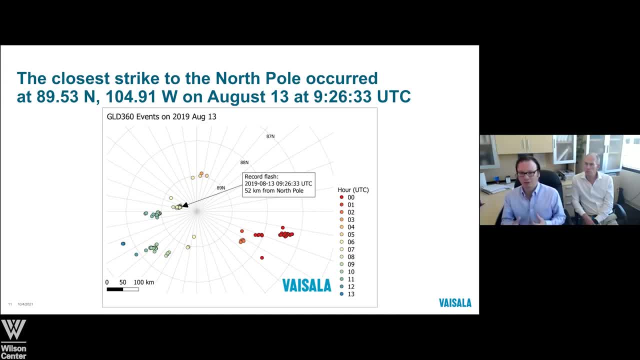 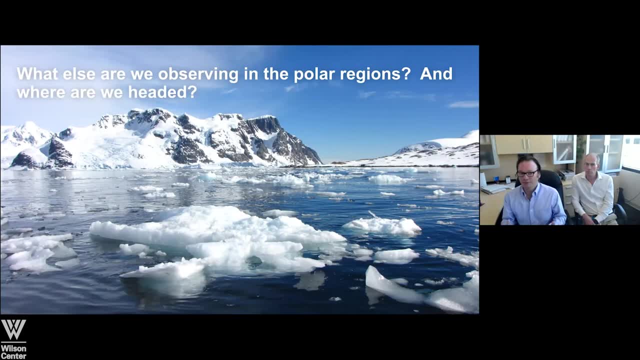 is impacting these very remote, extreme places on our planet, in polar regions. So where are we going to be headed next? Well, I mean, we're just going to be following the data. We're truly believing in better measurements leading to a better world. 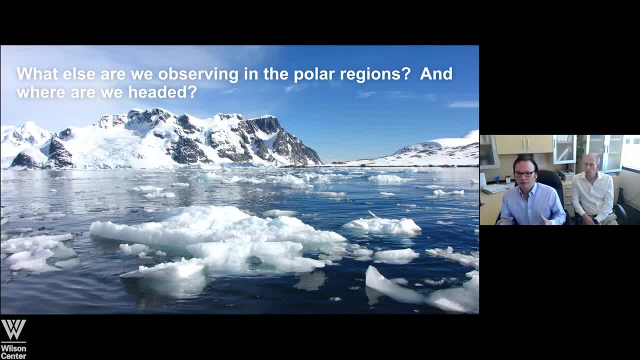 So we are going to continue to keep our curiosity, look to see what other technologies we can develop and modify to help us better understand some of these essential climate variables that we maybe aren't measuring yet. or the ones that we are measuring, How do we take that data to? 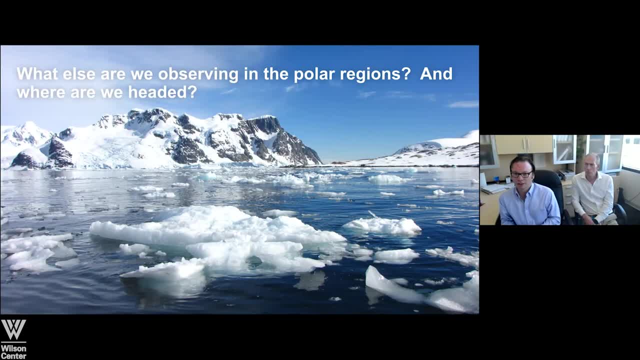 the next step: turn that into actionable information for the policymakers, for the researchers, and see what we can do to help mitigate some of the effects of climate change. So again, I wanted to thank you for taking the time to listen in today, for inviting us to talk. 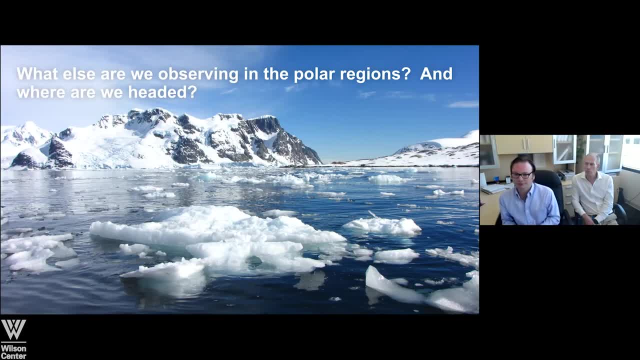 about some of what we do And we'll be happy to take any questions. Well, thank you very much, Boy. do I have a number of them? But TJ, any comments? before I make a few comments and then move on to our colleague Evan Bloom? Well, first off, I'm very glad I brought 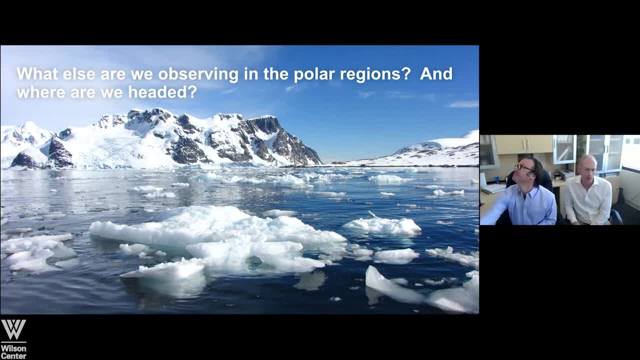 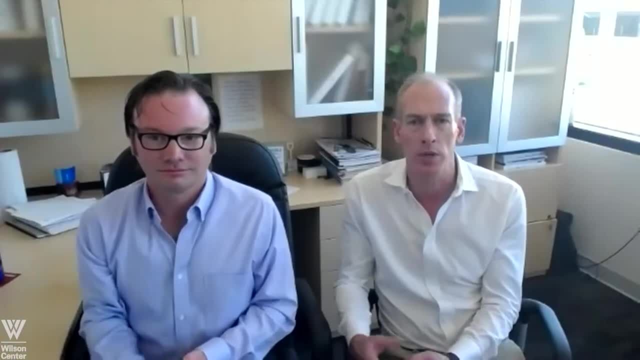 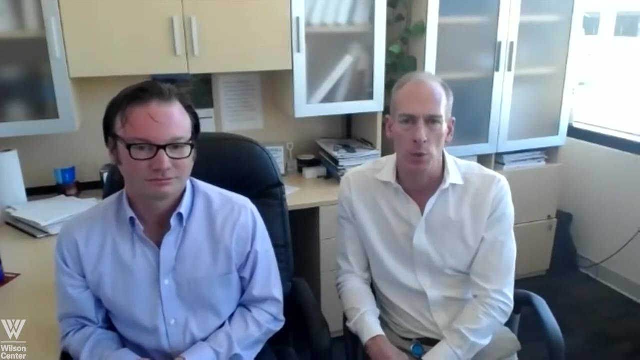 my colleague here. But besides that, yeah, it's very motivating for us at Vaisala to be on the front lines of providing the equipment and the data that groups like the WMO and groups all over the country here in the US and around the world can use, And it's something that we take very 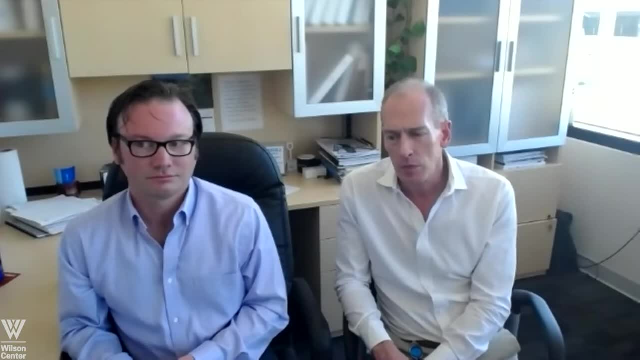 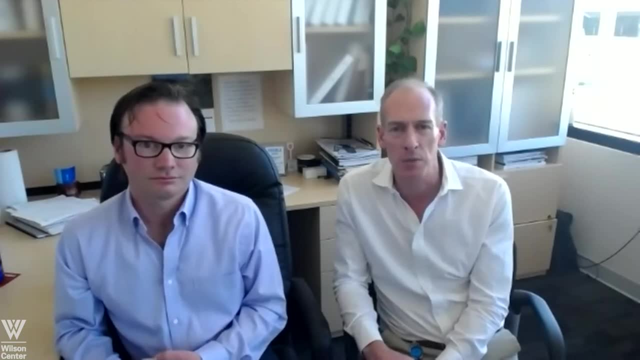 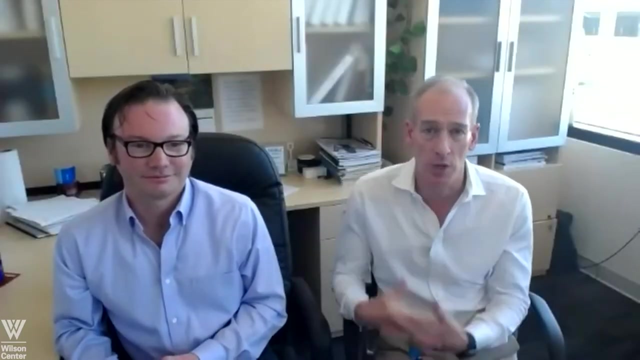 seriously and we're very motivated to do so And, again, we're very proud to represent Finland. I think we were what Hallie was referring to as the honorary Finns on the call, I believe. But you know, Finland is really on the front lines and doing a lot of work in this area And 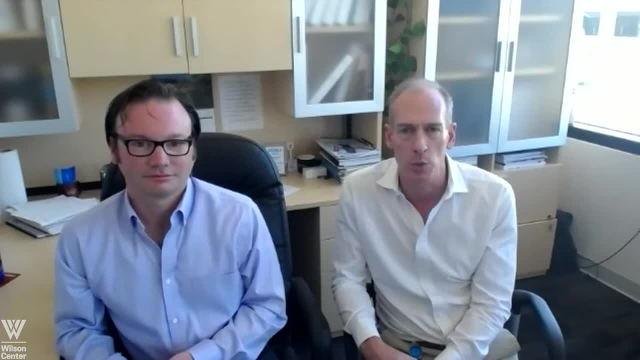 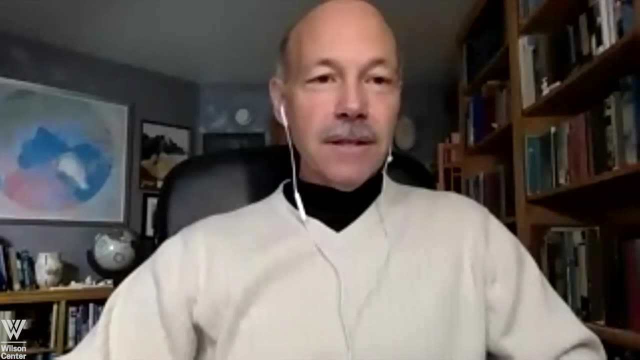 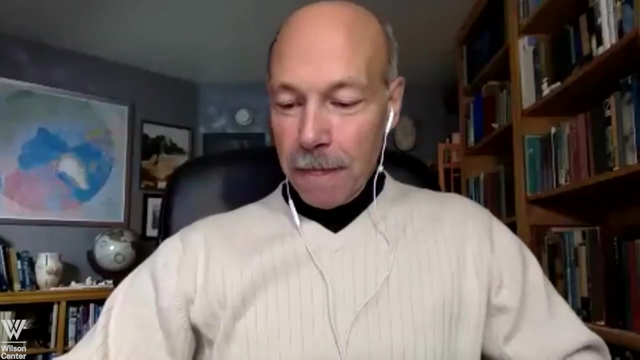 it's just an honor to be carrying that banner here in the US and around the world. Well, thank you both very much. The issue of lightning strikes near, on or near the North Pole is just absolutely frightening for a number of situations and a number of perspectives. But 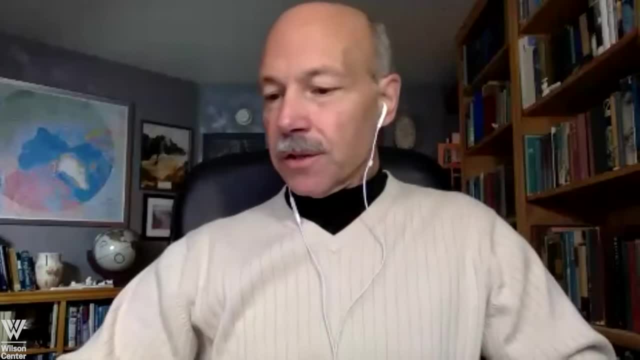 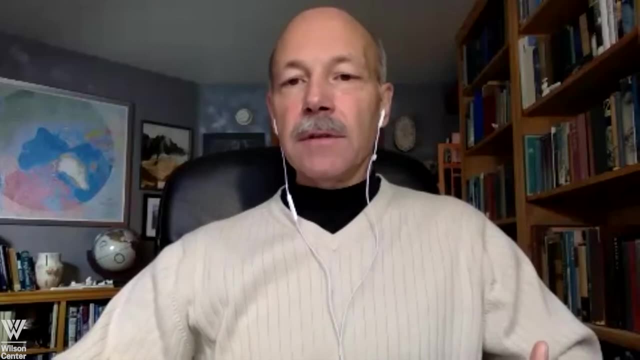 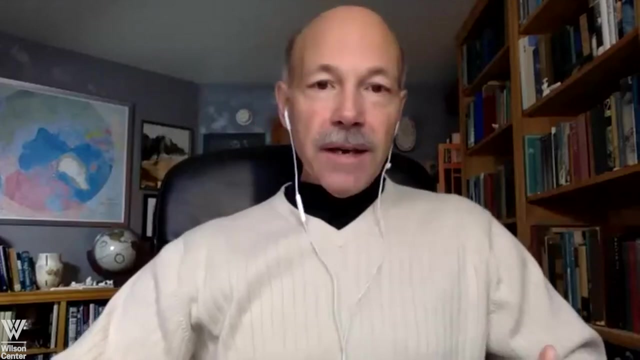 we'll come back to that, And I may even ask the Secretary General for his thoughts about this whole idea about observing networks. How much capacity do we collectively have in the Arctic? Where are the gaps? How does the international community fill the gaps in? 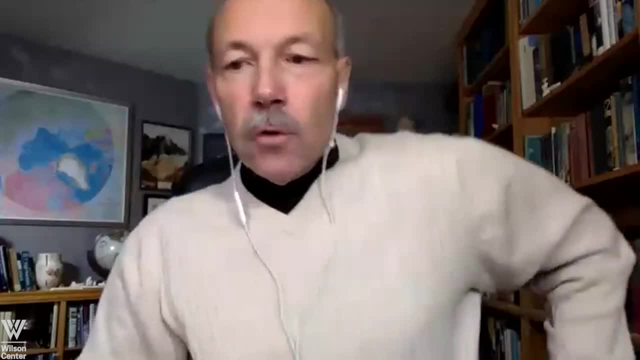 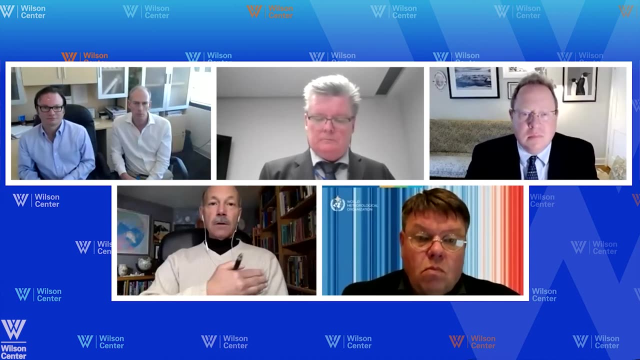 monitoring and observing so that we can make better, more informed decisions, not just about our research assets, but also how those assets are funded and how they may come about in terms of informing, good, solid policy. And so maybe, Mr Secretary, once Evan is done, I can put you on the spot, if you don't mind. 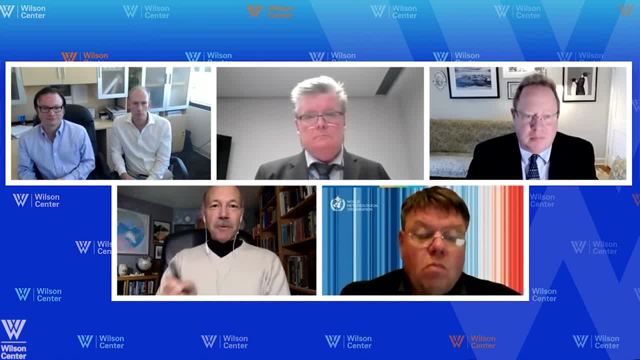 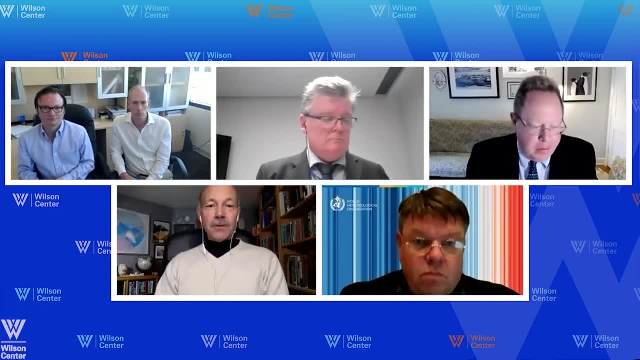 sir, and ask you about that connection between what we just heard and where the WMO is going as well, if you don't mind, But I'll reserve that until Evan is done. But thank you so much And thank you to our colleagues there at the CISO. Next is our good friend and colleague Evan Bloom. 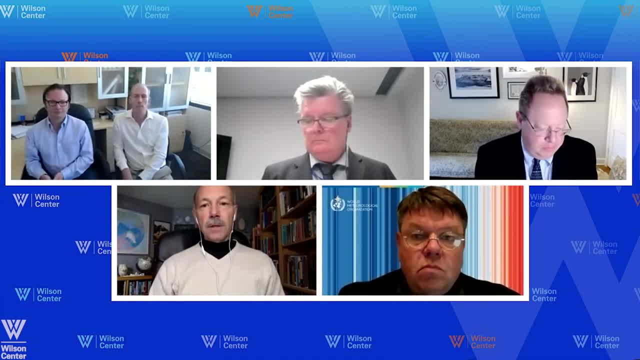 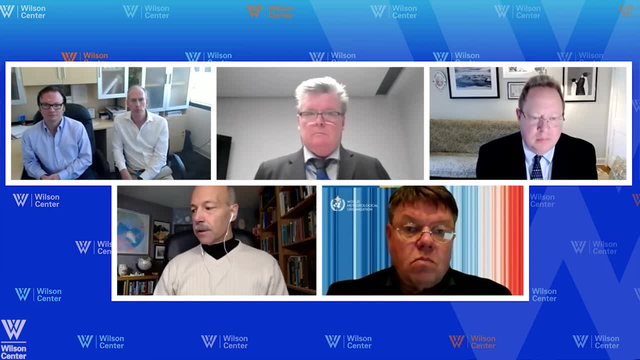 As many of you know, Evan served as the former Acting Deputy Assistant Secretary for Oceans and Fisheries. I will note that Evan had both portfolios of the US and the US and the US portfolio for the Arctic and the Antarctic region, which is why I find his participation today. 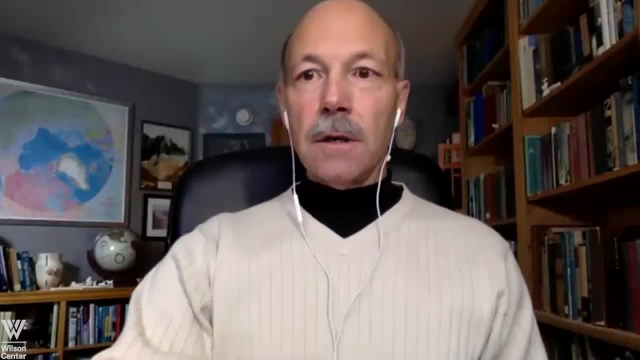 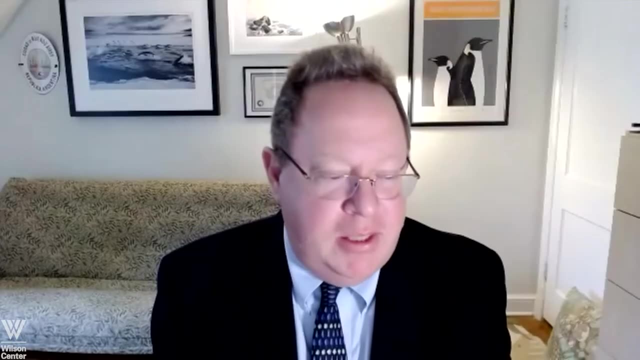 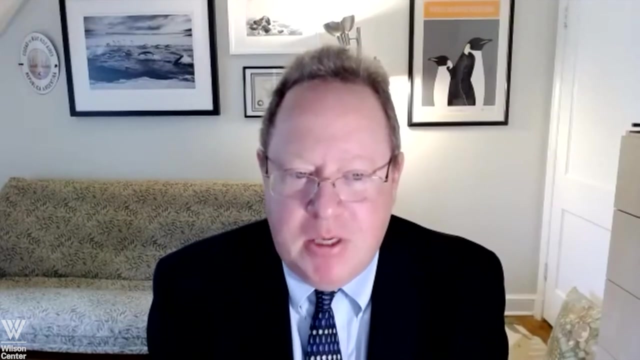 important, but also seek his guidance, often on issues within the Polar Institute. So, Evan, let me turn over the floor to you. Mike, thank you very much indeed, And I'm very pleased to be part of this panel with very distinguished experts and officials, So I thought I'd add some additional. 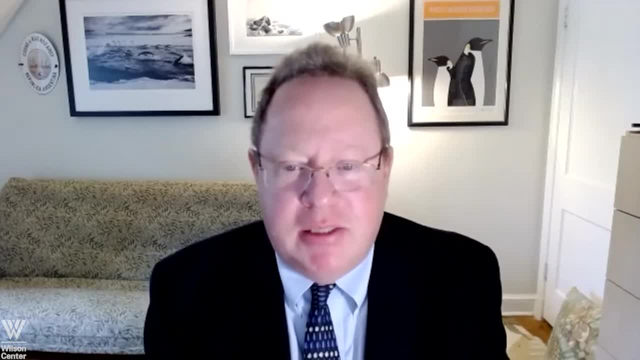 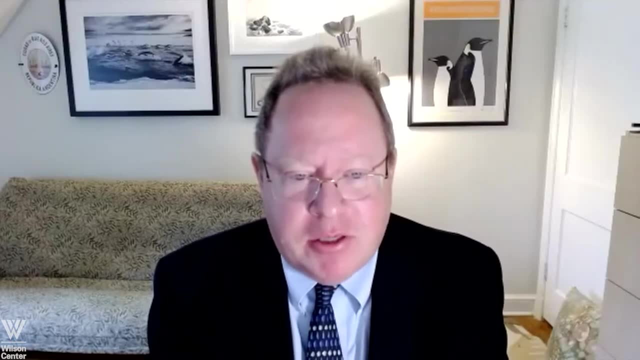 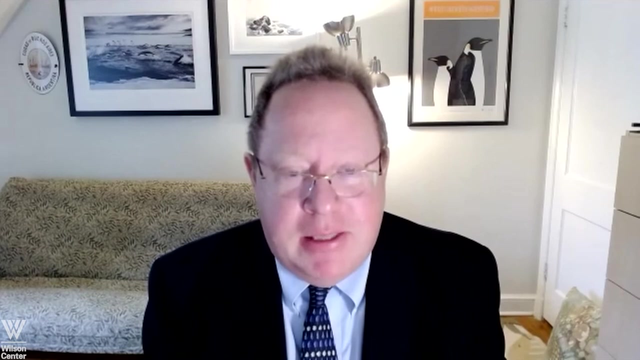 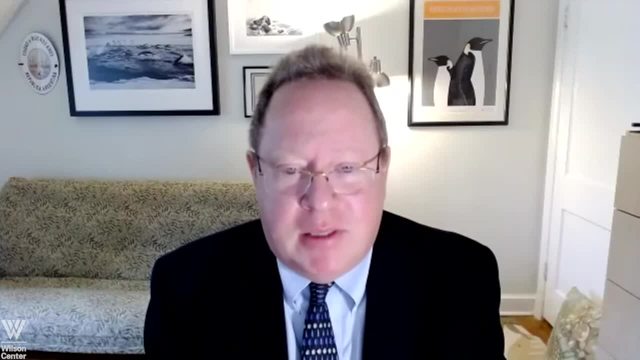 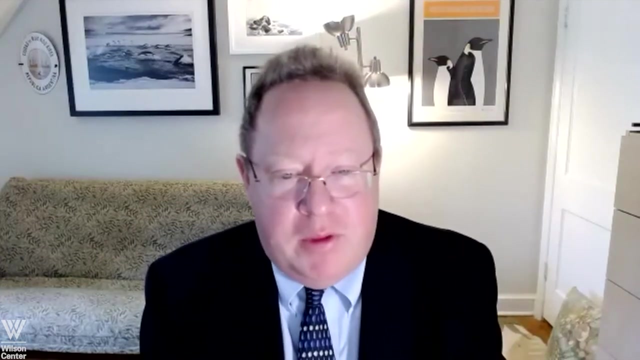 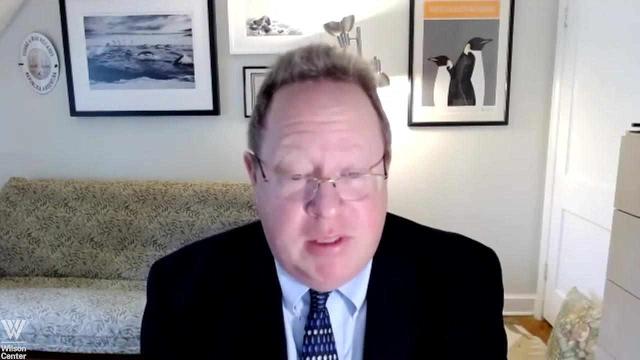 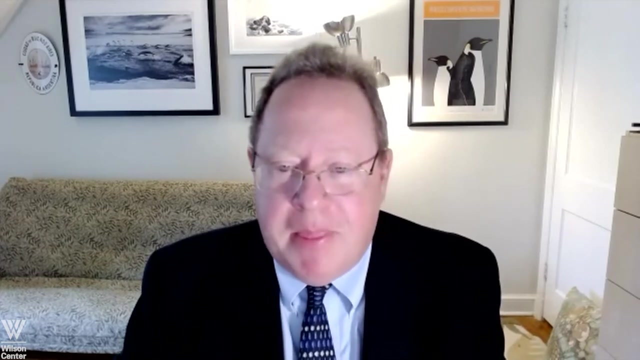 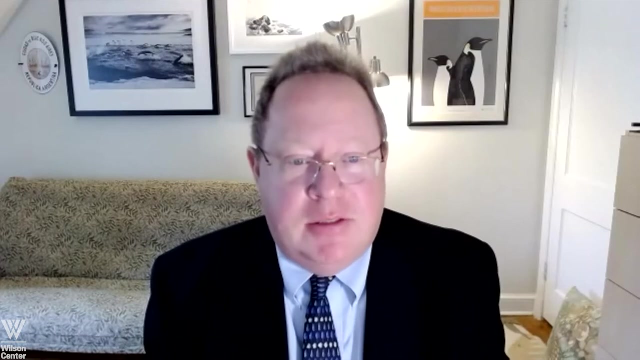 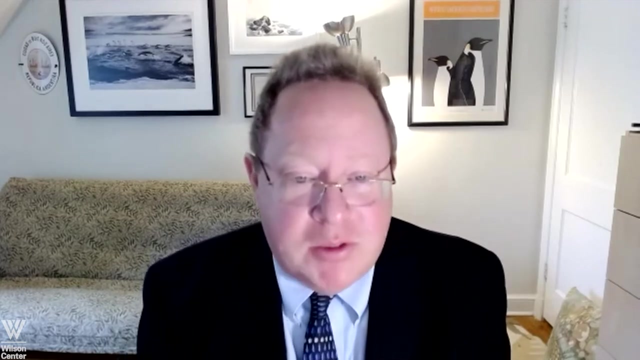 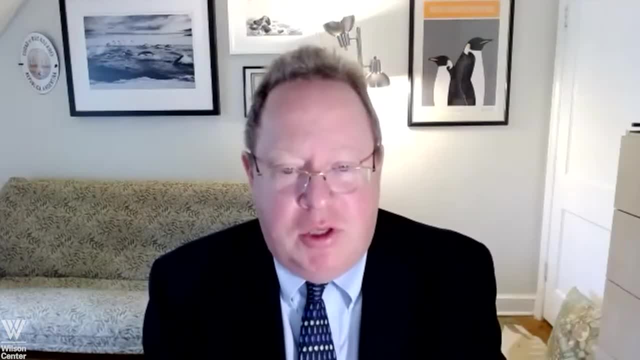 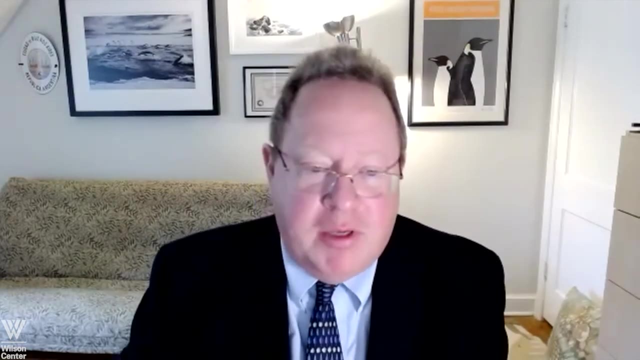 And with the advent of the Biden administration, the US is now able to rejoin efforts within the Arctic Council that address climate issues and connections to the Arctic. The Arctic Council is a good forum for some of these discussions because of the presence of the permanent participants, the indigenous groups that sit at the table along with the states. 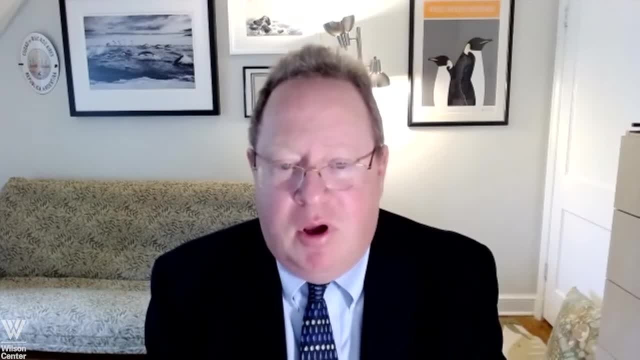 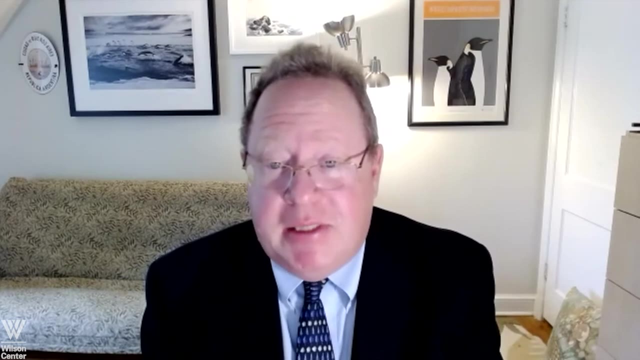 They can bring indigenous perspectives on climate issues in the Arctic, so both indigenous knowledge and scientific knowledge are both taken into account. Arctic science, Arctic science- Arctic science is important for all the Arctic states, as is science-based decision-making for Arctic governance. The Council has given rise, as was mentioned, to three legally binding agreements among the eight Arctic states, and one of these promotes Arctic science by attempting to lower the barriers to scientists seeking to work within the various territories of the Arctic. 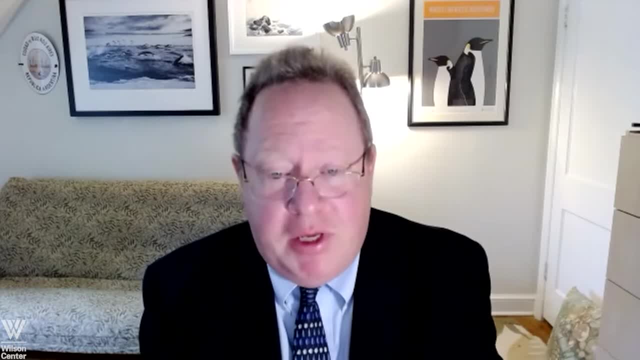 The Council has a series of working groups, as I already mentioned, that focus on Arctic science by attempting to lower the barriers to scientists seeking to work within the various territories of the Arctic. The Council has a series of working groups, as I already mentioned, that focus on 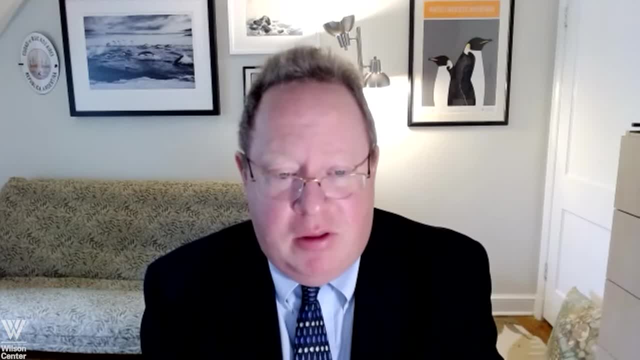 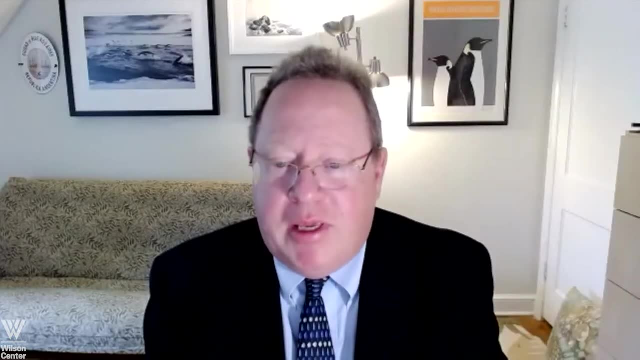 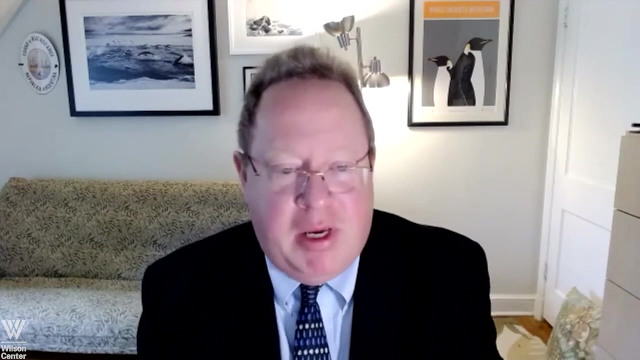 technical issues with government, scientists and other experts. So also those who follow the Council's work will know about the groundbreaking Arctic Climate Impact Assessment from 2004.. It was the first comprehensive, multidisciplinary assessment of the impacts of climate change in the Arctic and was designed to provide input to policymakers as well as to the IPCC. 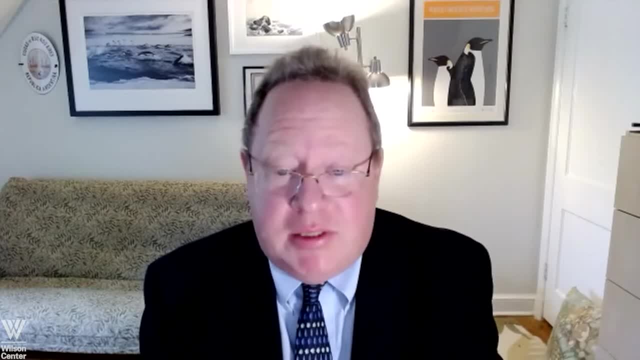 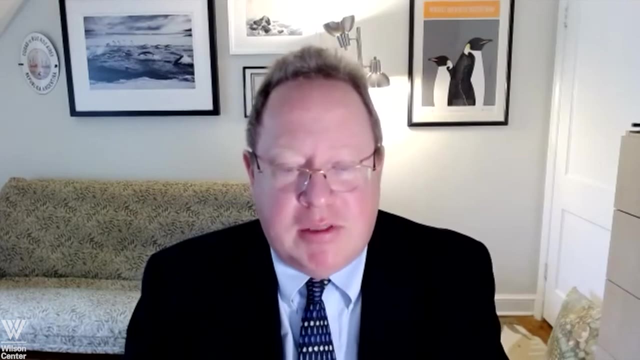 Now this initiative seems like a walk in the park. Now, this initiative seems like a walk in the park. It was a while ago now, as does some of the work done under the UN Framework Convention on Climate Change some years ago, but all of this provided a foundation for the immense, very sophisticated efforts that are now going on to address the climate crisis. 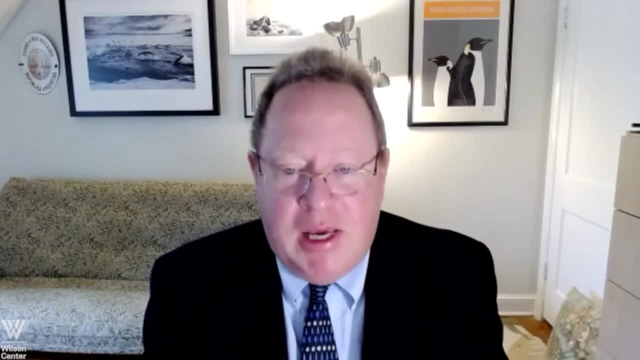 So there's a keen connection among Arctic science, the work of the Arctic Council on climate issues and the issues to be grappled with slowly at the at climate level. Now another Things to Report from theprising conservation and development Corner Cultures. 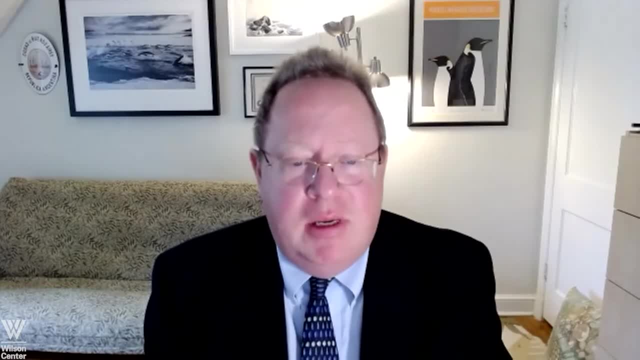 You all know that one of the most significant goals on this final agenda was to ensure hundreds and hundreds of millions of builds and infrastructures in the region. And then the other hon Columbation of lessons was powered by the community policy work that was done for COVID-19.. 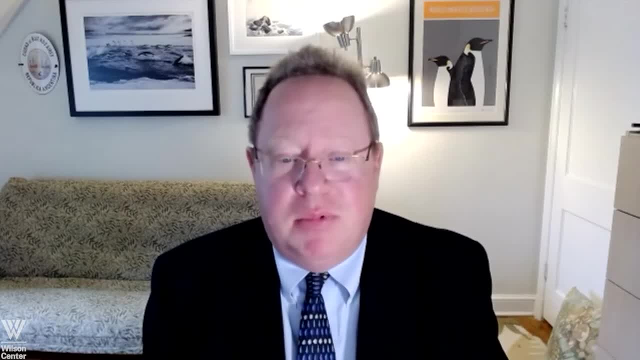 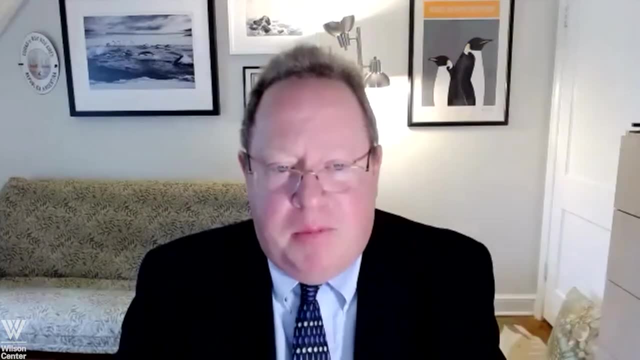 So let me just take you for a few minutes and then turn us back over to David. Thank you, David. Yeah, Bob, if you'd like, Sure, Thank you. tensions that exist on other issues. The pandemic has reduced international scientific efforts in. 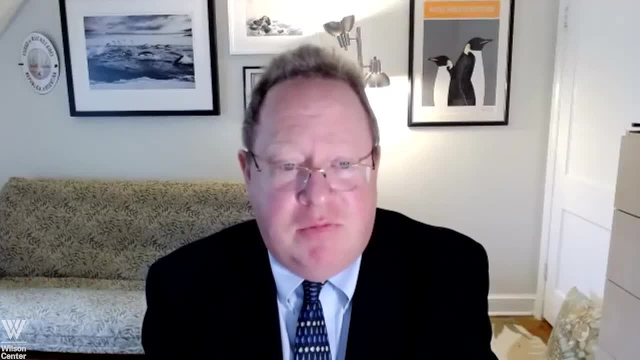 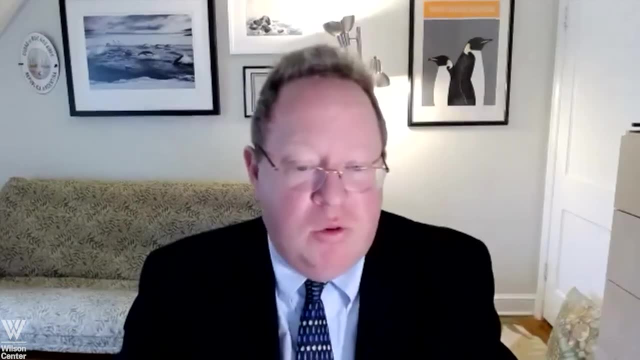 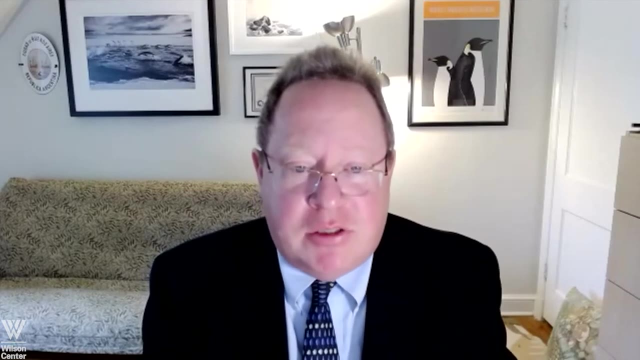 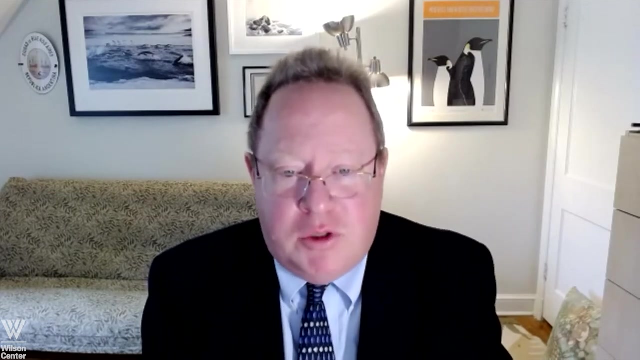 the Arctic by a certain amount, as scientists have not been able to cross borders, in particular. As the pandemic recedes, hopefully things will get back to normal and the science cooperation agreement and other tools can be used to increase international collaborations throughout the Arctic. I'm glad that Ambassador Vorimaki referred to the efforts of 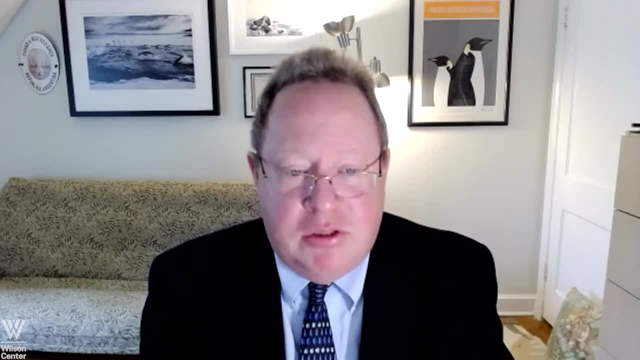 uArctic, It and a host of educational institutions are critical to efforts to study Arctic environmental change and a host of related topics, And I'm also very pleased that the Ambassador mentioned that he moves to the Antarctic Treaty when he gets a glazed look at the Arctic, And I'm also very pleased that he moves to the Antarctic Treaty. 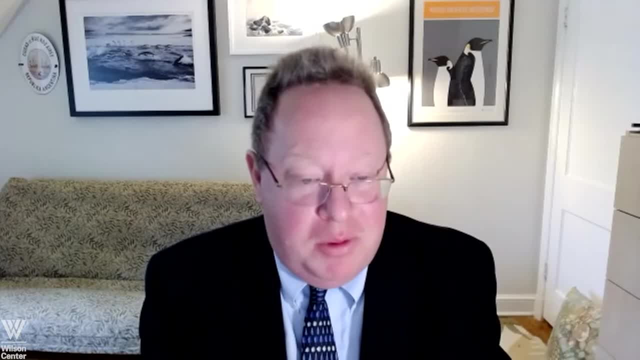 when he gets a glazed look at the Arctic, And I'm also very pleased that the Ambassador mentioned the Arctic Council, So I'll mention Antarctic issues for a moment. This panel is, of course, about climate science at both poles. at least that was the title, and it's worth reminding ourselves. 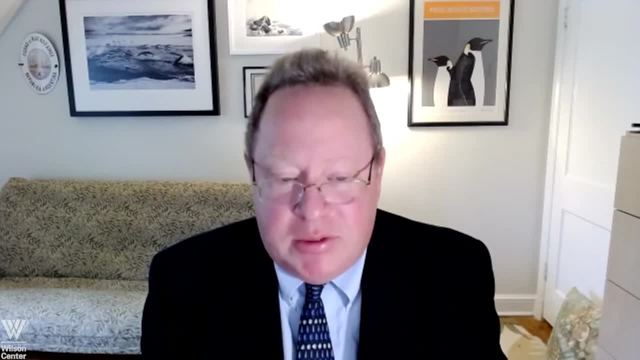 of the importance of science going on in the South as well as in the North. Indeed, both Finland and the US are leaders when it comes to Antarctic governance and to science at both poles, So work is going on in antarctica that is crucial to understanding the climate system and certainly 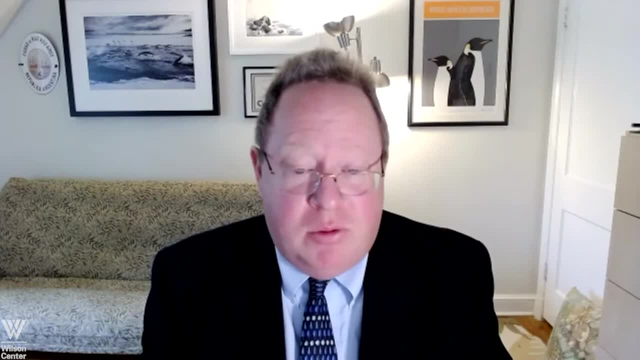 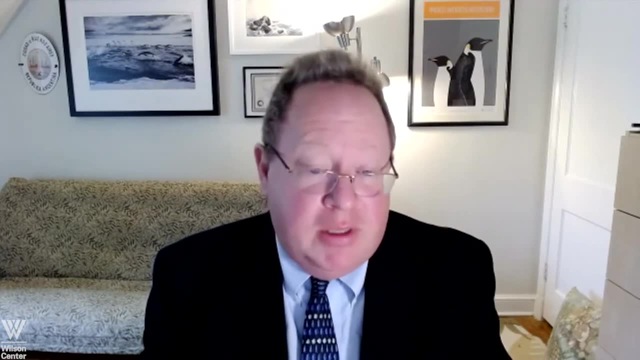 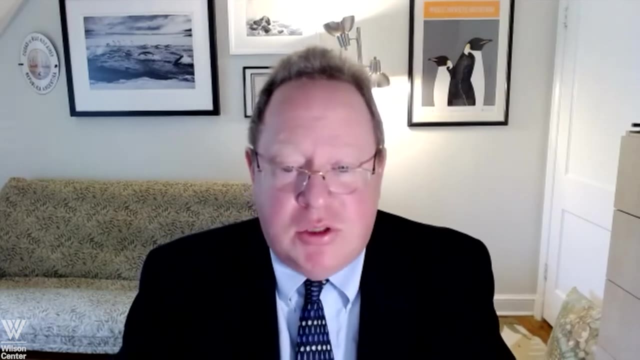 studies of glaciology tell us much about issues of sea level rise um the glaciology in antarctica, in the same way that studies in greenland provide critical information and a necessary warning for our societies. so, mike, i think i will stop there and turn it back to you. thank you, mr ambassador. 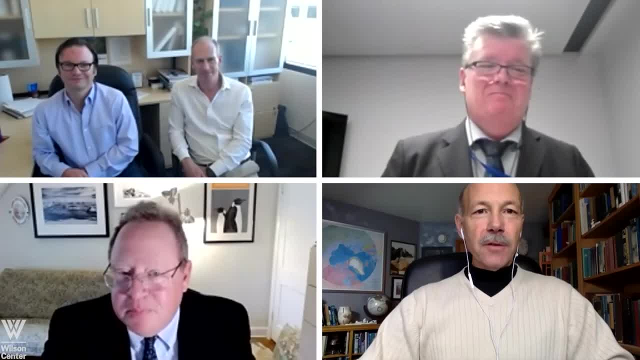 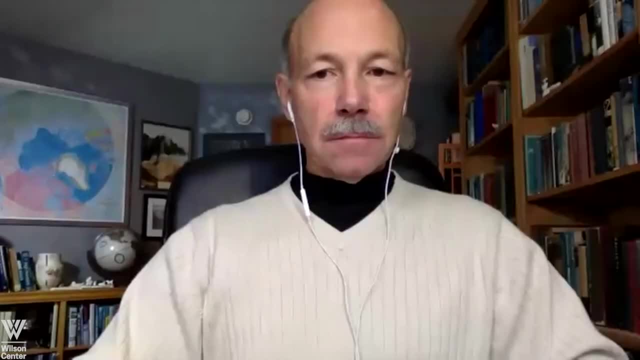 i saw your, your, your, hand up. do you want to follow up briefly before i move on to the questions? yeah, if, if i may just say that i very much um appreciated um evan's insightful analysis. just just few quick uh comments just to add that the the anthropology strategy that that we released. 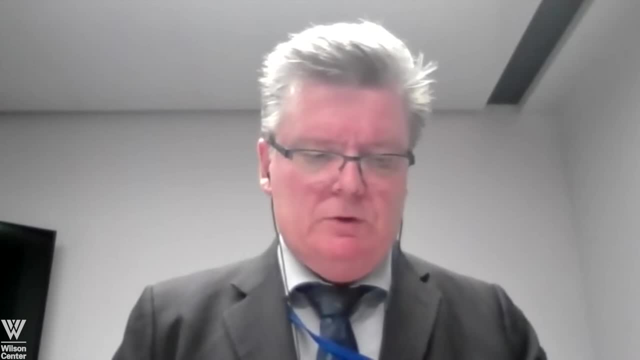 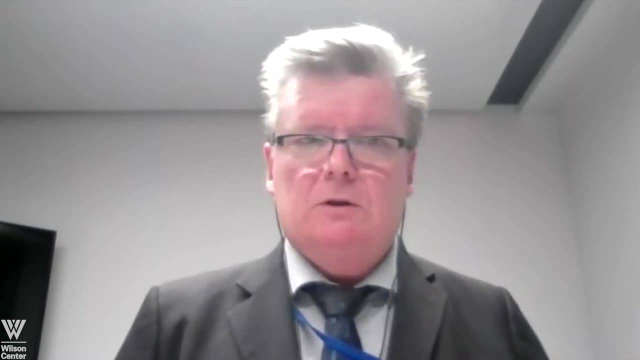 um, it was a process led by our prime minister's office. it was a truly collaborative uh exercise with all the ministries. the international context is overarches all the priorities. i mean that was a conscious choice that we did um, the thought being that nothing, we, we can't do anything in isolation or in a vacuum- everything. 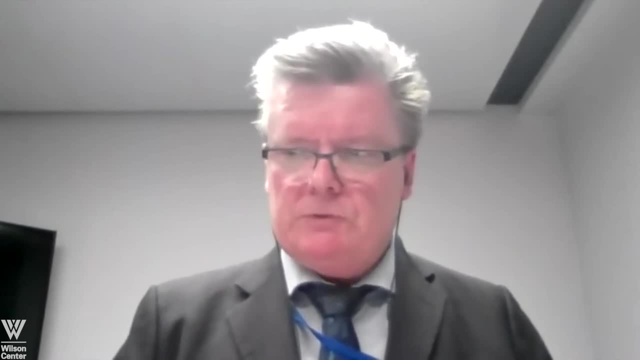 we do in the context of international cooperation. the strategy very much underlines the role of the arctic council and of the eight arctic states, but does open the and acknowledges that that wider cooperation, for example in science uh is, is needed um one of the novelties of the 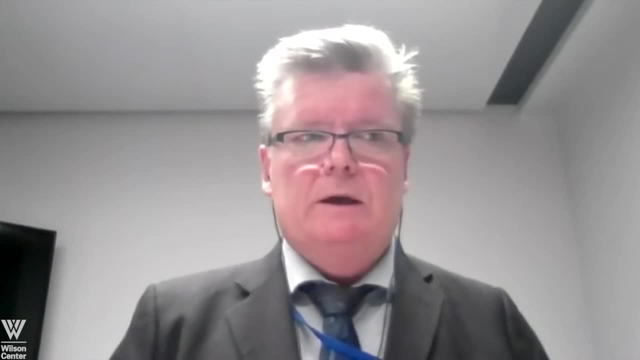 strategy was um that there was, for the first time ever, a brief section on the antarctic. as you may have noticed, and as my country's first ambassador, that covers both the arctic and the antarctic. um i i i find it um um strong position by finland to be one of the only five countries in the world who are both members of the arctic council and the antarctic treaty? um, there are the. the others are the united states, russian federation, norway and uh and sweden, and i look very much forward to welcoming the antarctic treaty consultative meeting to helsinki. 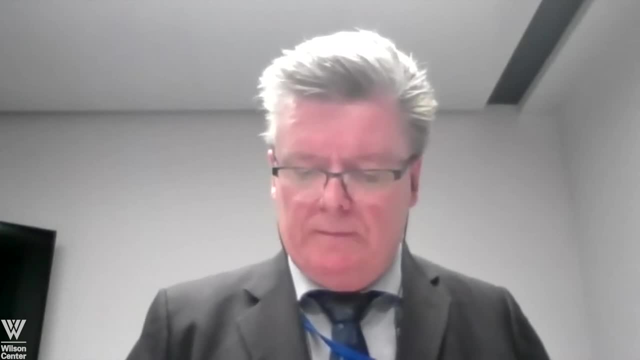 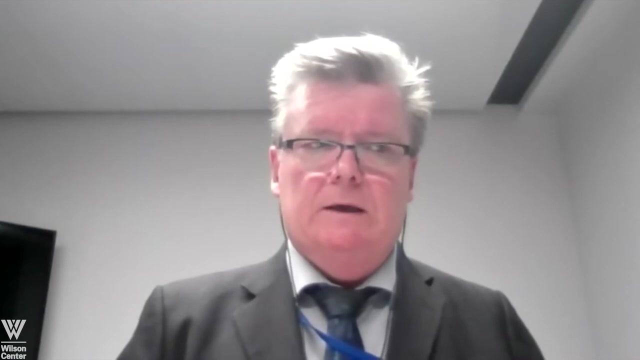 in the spring of 2023 and on the arctic council. environment, climate change- yes, absolutely, but there are also new challenges facing the the council from various directions and we just need to ensure that the council is ready to face these challenges. thanks a lot and thank you again, evan. 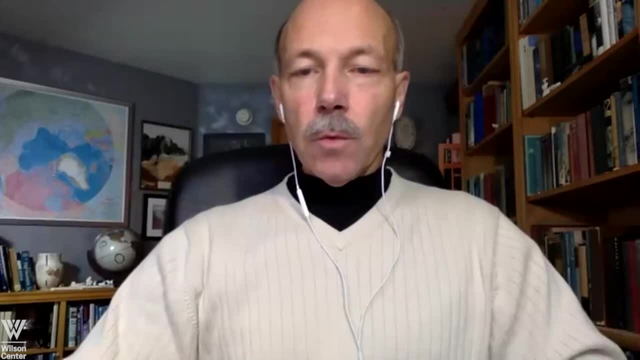 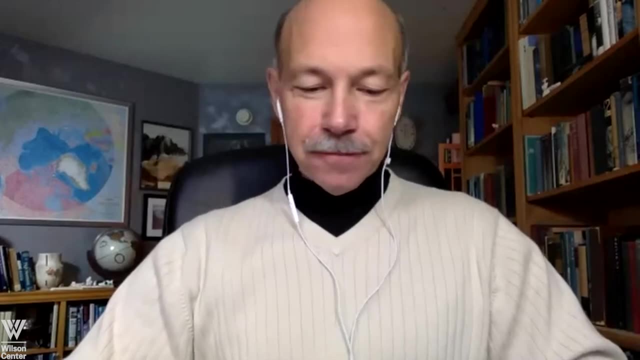 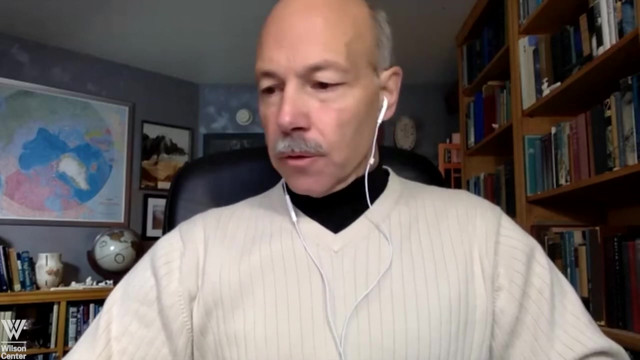 thank you, just for our colleagues in the audience. just remind you one more time: you can email us at poler, wilsoncenterorg with your questions or comments. but i'd like to come back, mr secretary general, to uh, to the questions i wanted to ask you, in no particular order, but to start with our. 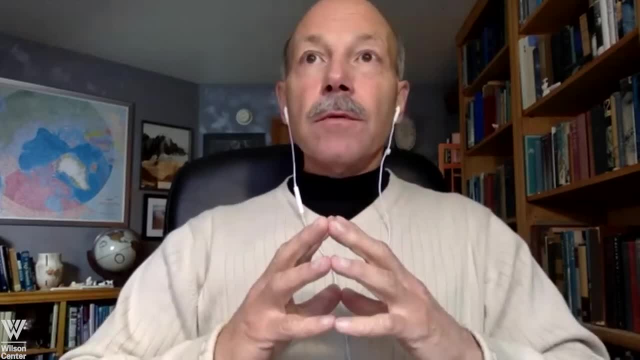 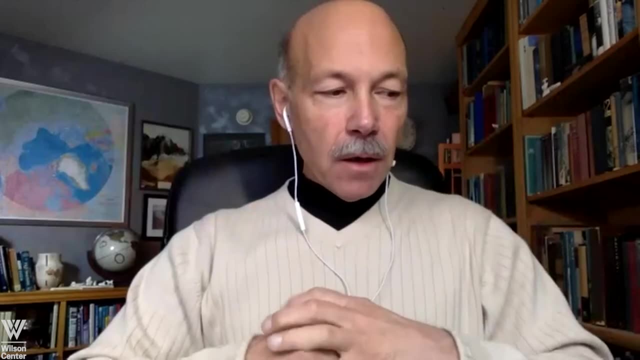 friends from uh visla, uh, the arctic. it's a huge area to cover, right like like many other places on the planet, but from your perspective, what do you think about the arctic? and what do you think about the arctic? and what do you think about the arctic, but from your perspective? 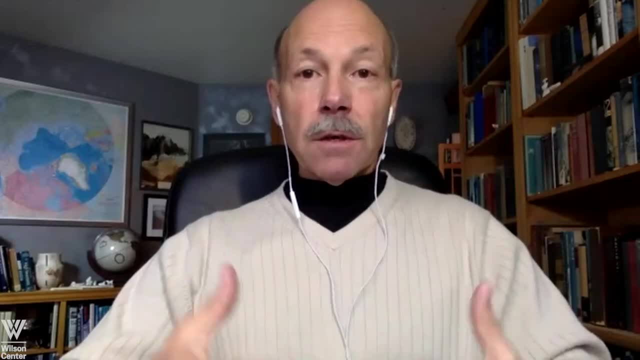 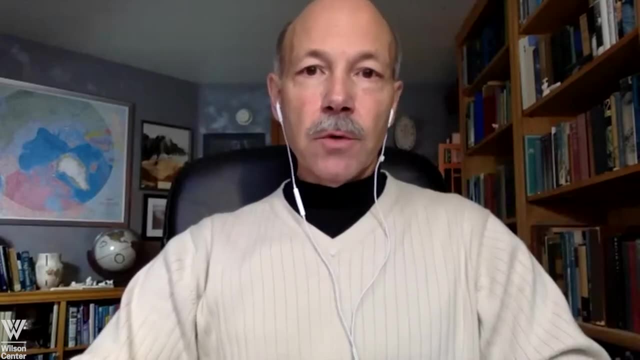 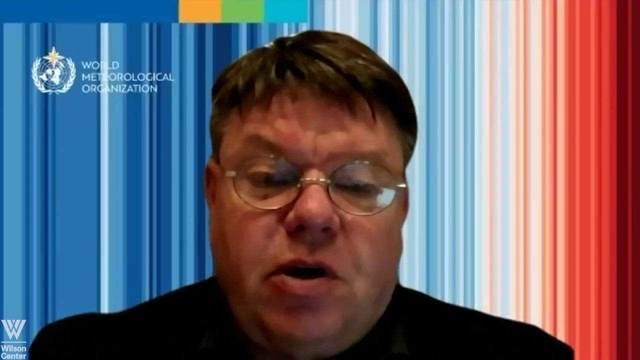 how are we doing in terms of our observing networks, our capacity to understand what is happening in the north, and is it enough what the international community is doing at this point to inform and influence the work that you do, sir? yeah, from our perspective, we have two major uh. 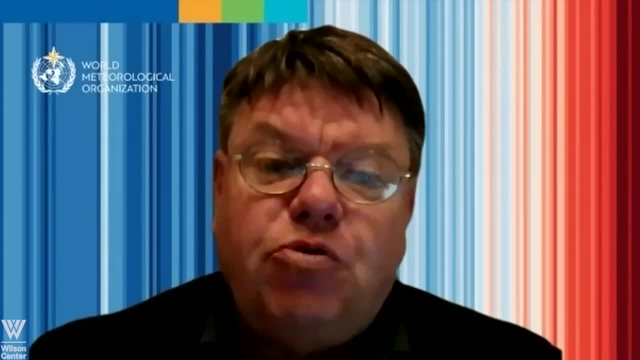 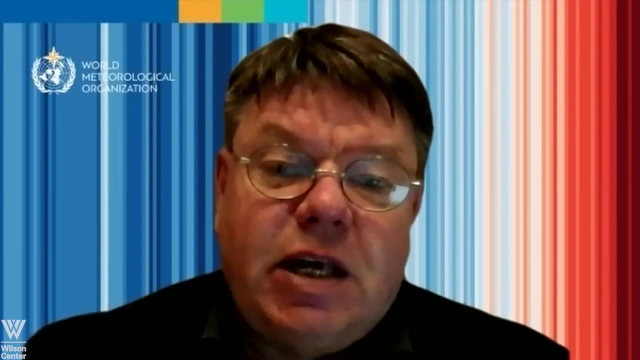 interests. one is uh one, the other one is related to operational services and and for that purpose our basic observing network is still too sparse. we are just about to set the new global standards for the observing systems. we will have our general assembly, our congress, in a couple of weeks. 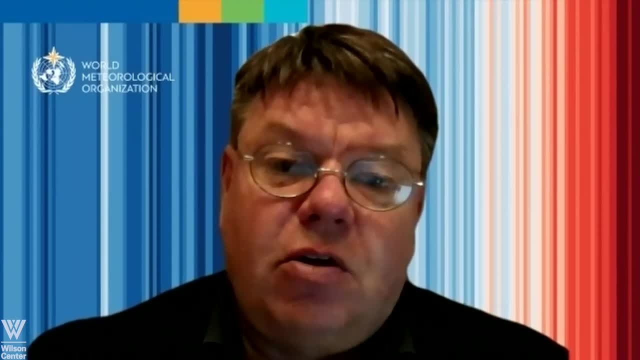 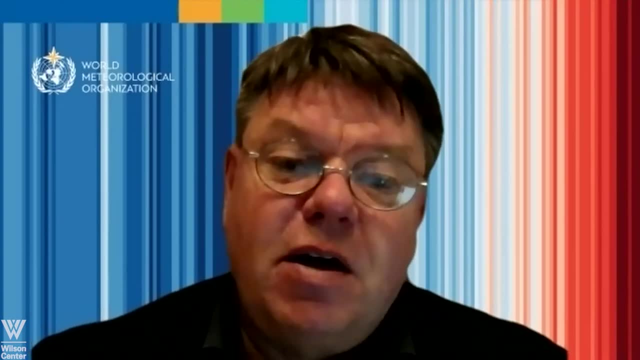 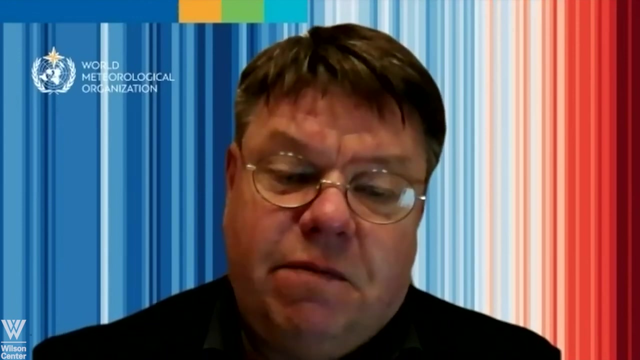 from now and there we are setting a new standard called global basic observing network. we and- and we have already heard some concerns from canada for example, that they cannot afford having such a dense network, even in a wealthy country like canada, and also russia is having difficulties. they have fairly dense networks in the european part of the country, but 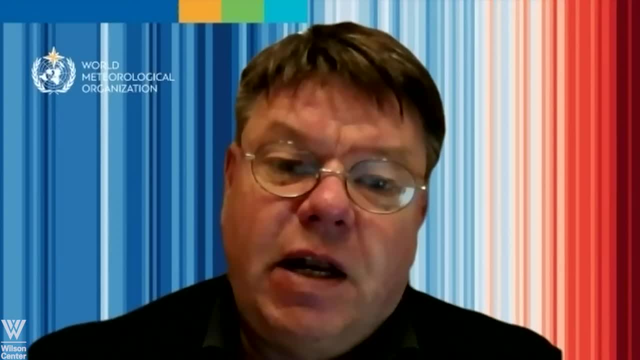 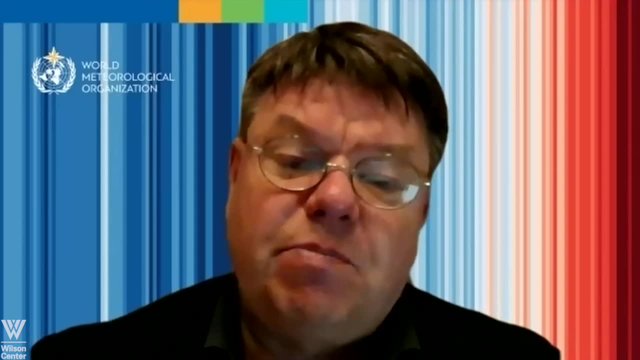 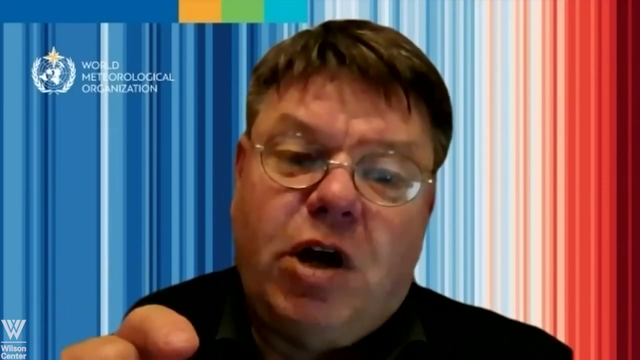 but the siberia is also very, very data sparse and of course these sea areas, that's that's also also a challenge, so so that means that the basic services uh in that region remain poor. if we would have more dense network we would have a better accuracy of our weather weather forecast. 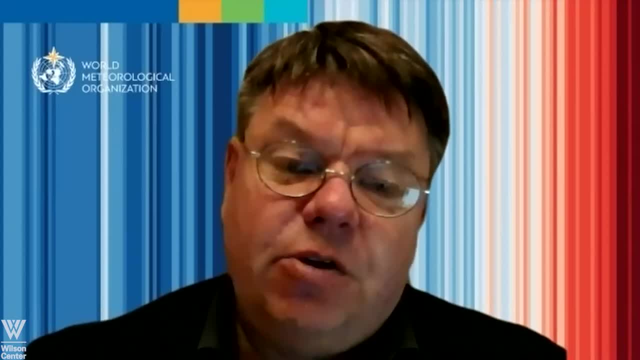 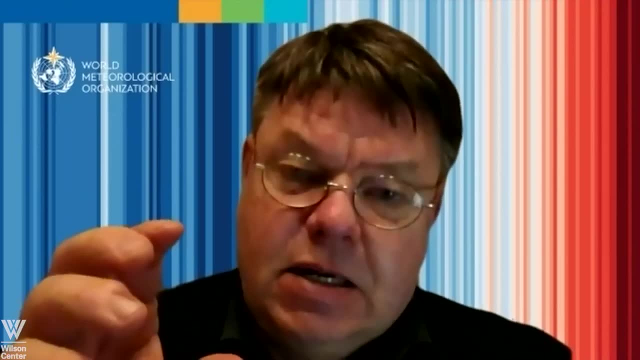 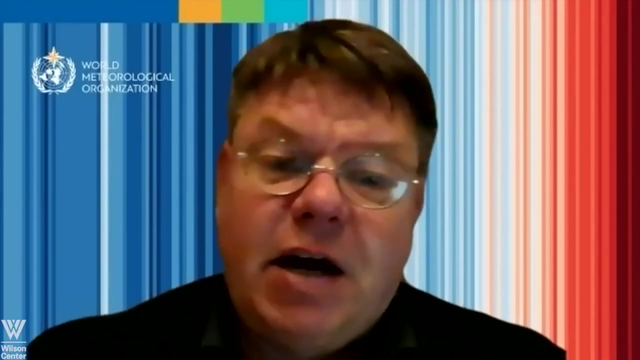 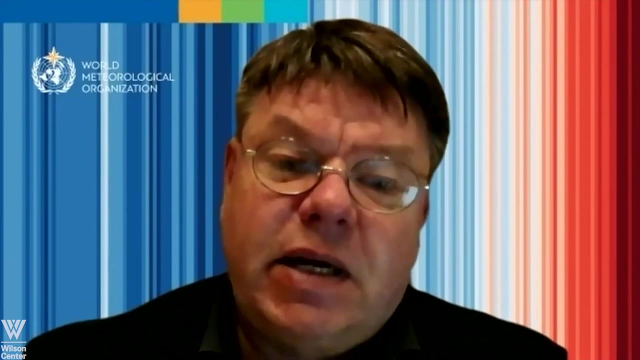 and and the other challenge is is related to, uh, to science and and, and and and to understand, uh, what's happening to the oceans and the atmosphere and the whole earth system, and also there we have challenges, and and and we should also do research, you know, directly into the ocean and our land to see in an example. 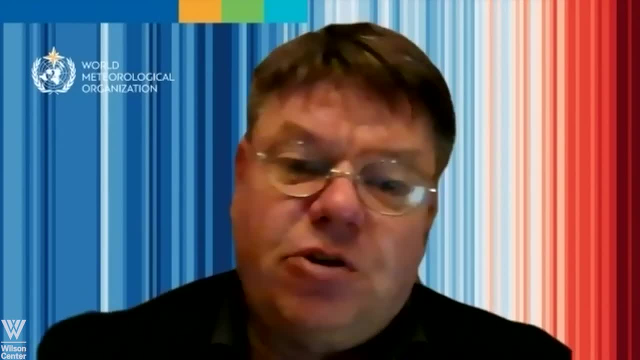 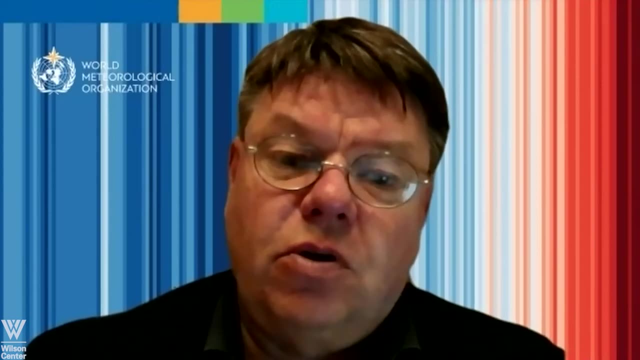 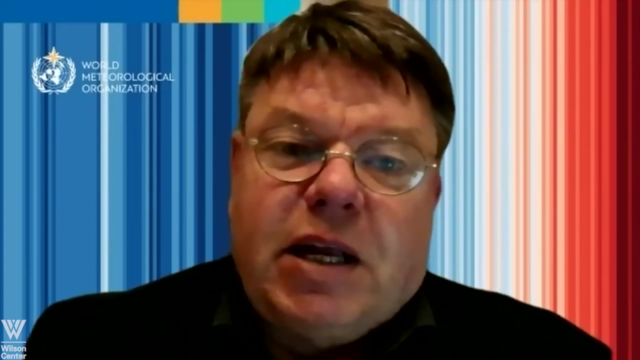 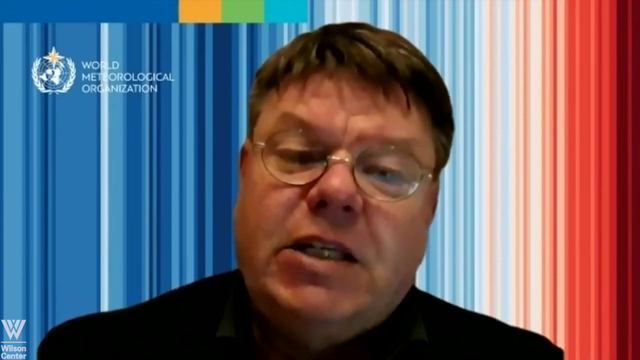 what would we be doing to do to What's ballast areas? I was wondering what you think about pequenaale. um well, so, Hmm, whether we are going to see some release of methane from the Arctic permafrost And so far. 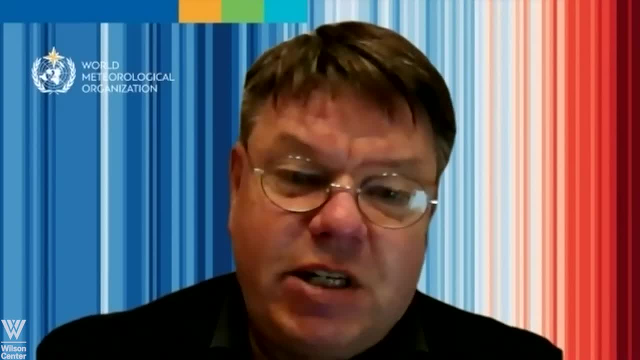 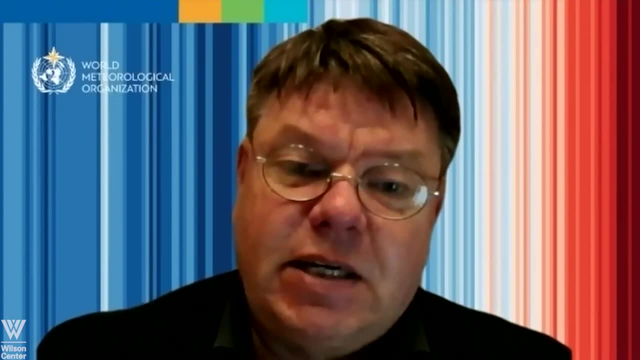 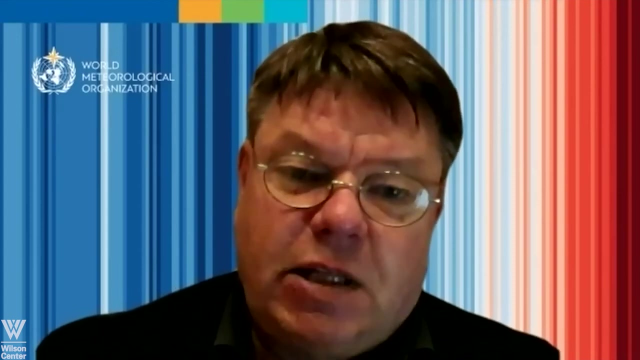 we haven't seen it happening, But this political situation is a slight challenge as well. For example, the USA was forced to withdraw from these Dixie operations because of some challenges with Russia already 10 years ago, But Finland has continued running those. And then my plea for 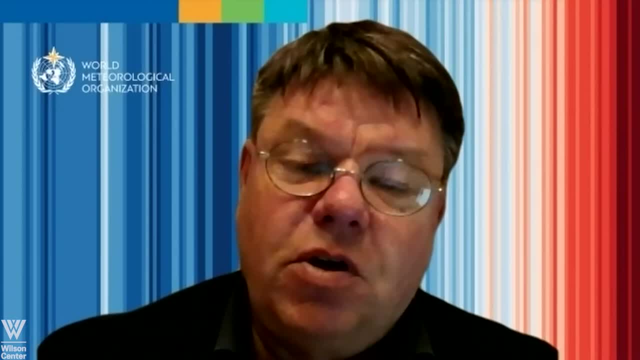 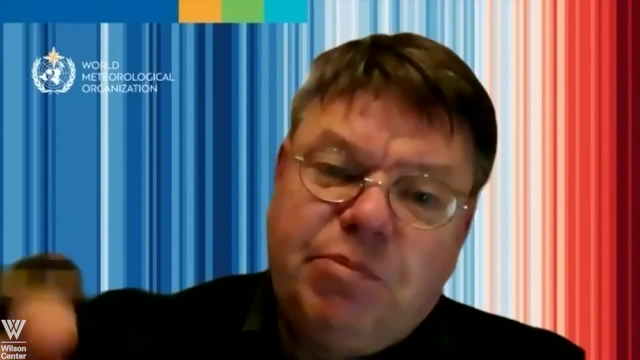 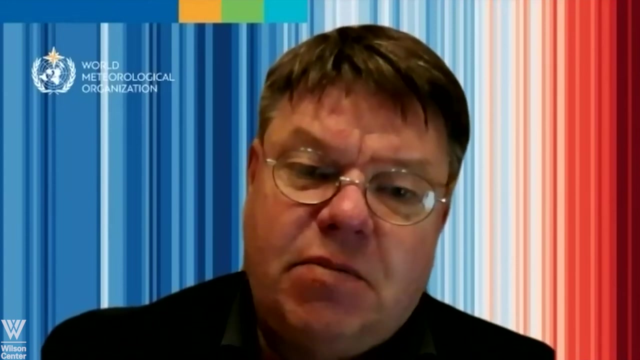 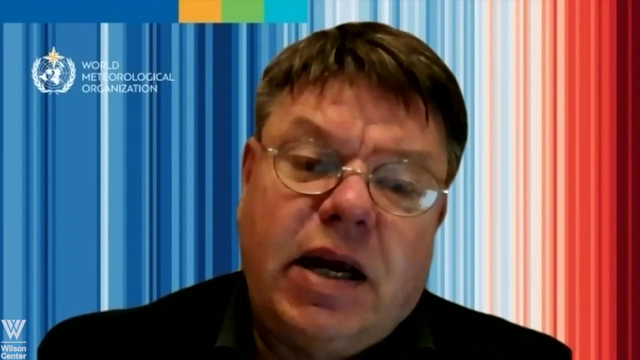 Santa Claus is always that we should afford a satellite program which would have this kind of Molonia, this electric Molonia orbit, And both NOAA and Canadians have been trying to set up such a program And that would enhance this data gap that we are having there, And the Canadians established such 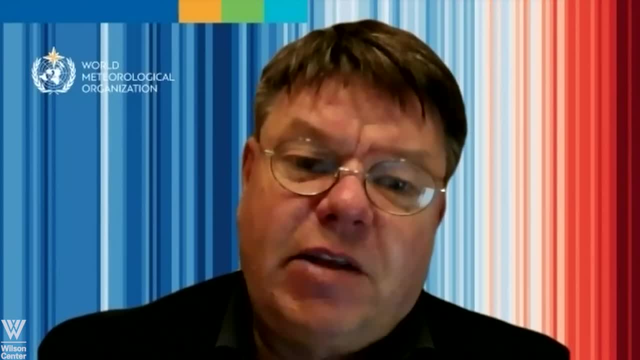 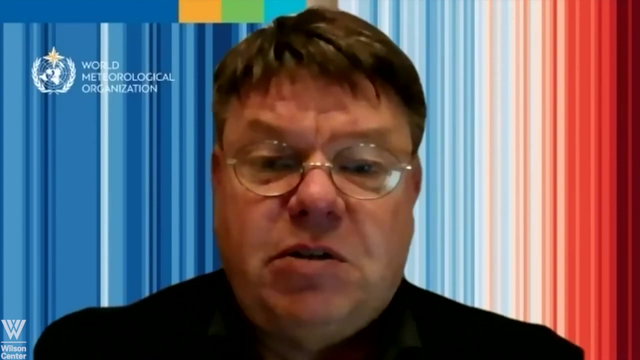 a setup, But once they took the military on board, the mission became so expensive that the meteorological part was pulled out of the mission. So that's still something that I would like to see happening And that would also come forth to need in the southern hemisphere, in the 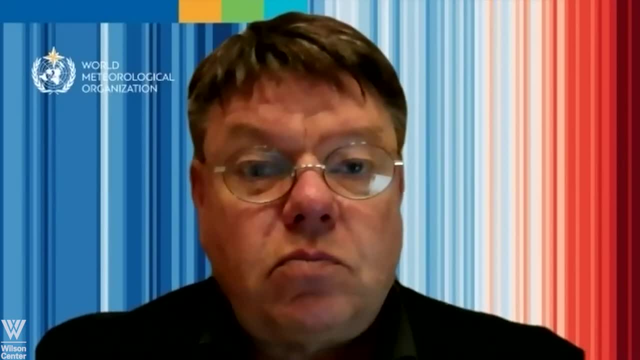 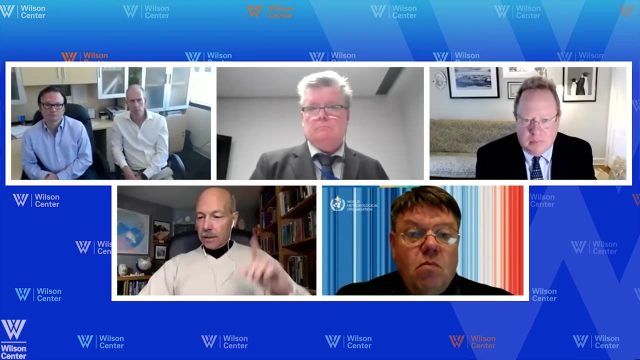 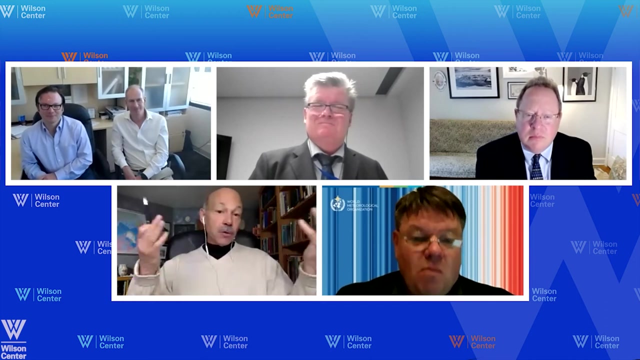 same way. Thank you for that. Let me just follow up on that just very quickly And we'll see what we can do. I just live a few miles from North Pole, Alaska, But I know all Arctic countries claim Santa Claus in one form or another, So we might as well all ask Santa's from our region for these. 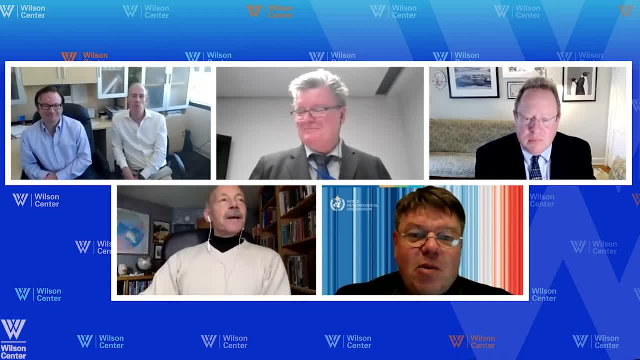 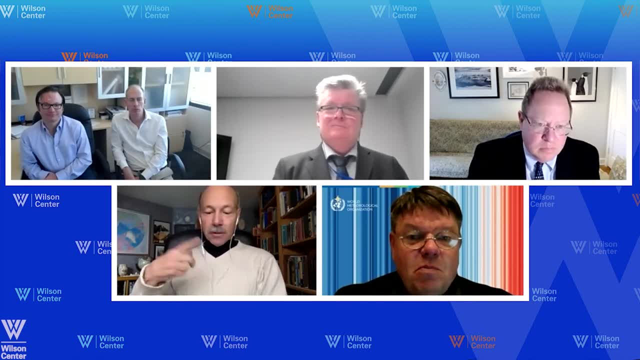 gifts, It can't hurt, Related to the costs of either, whether it's geosynchronized or elliptical orbit satellites for data. you mentioned the cost. Yes, Yeah, Yeah, Okay, NOAA and the Canadian government, but I'm wondering with all of the private industry now. 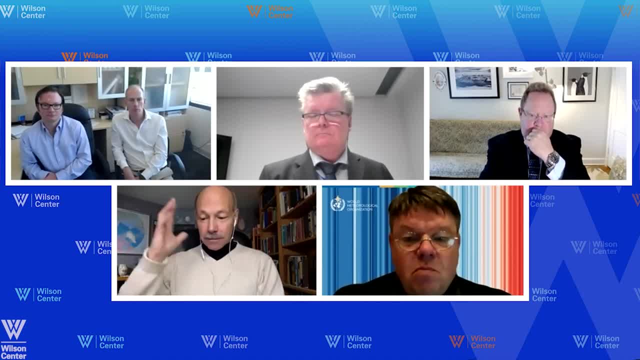 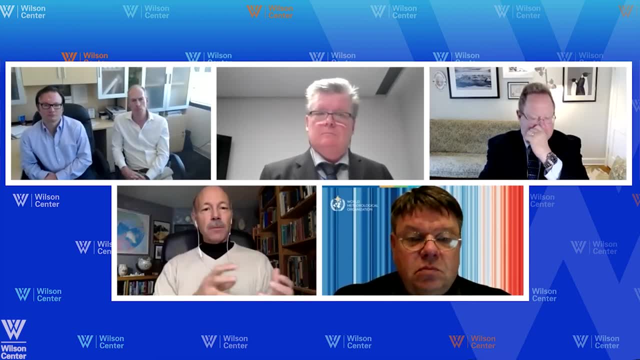 all of SpaceX and all of these incredible advances in such a short, what seems like a short period of time. I'm wondering: is there a combination within these public-private partnership sphere that could advance Arctic research as well? That's a good question, And we have started. 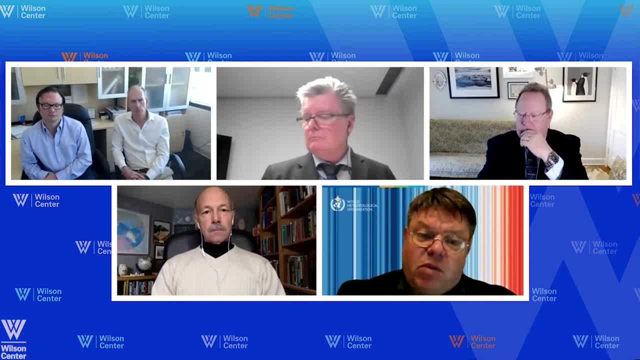 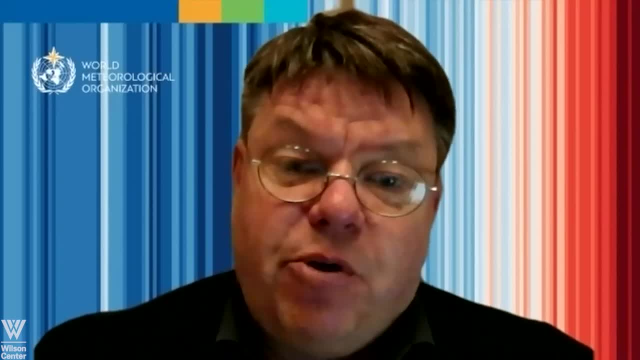 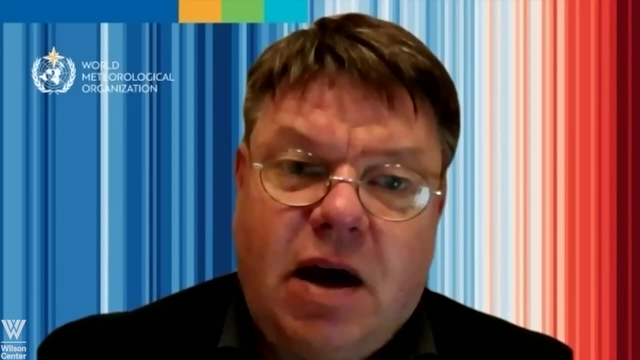 seeing growing amount of private sector-driven satellite programs, And since these microsatellite programs are becoming more affordable for the private sector, that's already happening, But so far we don't have dedicated Arctic ones. Finland has a company called IceEye which is providing. 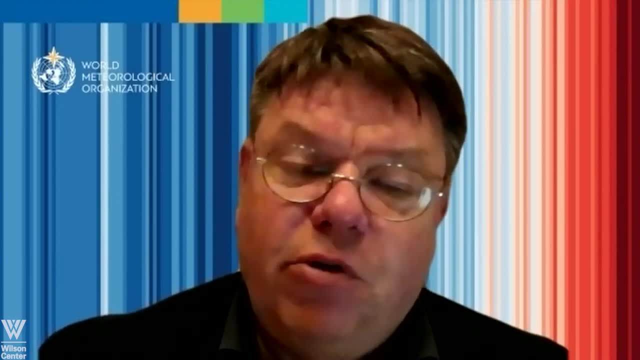 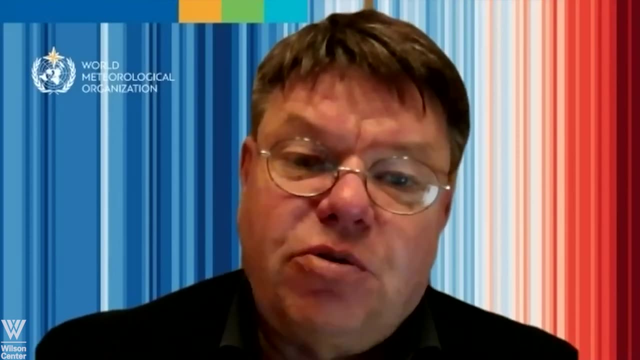 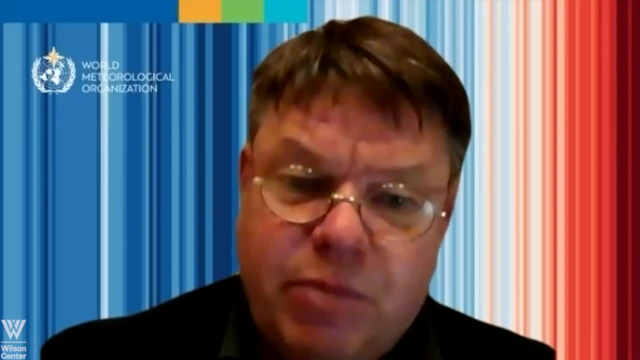 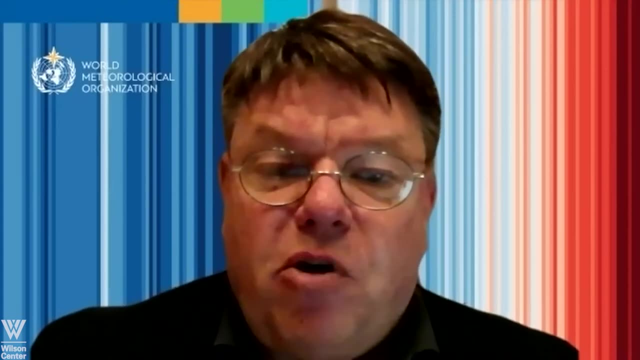 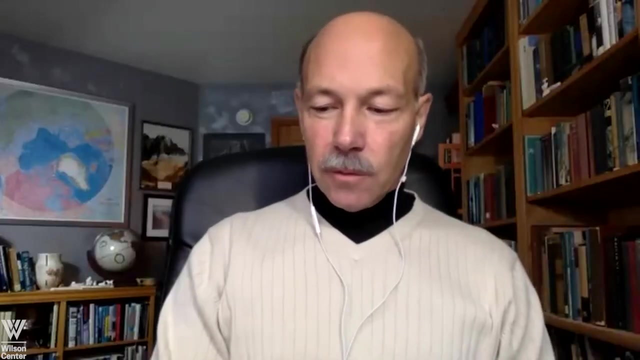 very much favoring public-private engagement, so joint ventures, And if we are able to open such a window, that would be great, Thank you. And of course, we're familiar with our friends at IceEye and the work they're doing. It seems like maybe that's a new trend, especially since 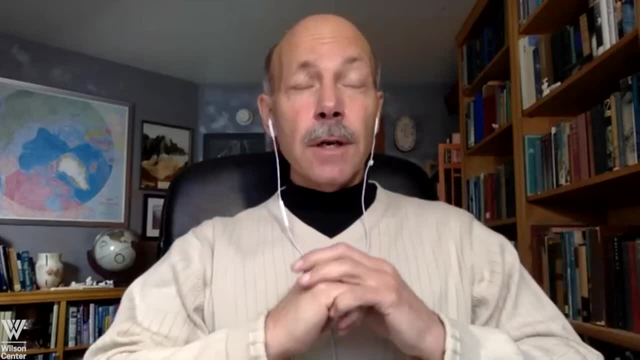 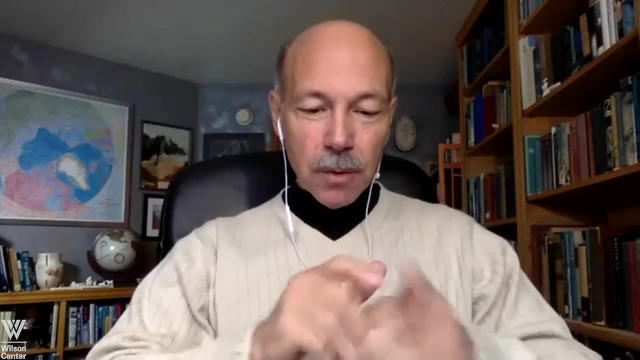 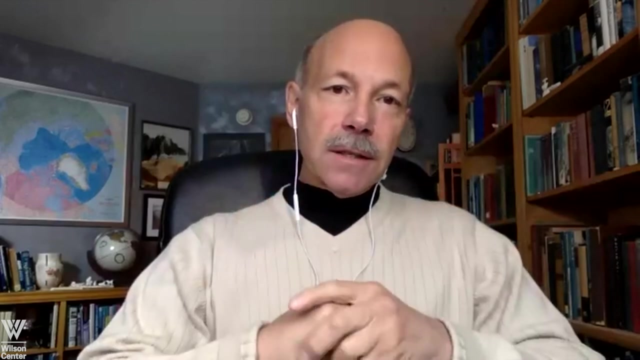 we're all struggling with how to provide good data for good policy. I have so many other discussions, questions about COP And other things. maybe we'll have some time to come back to those. But, Mr Ambassador, a question to you about the Arctic Council here for a moment, And I'm glad you linked 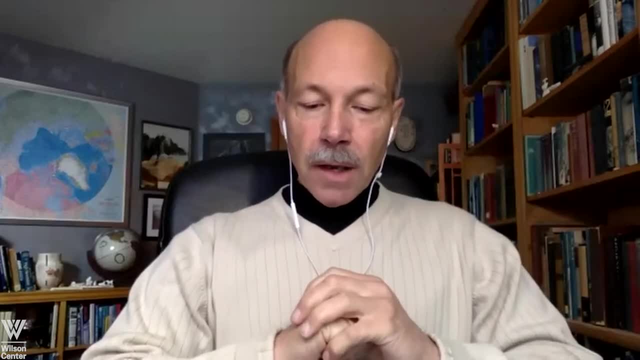 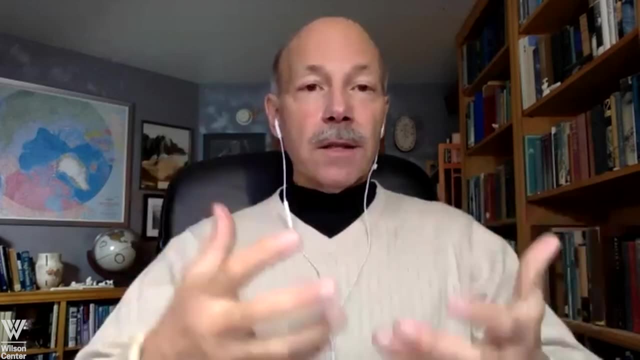 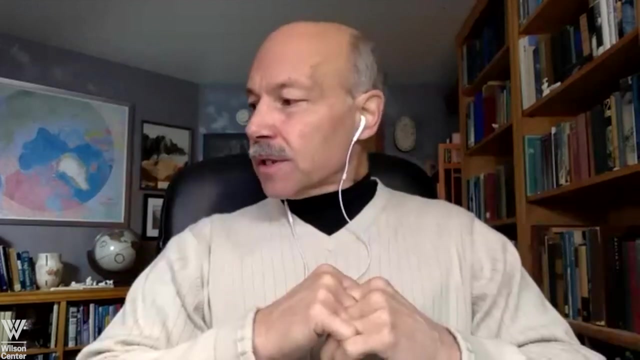 Arctic and Antarctic, as Evan did as well, But in terms of the Arctic Council, it is the most consequential forum at the moment for Arctic nations and non-Arctic nations to participate in. I'm wondering what you see for the Arctic Council. 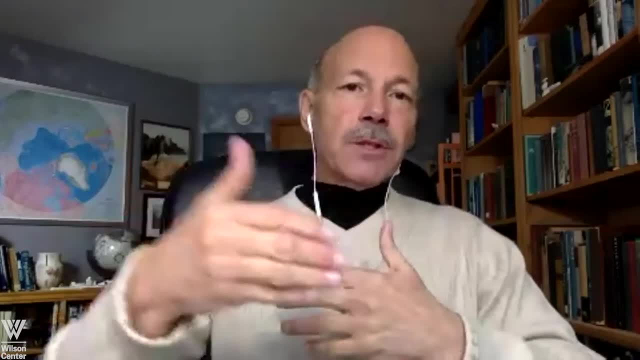 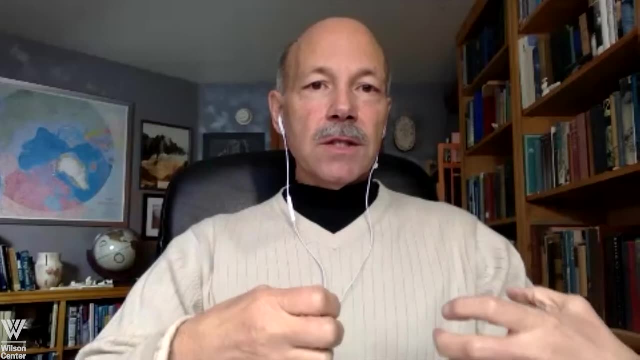 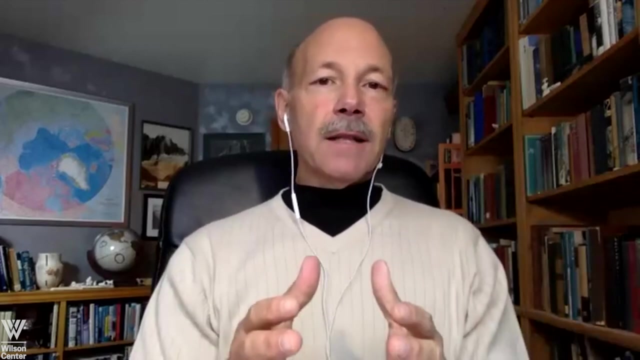 in the next few years, not chairmanship by chairmanship, but in terms of the expectations on the Arctic Council. right, I mean it's now. it went from trying to explain to people what the Arctic Council is and now has almost become a body that has the expectation level up pretty high. 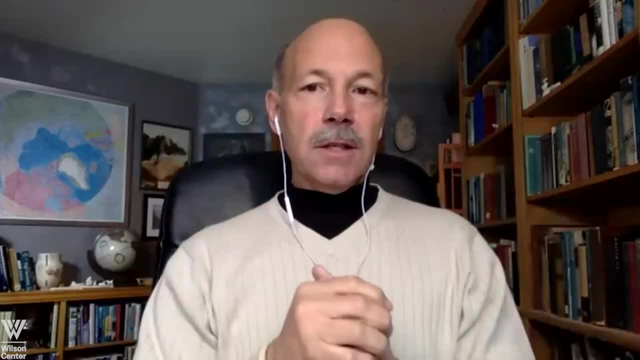 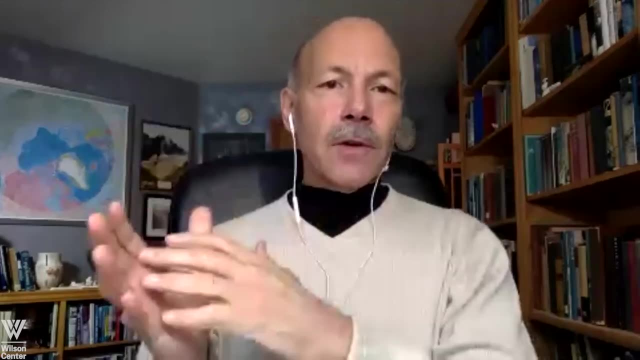 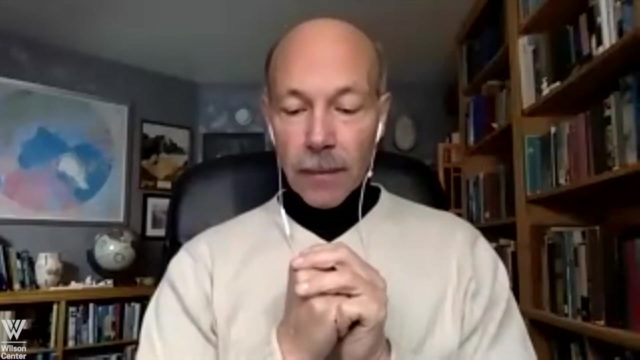 to navigate so many issues, And what are your perspectives on its ability not to get into other areas but to simply keep up with the rate of change in the North, knowing full well, as Evan pointed out, the history of where the Arctic Council comes from, came from and why it? 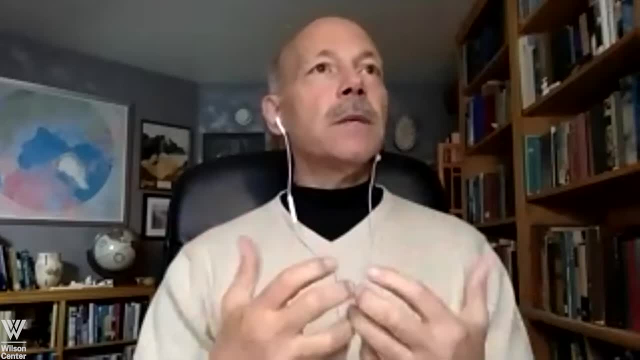 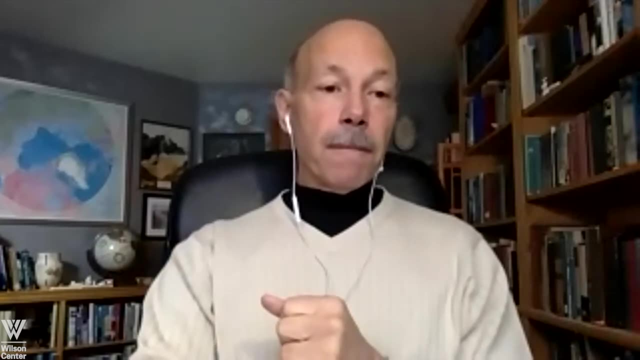 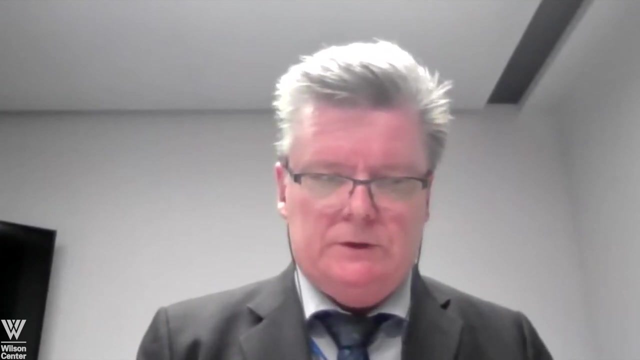 was created. What are your thoughts about its ability to keep up with the rate of change and so much that's going to be demanded of it in the next few years? Thanks, Mike. The Council will be faced with challenges. I'm convinced that we will be. 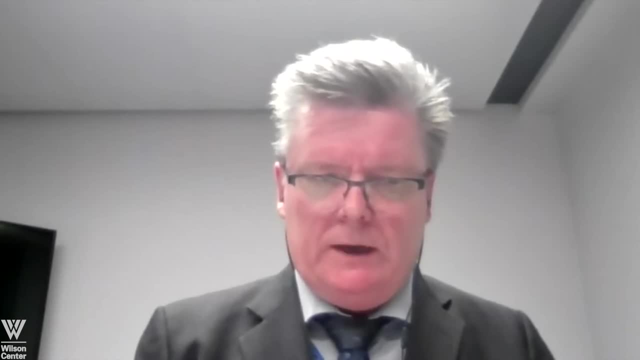 able to face the challenges, but a lot of work lies ahead of us. There are so many new things that we need to address public health and the pandemics, the economic cooperation-related aspects at large, that there's a whole big issue with the marine governance and the BBNJ negotiations. 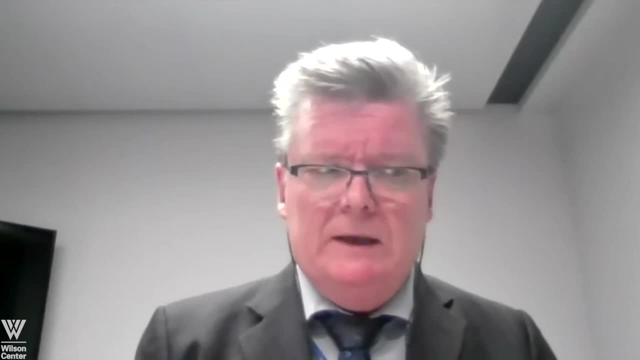 and also really our interaction with our observers. I mean, we're a council of eight member states and a permanent member state and we're going to have to face the challenges. We have 38 observers currently. Several had applied before the Reykjavik meeting. 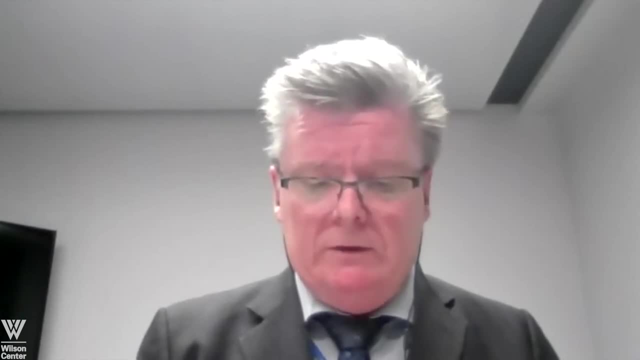 I am aware of several others who are planning to submit their observer application. So that's something that we need to reflect internally and we will have ahead of us a strategic reflection during the Russian chairmanship, and I hope that will be conducive. I think some of the 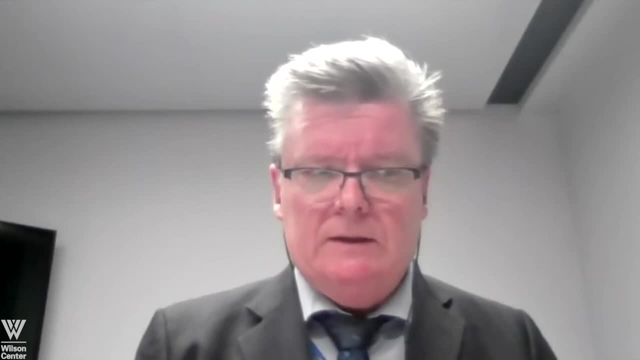 challenges. one can read in the Reykjavik declaration and the strategic plan that were adopted in May, but my firm conviction is that the Arctic Council shall remain the preeminent forum for circumpolar Arctic cooperation. I don't know who could possibly replace it, but it's not a free ride. 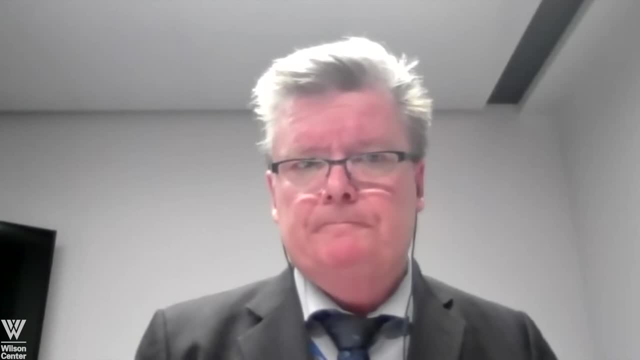 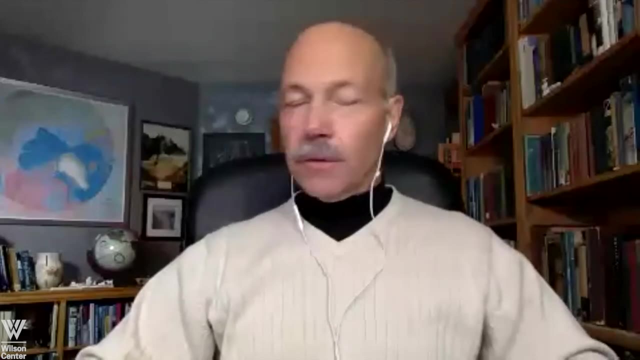 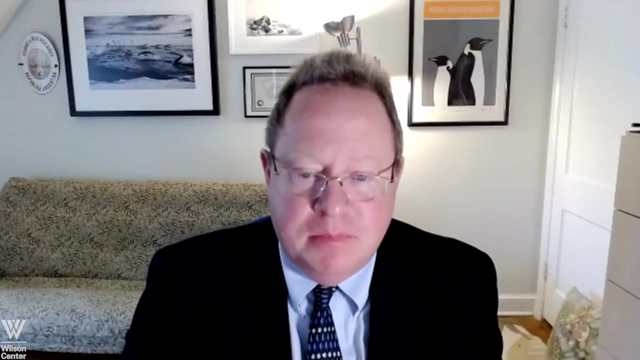 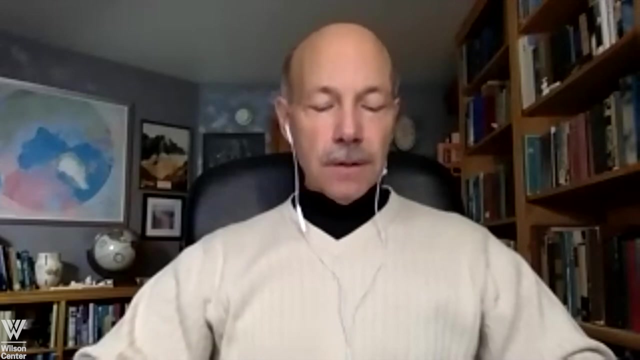 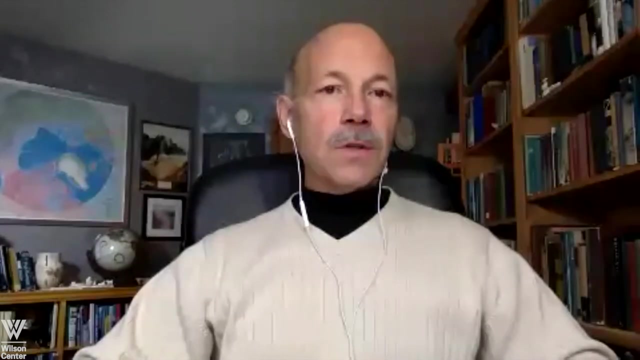 and we need to reflect carefully how we threat forward. Thank you so much, Maybe to my colleagues who noted the strategic allocation of their assets. You both noted the future role of the company and its efforts to serve the community. So back to the Secretary General's comments about the need for more robust observing networks platforms. 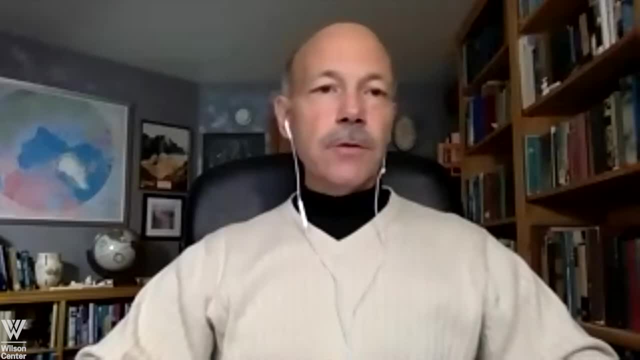 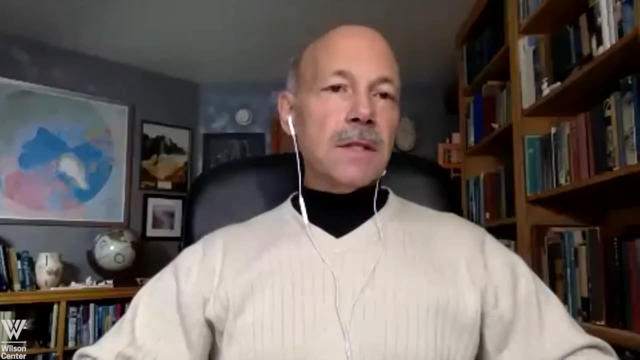 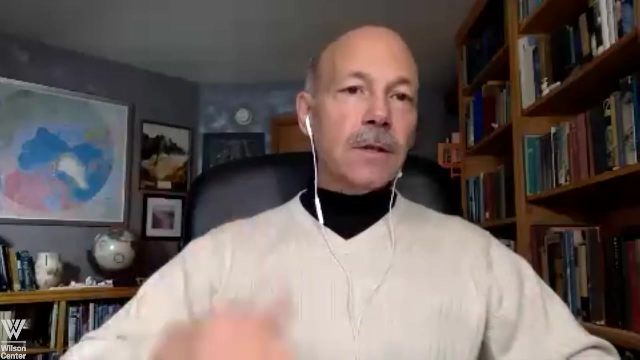 locations- It's the terrain that you try to cover, both in the Arctic and Antarctic- are simply mind-boggling. How do you go about deciding your priority list? What are the priorities? Do those come from inside a corporate model, or do they come from external and the needs of the community? 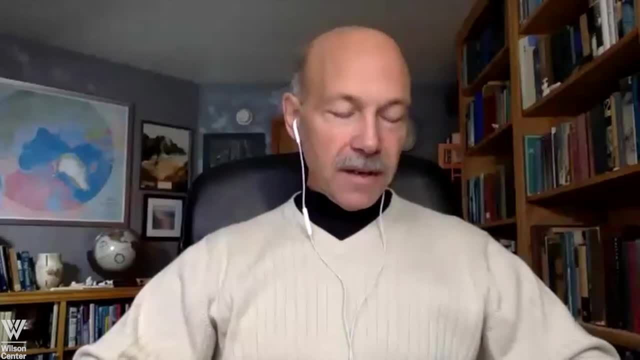 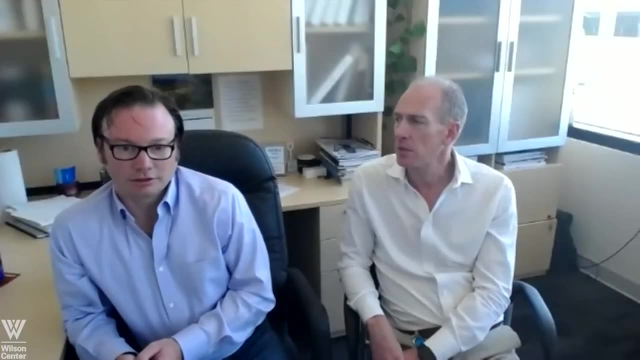 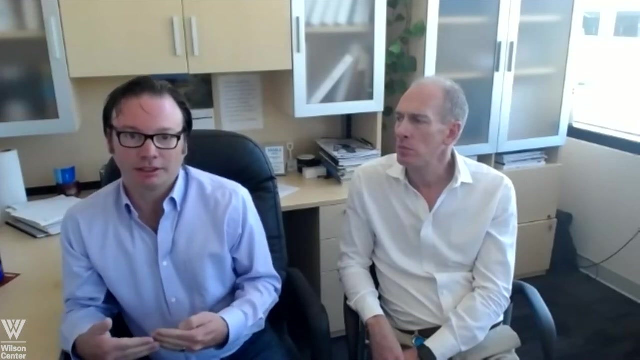 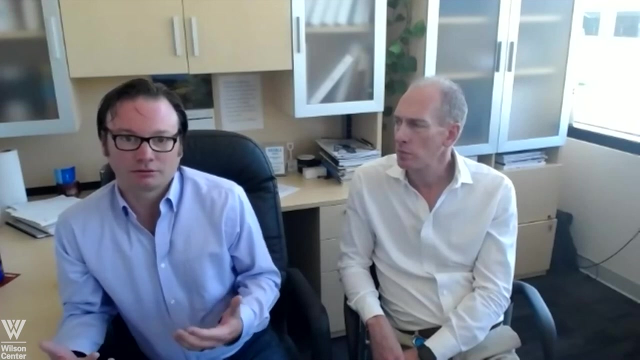 to try to solve problems that we're currently all faced with in both polar regions. It's certainly a challenge, and what we do as a company is we look at how can we meet some of the UN guidance on certain policies, And then we also are listening to the weather community at large and what are their 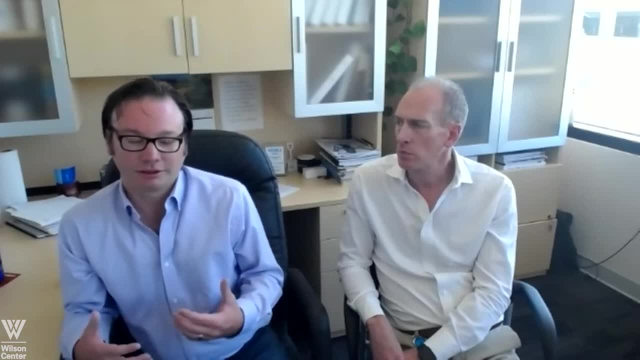 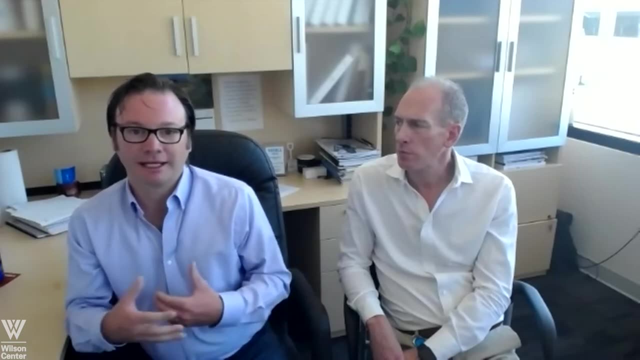 focuses, And so we want to work hand in hand with the people that are doing the measurements, people that have those measurement challenges, and the people that are taking that information and using that to make certain policies or make certain decisions based on those measurements. 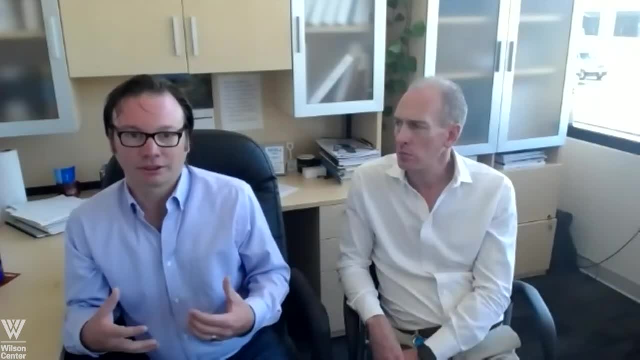 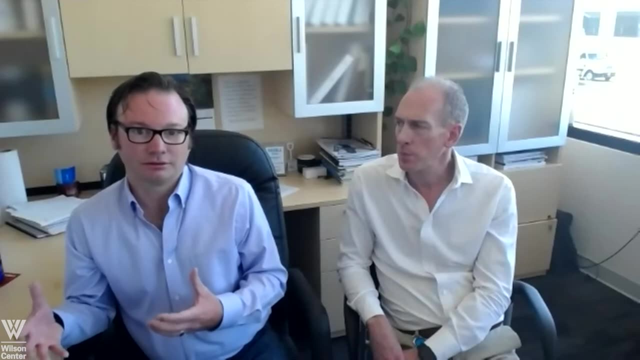 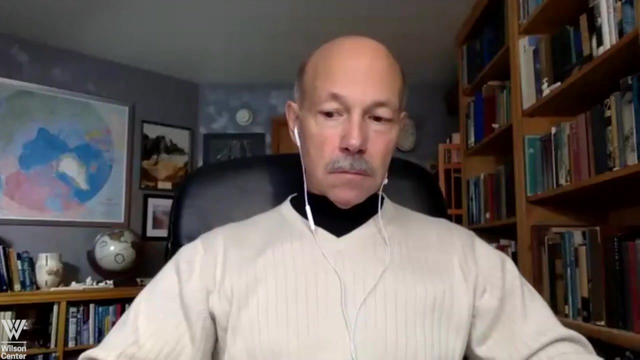 So we see ourselves kind of working together and bridging that gap between the policy makers and the people that are collecting the data to inform those decisions. Thank you, Thank you, Just a quick comment. There is probably a challenge and Chris feel free to weigh in on. 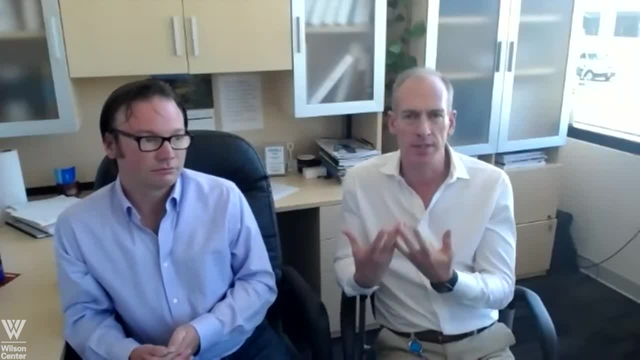 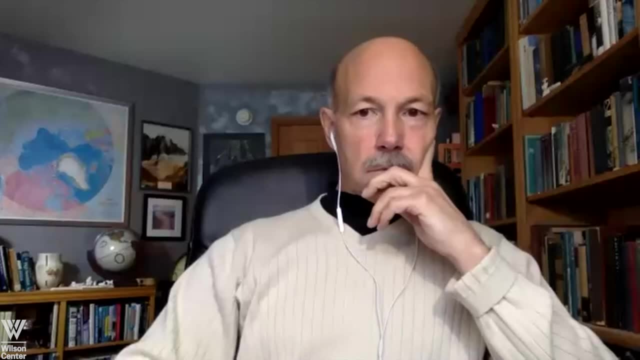 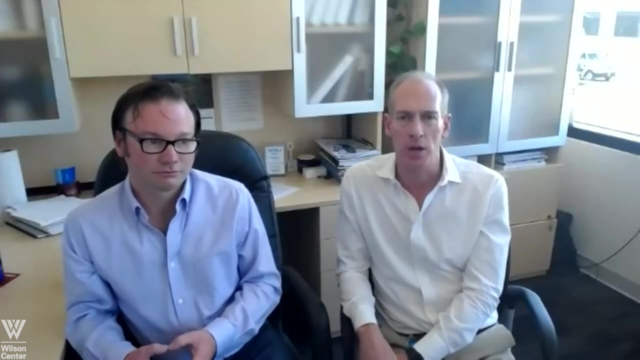 this, that we obviously generally sell the data We sell to government entities and the like, And when there really is no country right at the pole, on the North Pole, and then Antarctica is its own split between certain outposts. who is the customer in that scenario? 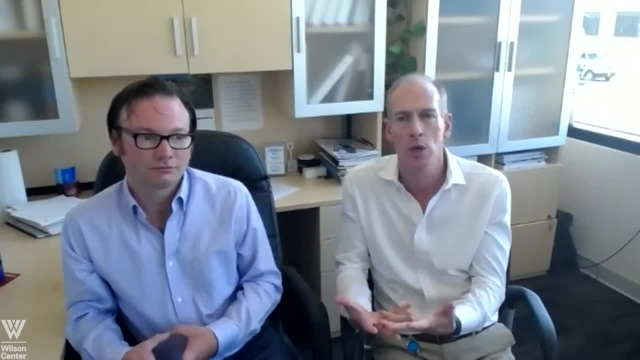 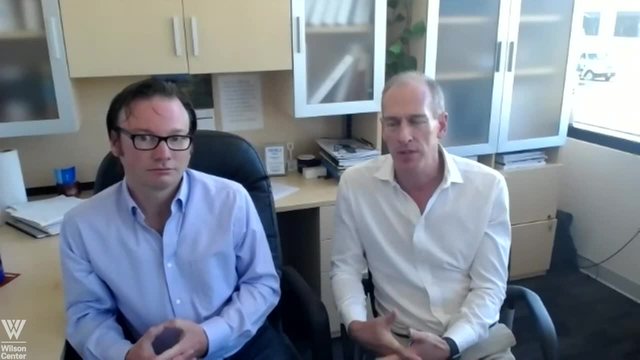 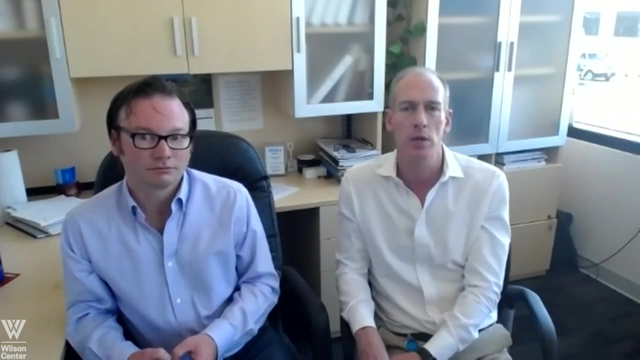 So that gets a little bit complicated. We certainly want to do our part and serve the world at large as best we can, But sometimes I think it's a challenge in terms of who's actually buying the equipment and why, And so that's something that we have to factor in. 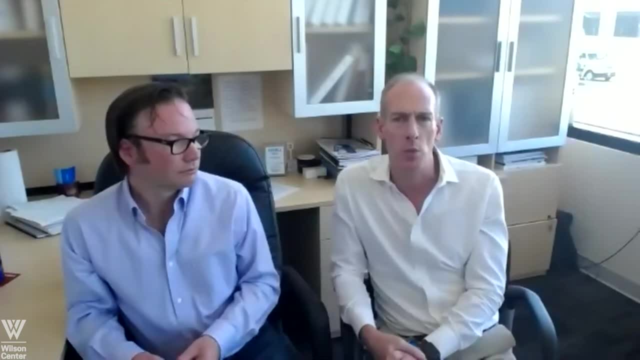 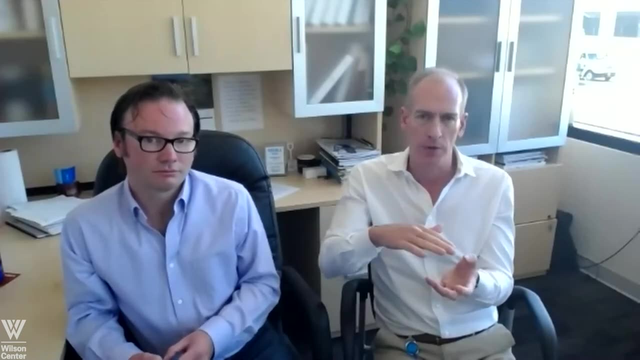 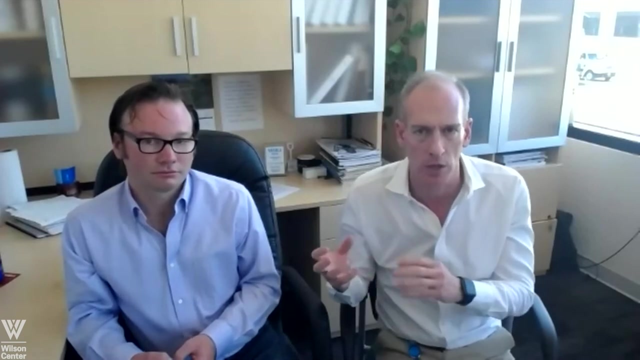 But one other thing that was mentioned is we feel very strongly at Vaisala that there is the need to cooperate both with our observations at the surface level and up into the atmosphere and then combine that with what satellites can do, That we don't feel like we're a competitor. 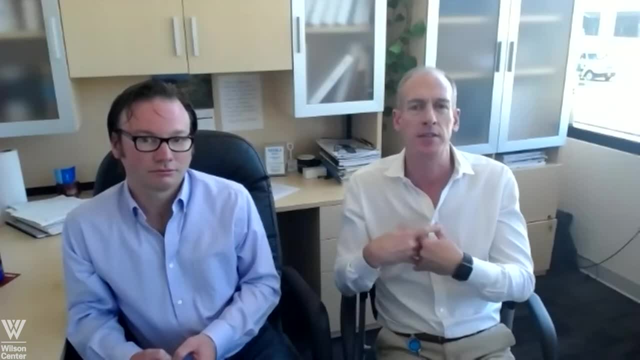 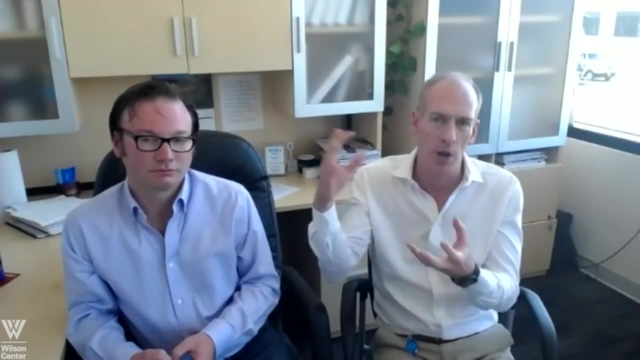 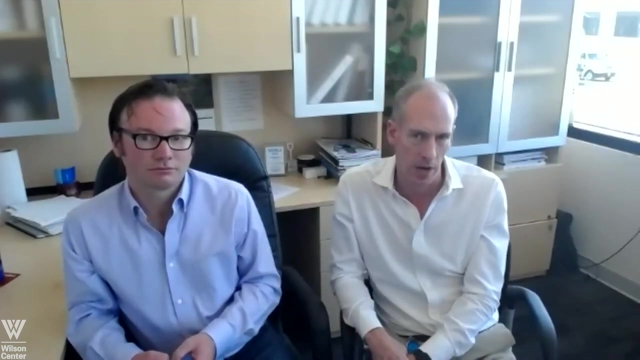 to satellites and I hope they don't feel like we are. I think it's the production of a program, but it's the production of a full data set from both what we cover and what the satellites cover that can provide the best data for the world at large to be able to forecast, compare and make. 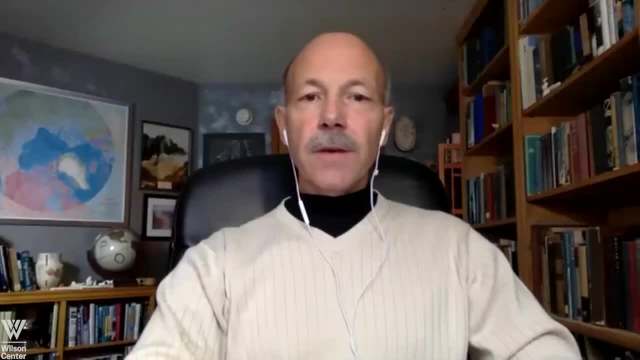 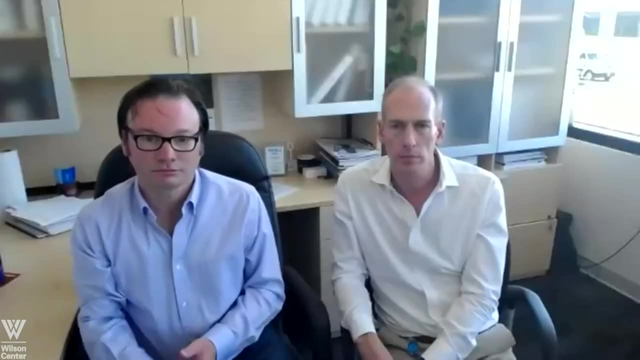 the determinations about climate change. Yeah, that's good. Thank you very much, Evan. I'll put you on the spot here. I want to focus a moment about the Antarctic and Secretary General. I'll come back to you for a follow-up. 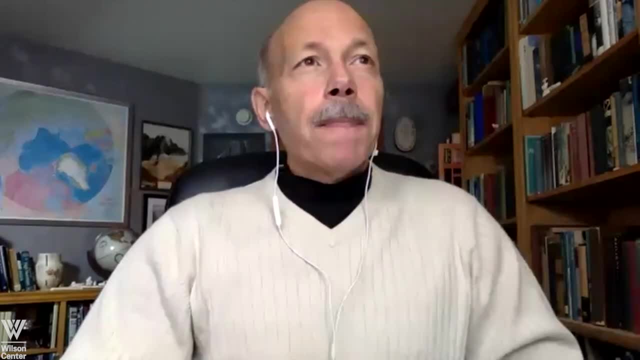 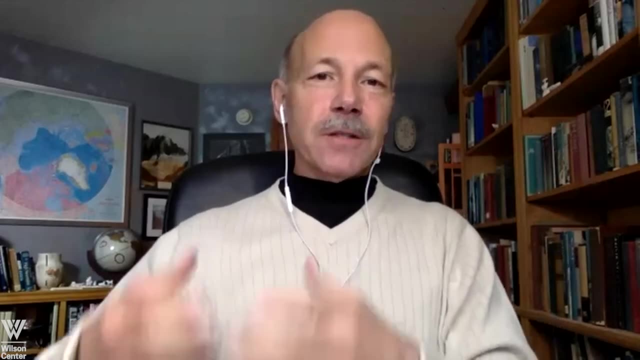 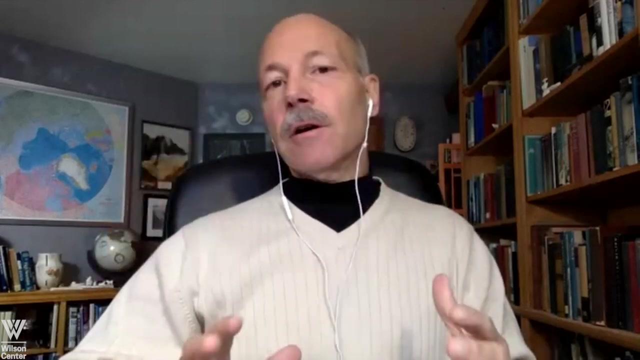 I want to talk a little bit more about this dual emerging narrative: The Arctic. now you hear about the Arctic far more often today than you did even five or 10 years ago. right Now, you can throw a dart at a calendar. Odds are you're going to hit the date and there's going to be an Arctic meeting. 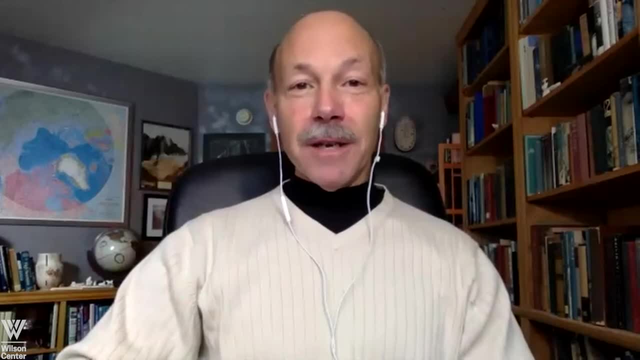 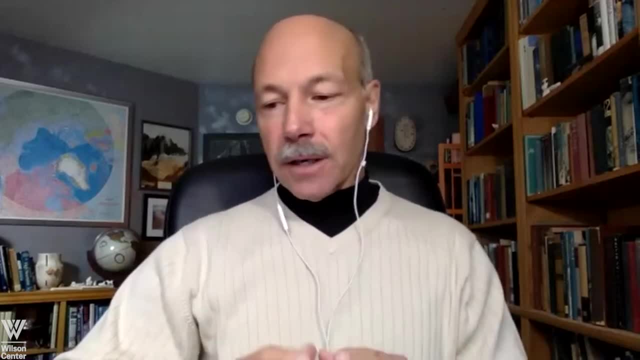 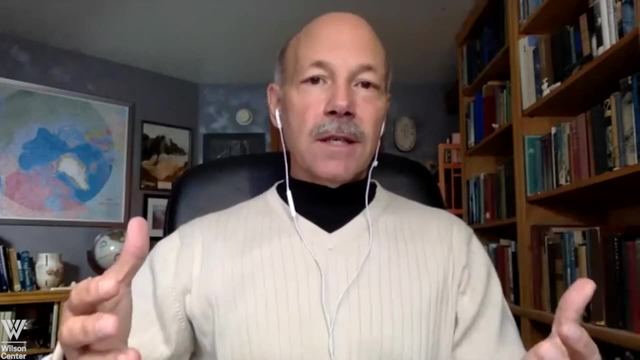 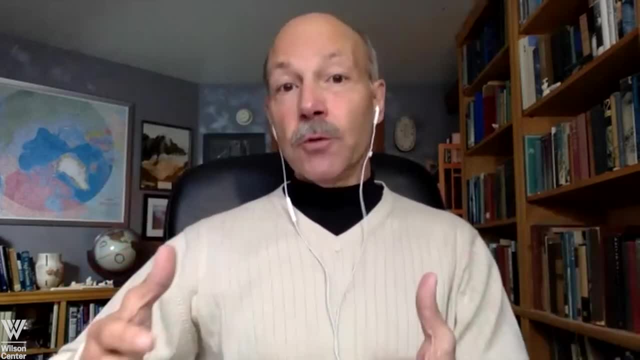 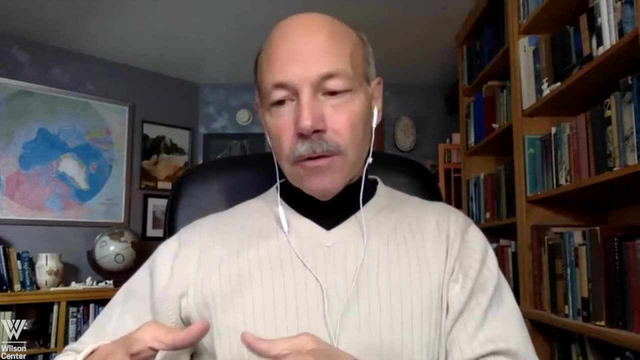 everybody has equities in the North. You may not think you do, but you do. You have a connection to it, And so in some ways it's a good thing. But now I would argue, maybe it's just that we 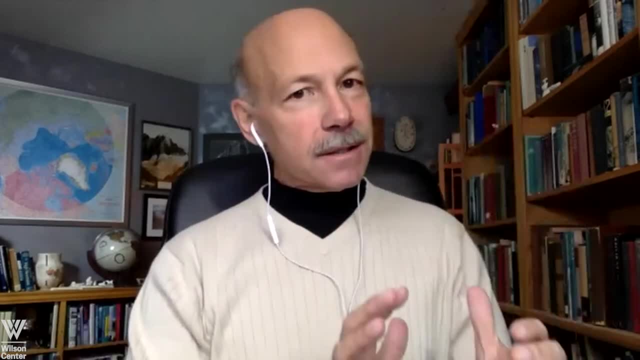 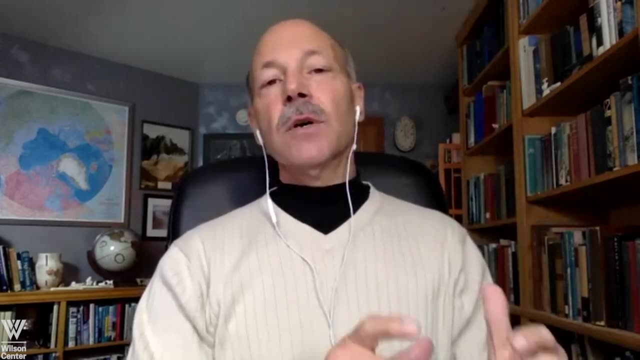 follow it a lot. The same is sort of happening with the Antarctic And it's sort of it's a very different narrative, But we're hearing more and more about the Antarctic mostly, mostly about the issues related to climate. So would you agree with my statement that we're hearing more and more? 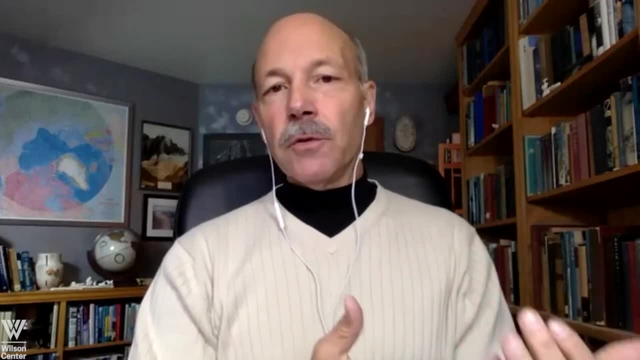 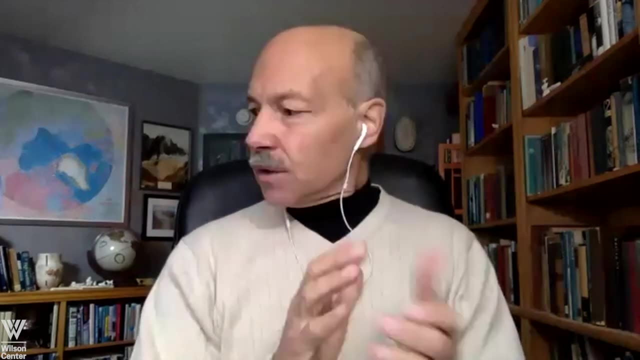 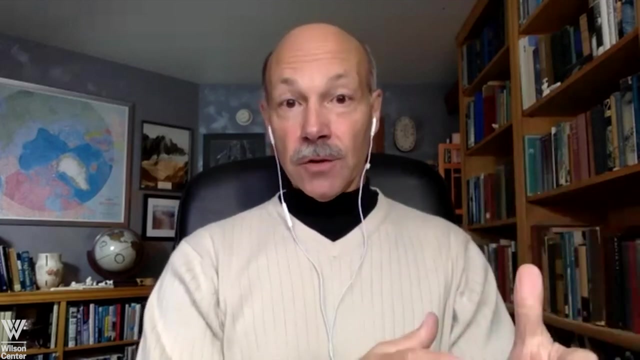 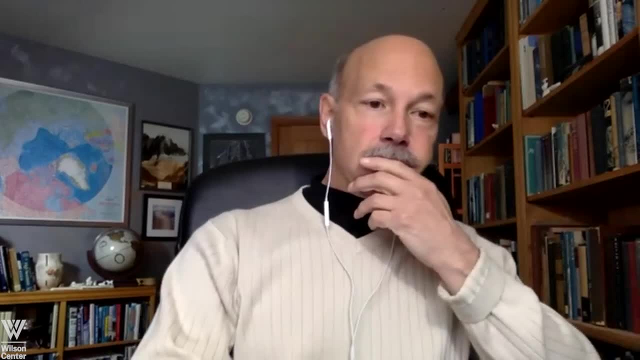 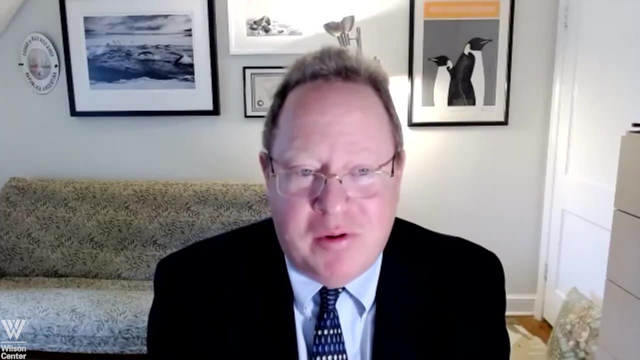 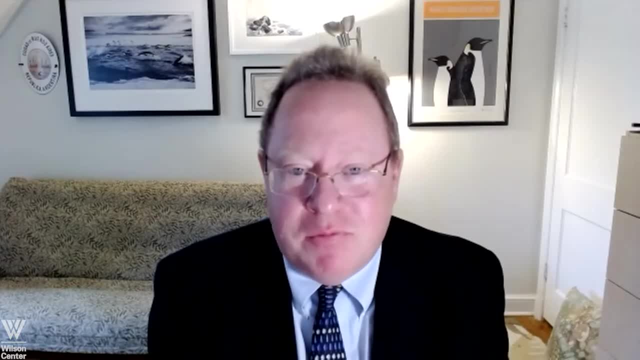 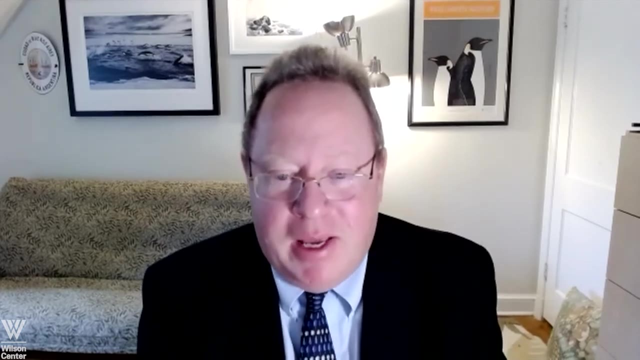 That is, if you go to southern hemisphere countries, if you talk to Chileans and Australians and others, they probably have a few more conferences and focus on Antarctic, Antarctica than you would find, say, up in, up in Alaska, And I think that scientists in general, if you go to the National Science Foundation, 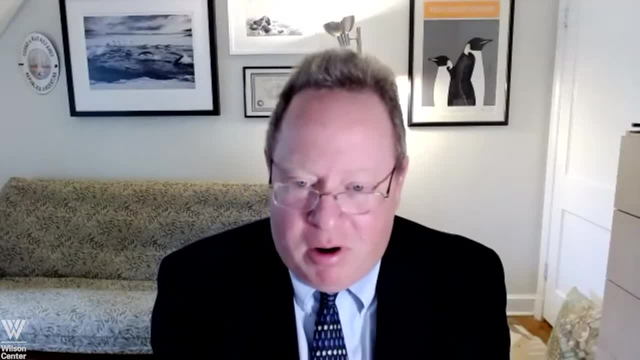 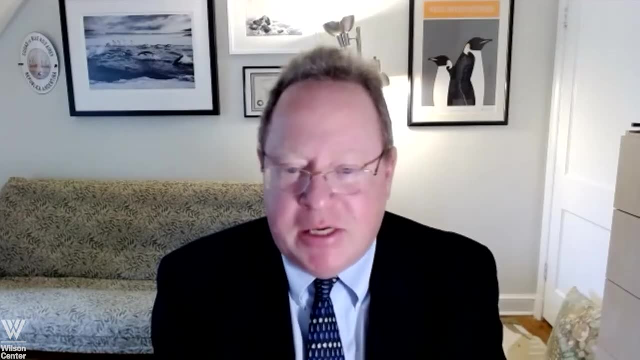 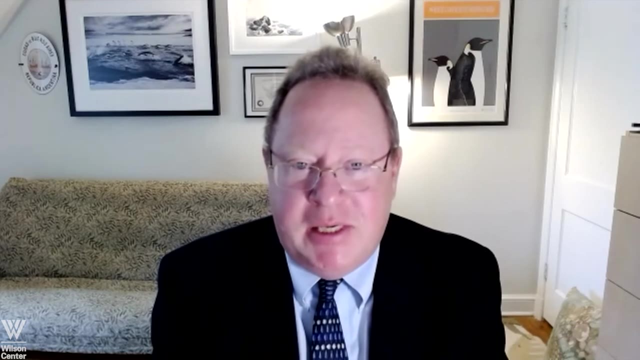 they have an Office of Polar Programs. It's not just Arctic. They are focusing on Arctic and Antarctic science and the connections between the two. So, especially as if you look at the work of the IPCC and others, I think they're valuing both And 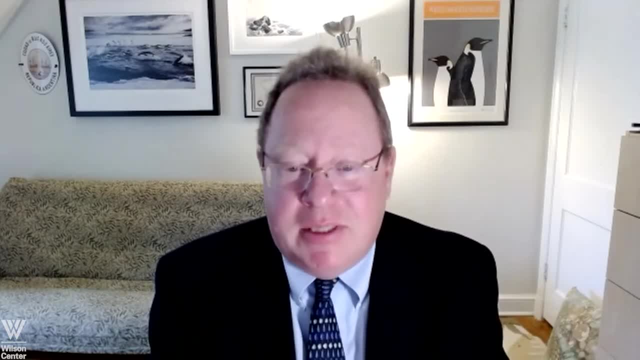 that, yeah, Antarctic policy and Antarctic science will become more and more in the forefront, especially when it comes to issues like sea level rise, where you can't really talk about that issue without looking at what's going on in Antarctica, not just Greenland and other places. 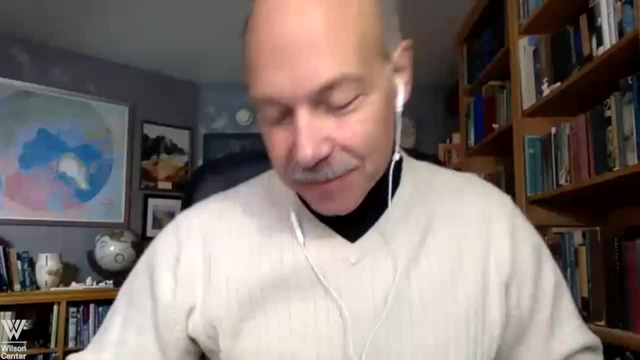 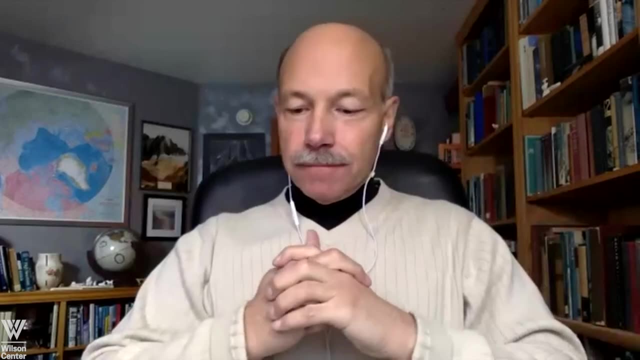 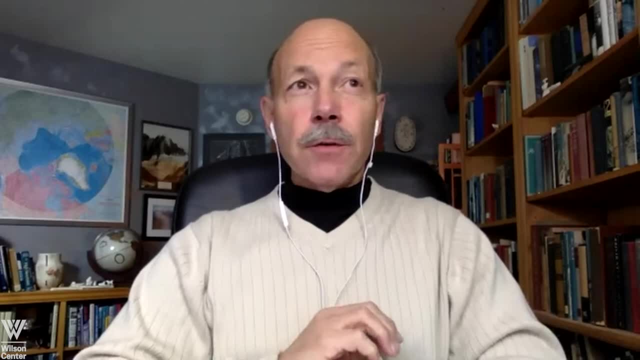 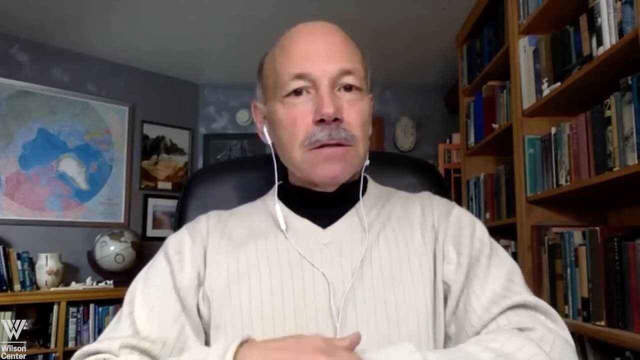 for the Secretary General. You noted, of course, we all know COP is coming up. There's so many issues, so many issues to cover in COP. You mentioned, and there's everything. there's political, economic, there's food availability, parts of our world like the, 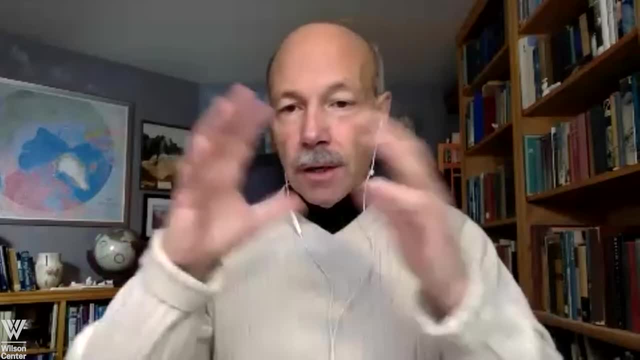 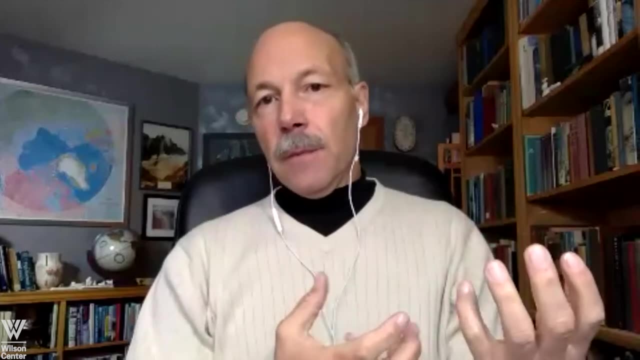 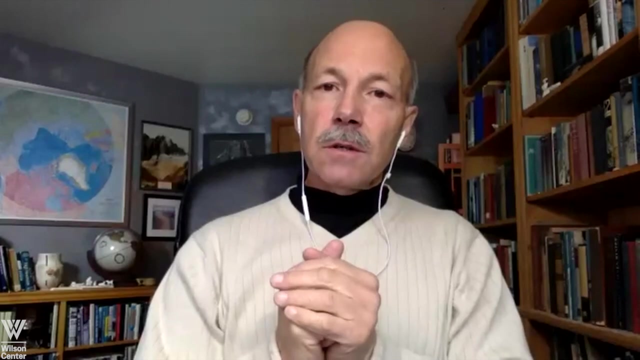 African continent. so many pressures there won't go into all of them When you were there at COP. how will the Arctic resonate at COP? I mean there's so many other incredible issues to address there. Do you see the Arctic elevating to a narrative equal to many of the other challenges? 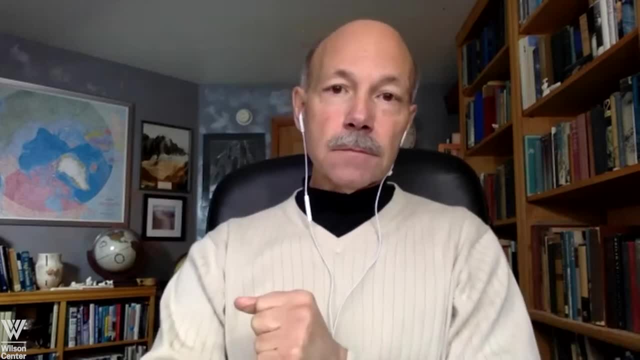 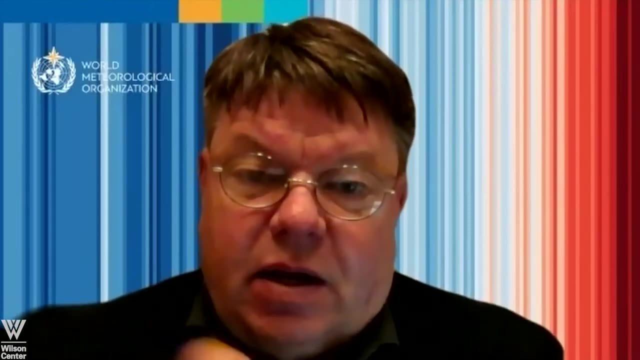 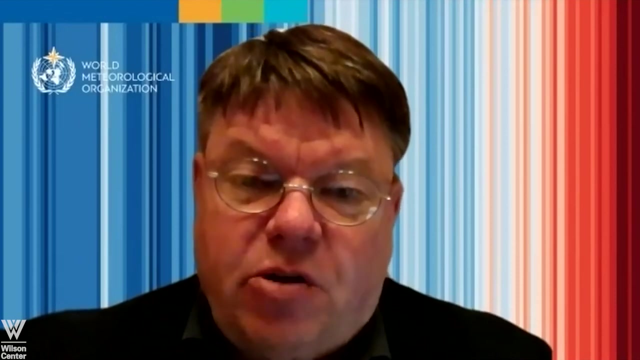 related to the discussions that are happening there. Yeah, of course. So the key issue is to to touch this MEC question, emissions and one of the questions- a couple of questions are related to this- but potential release of carbon dioxide or methane from the permafrost or from the bedrocks of the sea areas. 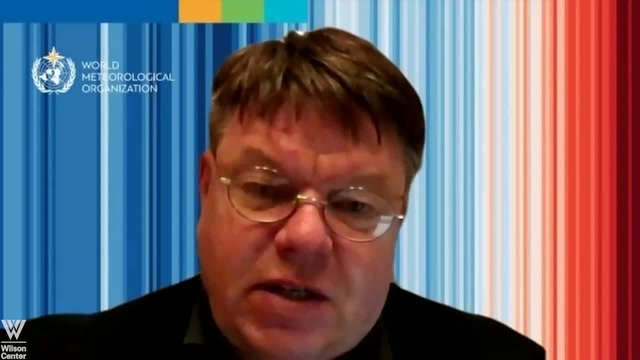 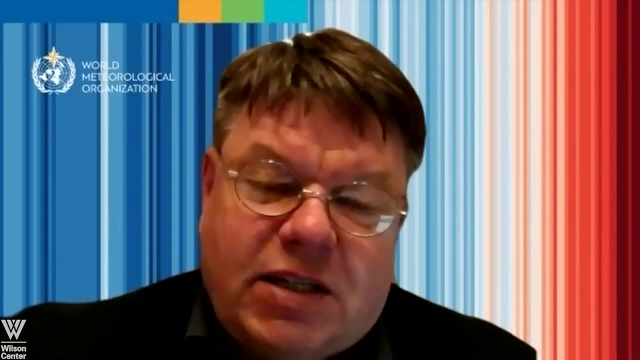 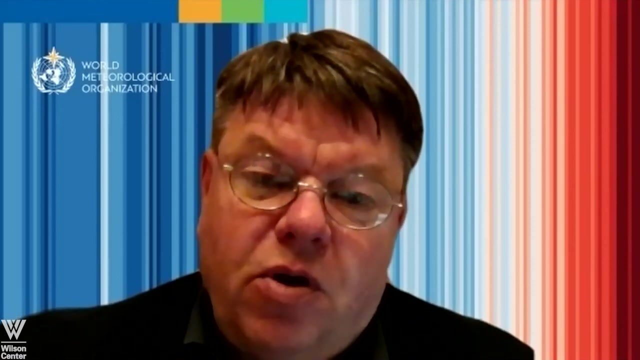 So those are political interesting things and they are some sort of tipping points. So far it hasn't been happening, but of course everybody understands that Arctic has seen the largest changes worldwide and that's going to happen also in the future, So it has certain symbolic value. I would say. And of course the Arctic countries are wealthy countries, and that's one dimension, And of course we have a large part of the fossil fuel resources that we haven't been exploring so far. They are located in the Arctic, especially in the Russian. 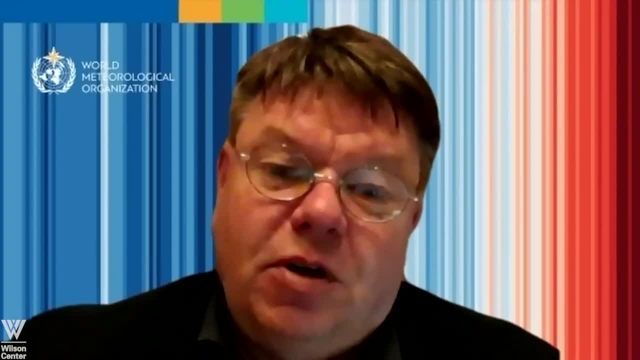 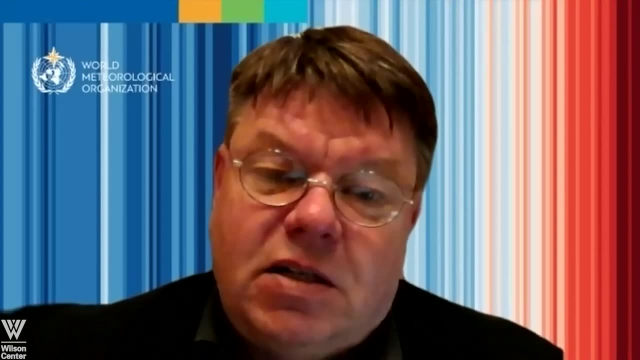 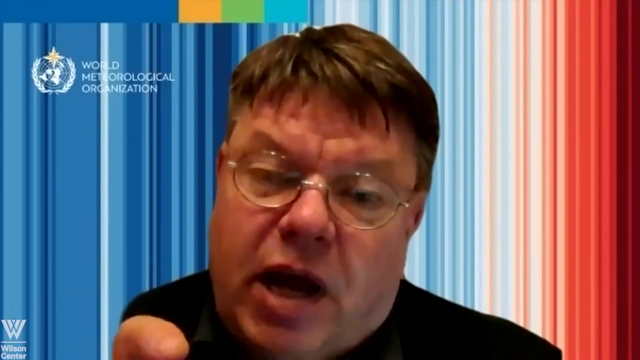 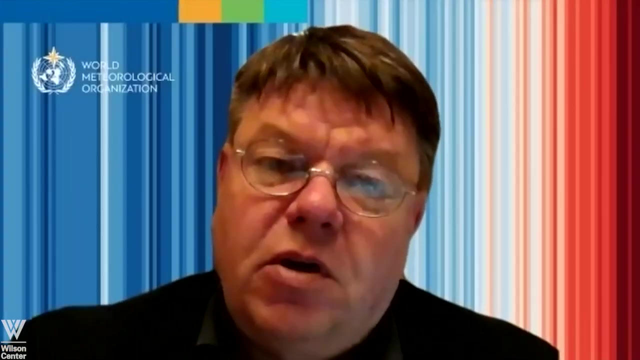 Arctic, and that's a politically sensitive issue- whether we will leave them on the ground, which should happen if it would be successful in climate mitigation. And, of course, we are paying also growing attention to climate adaptation. Many countries and many financing institutions have decided that they will allocate half of their financing for adaptation and, of course, once the 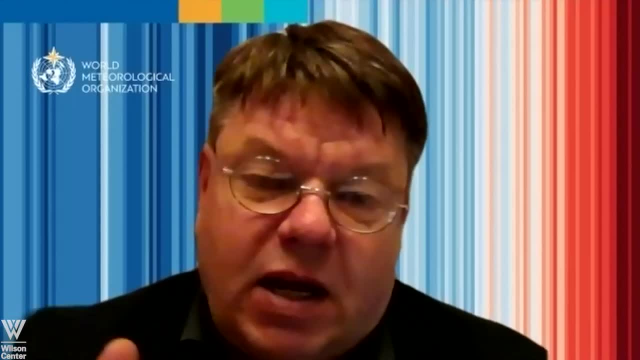 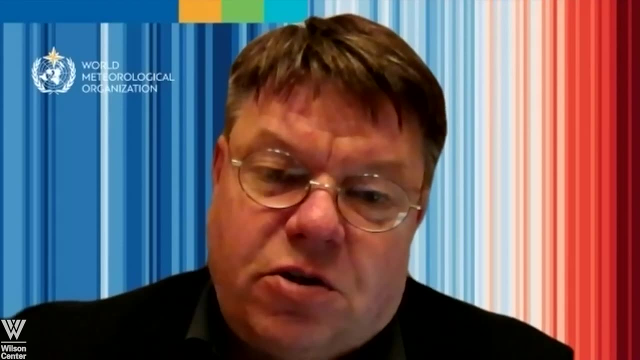 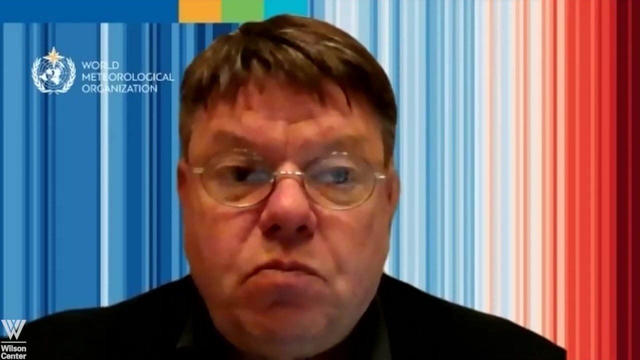 infrastructure is in the Arctic are about to collapse and the sea level rise is having negative impacts on the coastal infrastructure, So that's also one dimension of the things that we are dealing with. Well, I've never lied to a secretary general before, but there's always a. 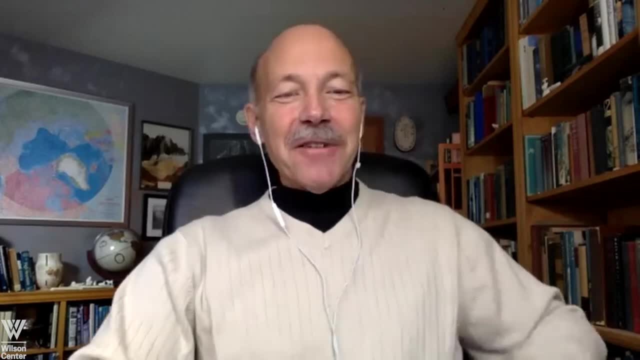 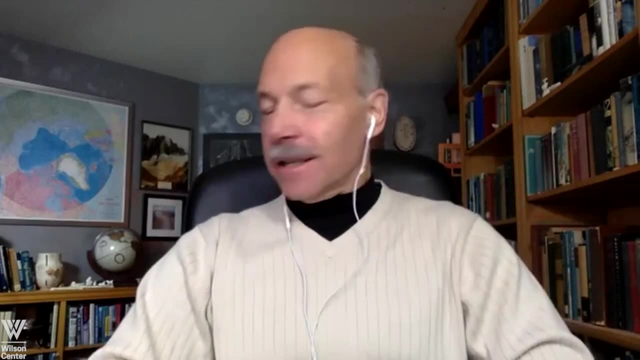 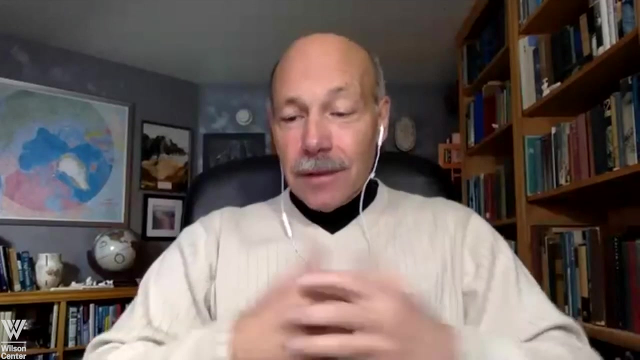 first time. So I want to ask you one more question, if I might. How do you feel going into COP? I mean, it's daunting. It's hard to sort of be uplifted when you see so much that needs to get done. On the other hand, there are some areas where there has been some progress, even if it's 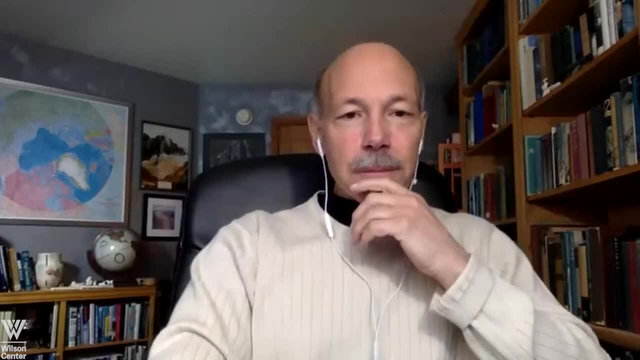 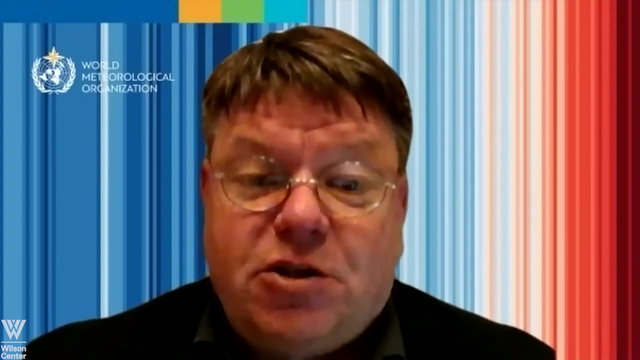 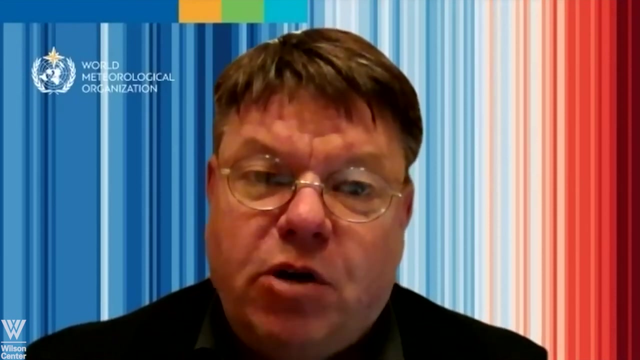 just awareness. So how are you feeling going? So I've been following this climate question since the 80s and it's a big surprise for me personally how much we are talking about climate nowadays And we have growing amount of countries which have, at least at the political level. 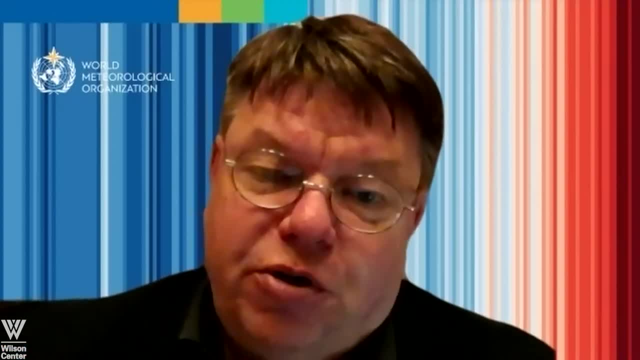 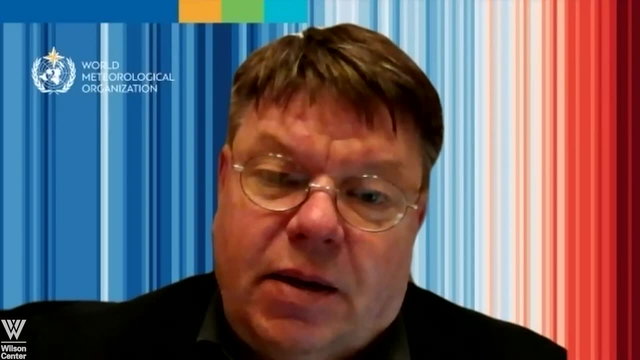 they have promised to aim at becoming carbon neutral by 2050.. That's the case in USA and, of course, European Union countries, and China has said that it's 2060.. And even countries like Russia and Saudi Arabia have said that they have the same target, But the concrete pledges they are still. 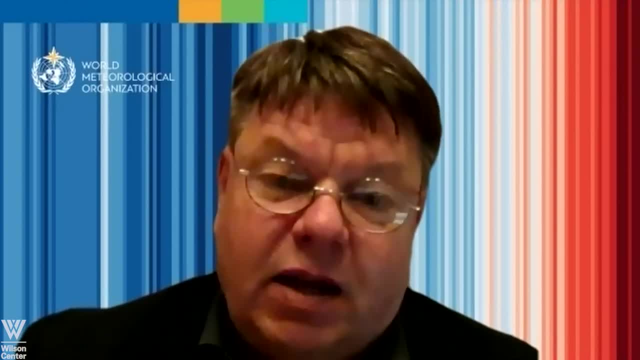 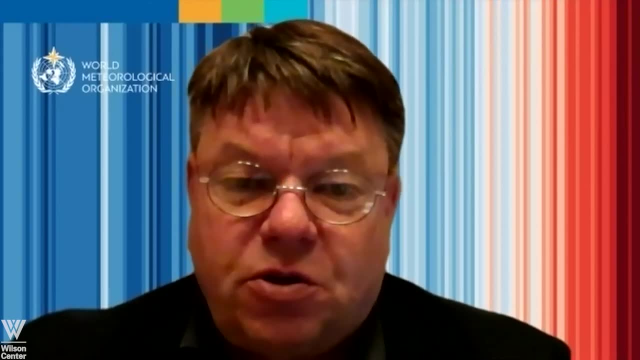 missing. So that's a big challenge in the climate And I think that's a big challenge in the climate. That's a challenge And what's happening also at the private sector. nowadays, if you listen to the car manufacturers or energy sector, the conversion is going on. 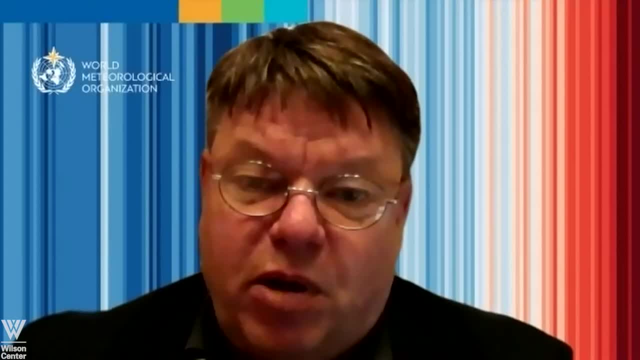 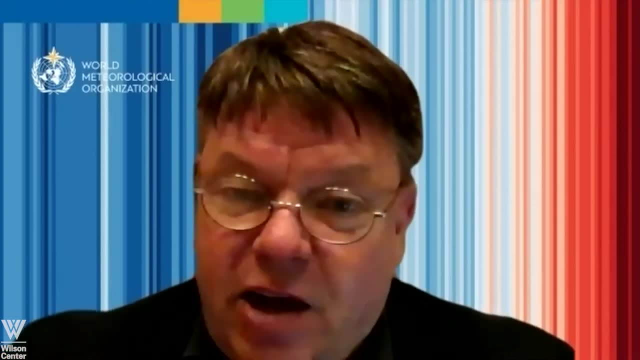 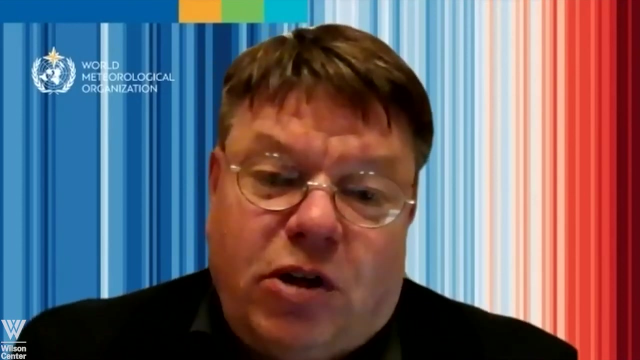 And I'm confident that we will be able to tackle this problem. But it's another question whether we are going to reach the Paris limit. So that's so far. we are not yet there. But two degrees is not out of question fully, Of course, that means more than four degrees in the Arctic. 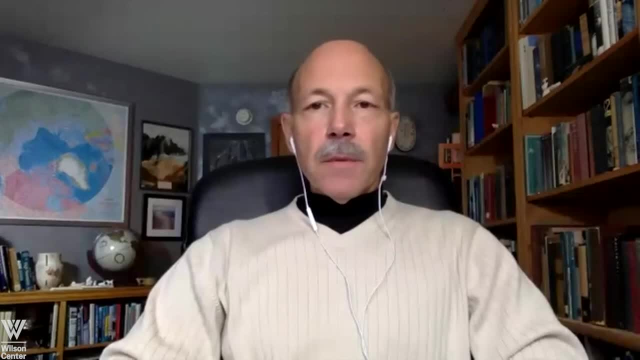 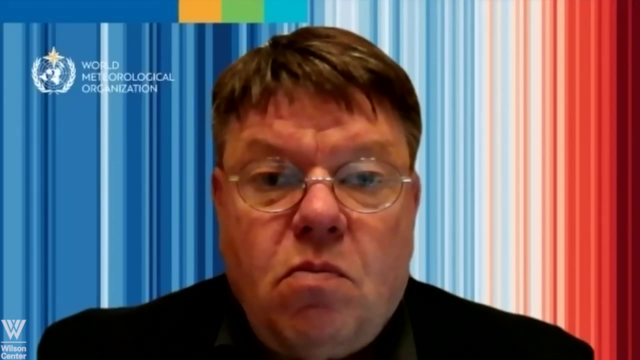 Thank you for that. Before I hand the program over to Heli for her last comments, I'm wondering if anyone else has some closing comments that you'd like to share. And, Mr Ambassador, perhaps I can start with you, and then our friends at MISLA, and then Evan, and then on to Heli. 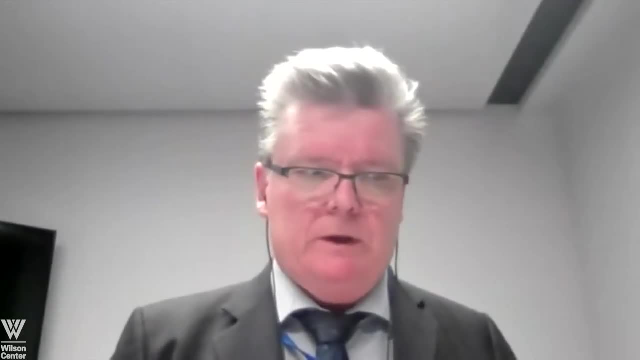 Mr Ambassador. Thanks very much, Mike. Very briefly, I have a sense that Arctic appears to be on everybody's mind that I talk to or hear about. I also have a sense that- and, Mike, you alluded to that already- that the Antarctic shall be on everybody's mind as we move forward. 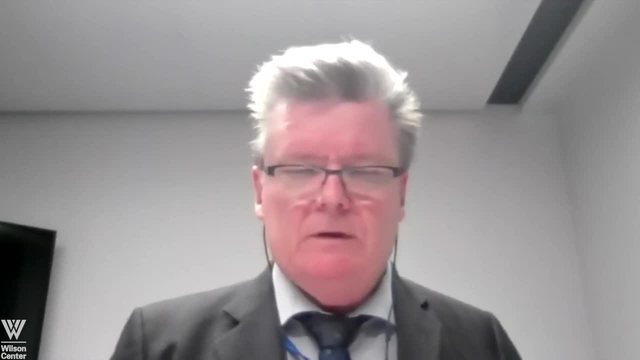 I think the key shall be to understand that, firstly, they're vastly different in terms of law, geography, History, But that there are some common challenges and common issues on climate, biodiversity and others, And our fate, our future, depends on our ability to address the challenges in both of the polar regions. 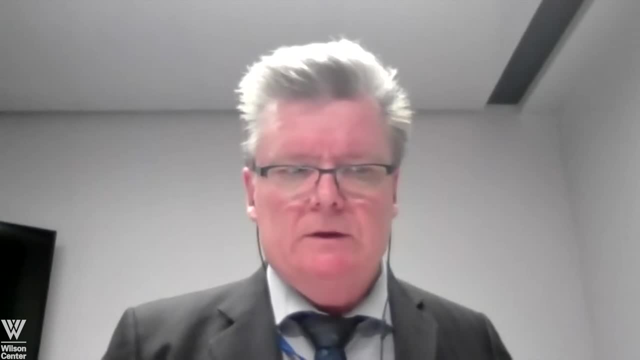 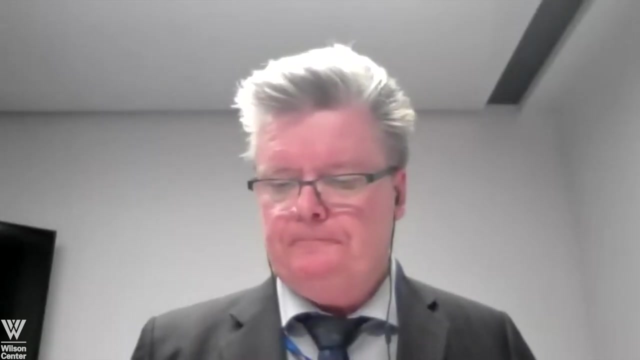 And that calls for increased attention to the Arctic Council in the Arctic and the Antarctic Treaty Mechanism in the Antarctic. It's only through international cooperation uh will be able to succeed. thanks, thank you for those wonderful comments, tj, chris. other comments please? i just wanted to again uh, thank you for letting us participate and again we feel very. 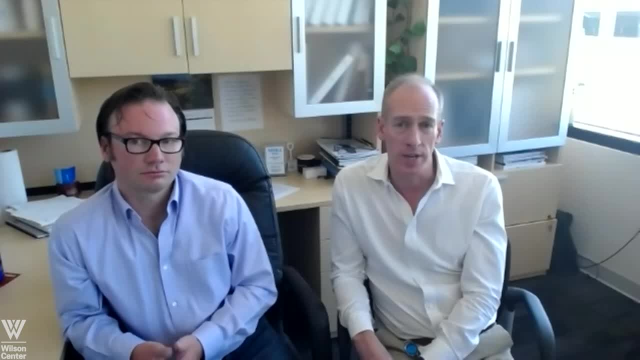 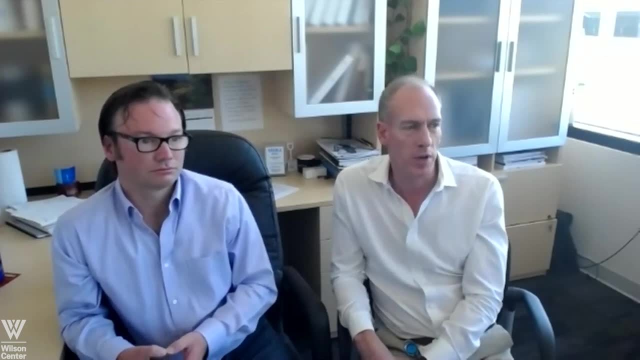 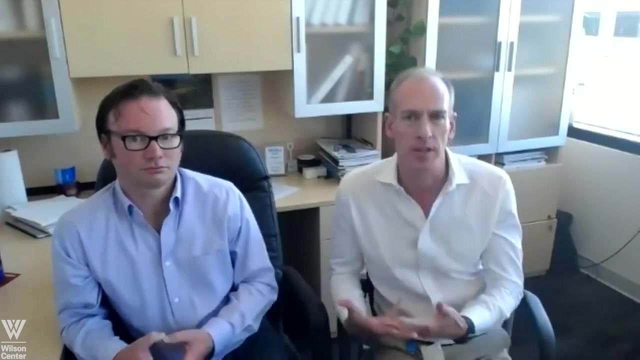 motivated advice law, that the work that we do is more needed than ever, and it's uh, it was uh difficult here in the us, uh, for a brief period of time to be in a country that seemed to be going against science and innovation as a science and innovation based company. uh, but now we're back on. 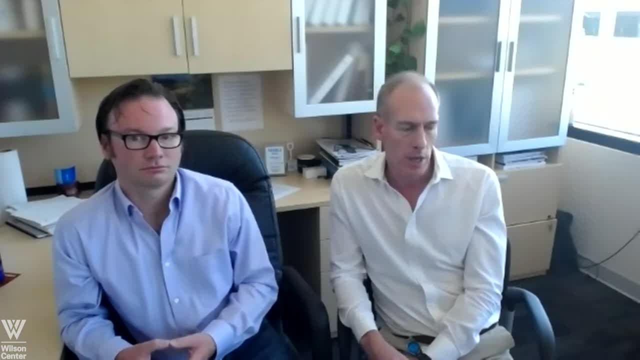 the right side of that and i hope that continues forever and um, we'll just do our best to continue to innovate and and provide the best tools out there uh to be able to provide the measurements needed to combat this problem and hopefully make some uh significant progress, wording off what we. 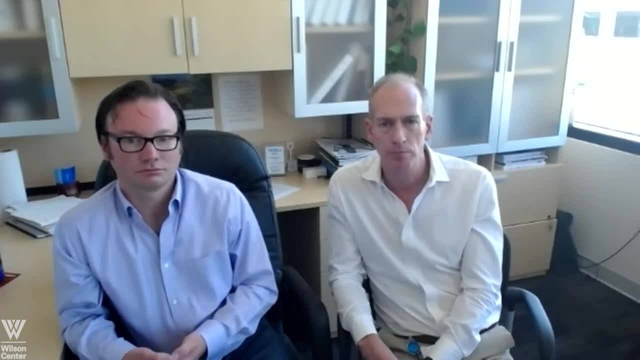 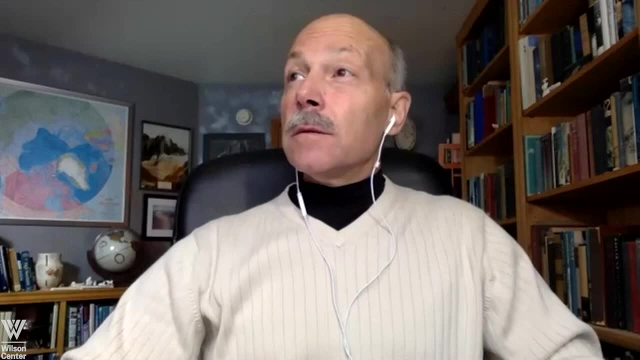 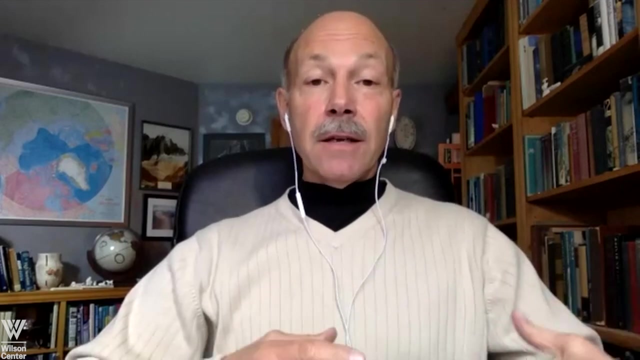 can in the future. well, thank you for that and i'm so pleased that you joined us today. uh, it's, it's more of the uh: provide providing an insight into the tools and the evolution of the tools and the application of the data that you have been able to secure through the deployment. 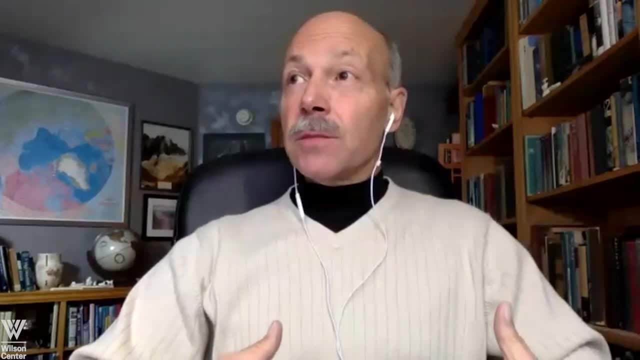 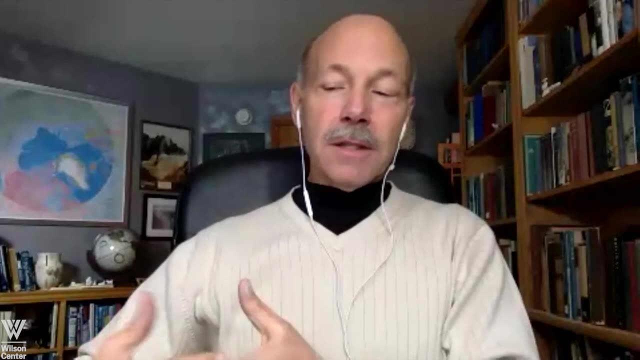 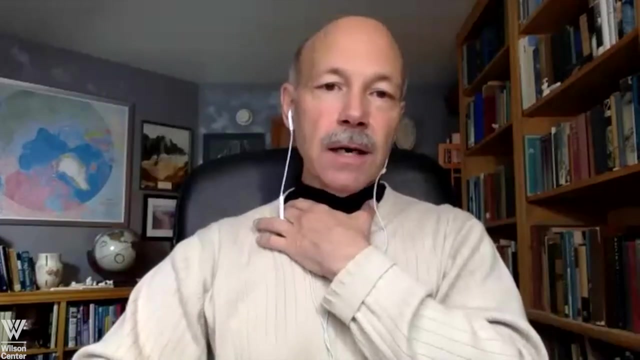 of these tools, uh, that has been not just the most productive in terms of understanding what- what your community is doing for the scientific and research and policy community, but also having this loop effect where these all are connected. we see that there's a lot of work that needs to be done and we certainly can't have sound policy without 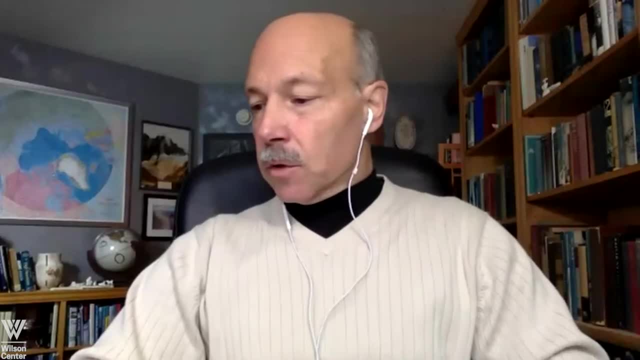 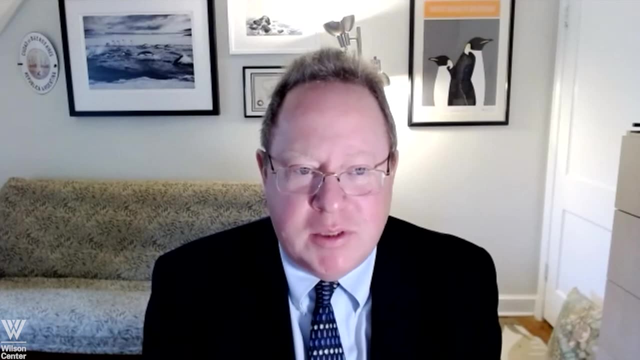 sound data and research and science and policy. so thank you very much, and now over to evan bloom. evan, some final thoughts, please, just very quickly. uh, mike, i'm just so glad that this panel has been able to focus attention on, on polar science, which is not a luxury for the world, it is a necessity. 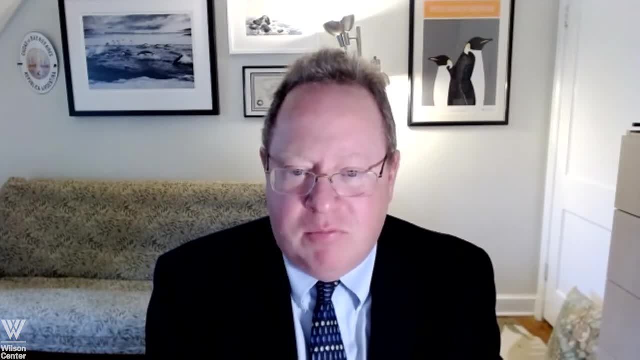 um, in order for us uh to get uh, in particular, climate policy, right, we're not going to be able to get that much more than we do right now. we're not going to have a lot of science in our country. um, we're going to have to uh to uh enter into the few weeks before. 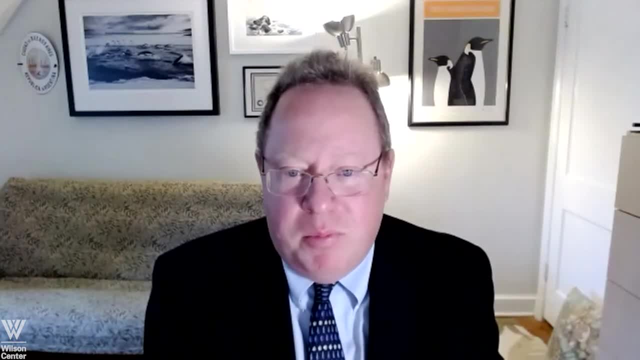 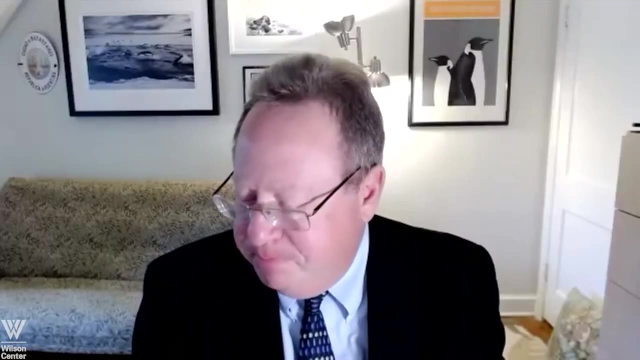 uh, glasgow, this is a critical moment, but even after glasgow we're going to have lots of other key moments. and, uh, there needs to be strong funding for science at both polls, and the political leaders have to listen to what that science tells us. thanks, 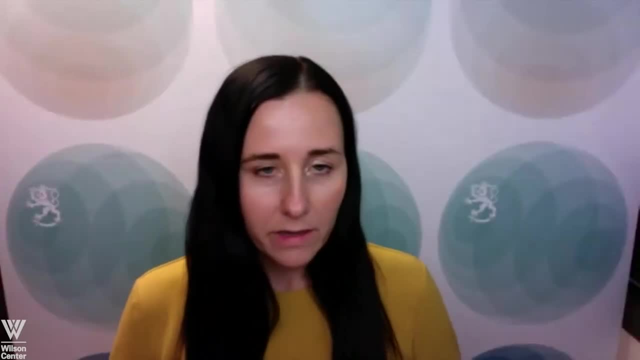 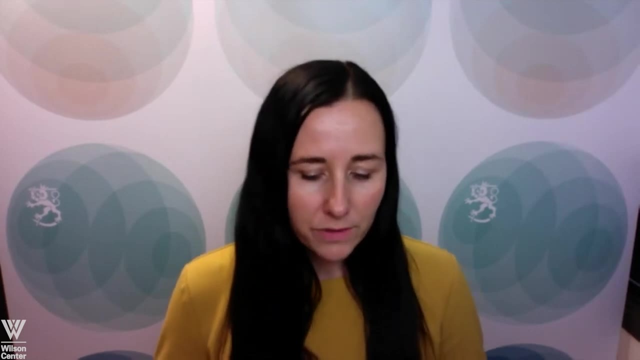 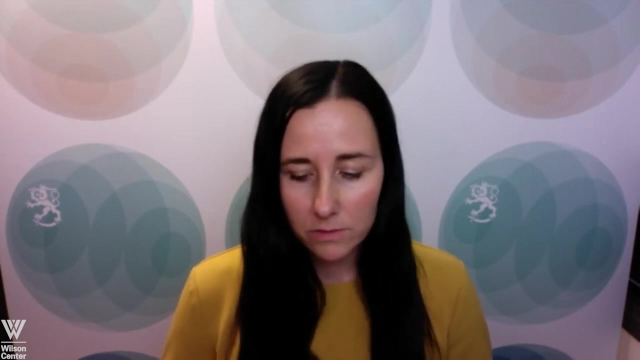 Thank you very much, Mike. Just to say thank you to all of you for such an interesting discussion. Many of you mentioned that we hear more about the Arctic and the Antarctic now, but we talked about the cup, but there is definitely always the need for more awareness raising and the embassy, together with Wilson Center and others, we look forward to providing. 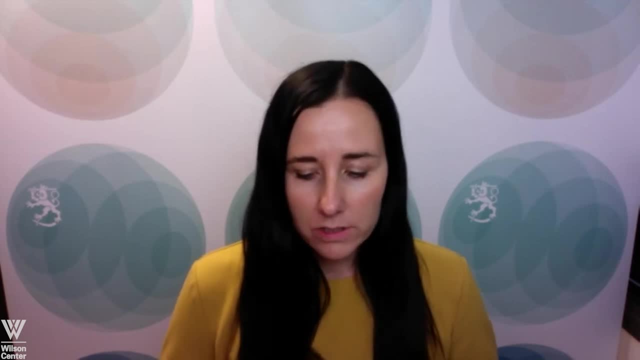 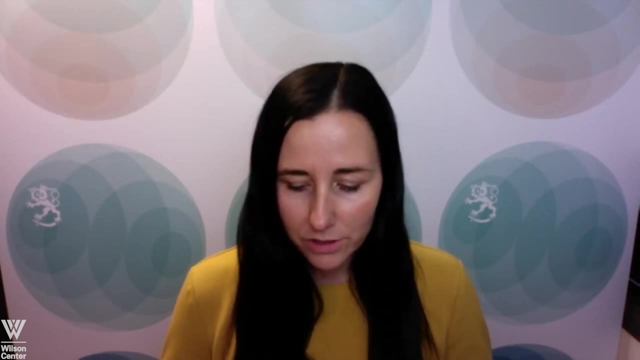 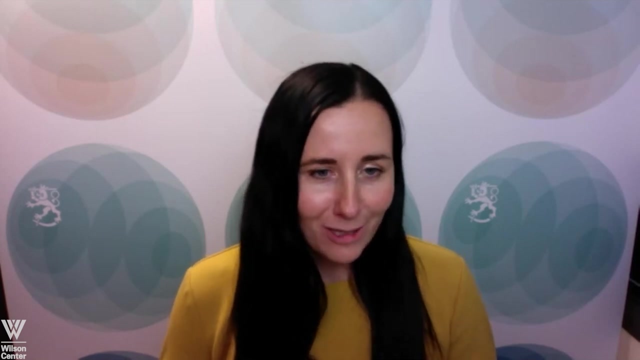 one avenue of highlighting these messages. so just thank you to the Secretary General, Ambassador water, Mackey and vice a lot for joining for this important discussion, And I wanted to also comment on what, Evan, you mentioned many times, and others as well, that it's no coincidence that the portfolio at the embassy, for example, has all three- Arctic, climate change and sustainable economic development- in one package.